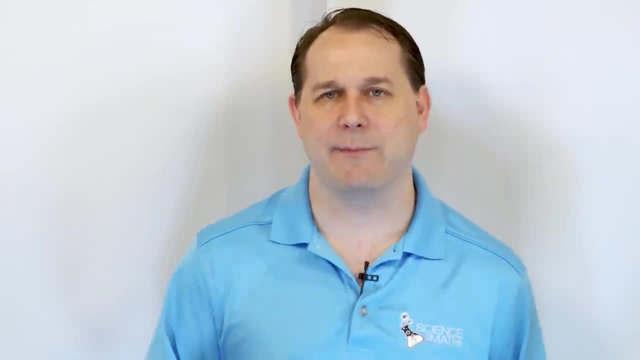 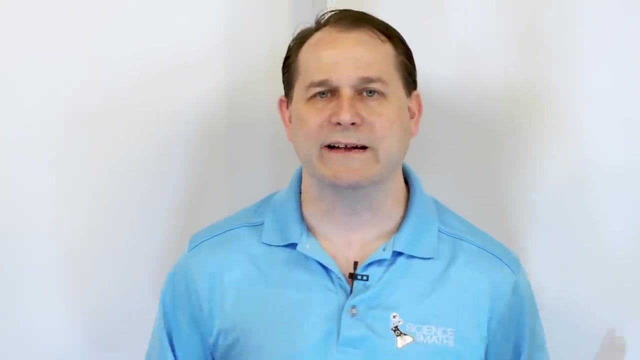 with imaginary numbers. I'm going to show you why we actually care about imaginary numbers. I'm going to short circuit about five more years of math education to tell you why imaginary numbers are so useful and a couple of examples of how imaginary numbers are used in modern-day mathematics, modern-day science and math. So stick with me to the end. 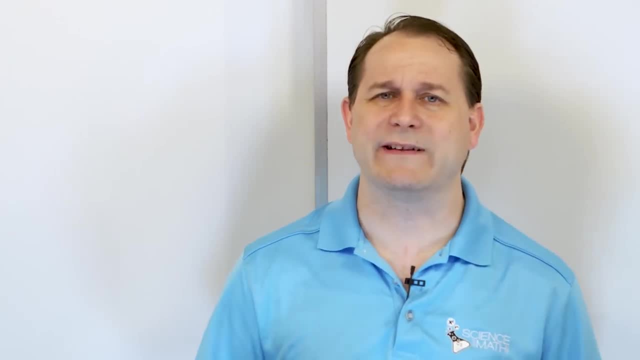 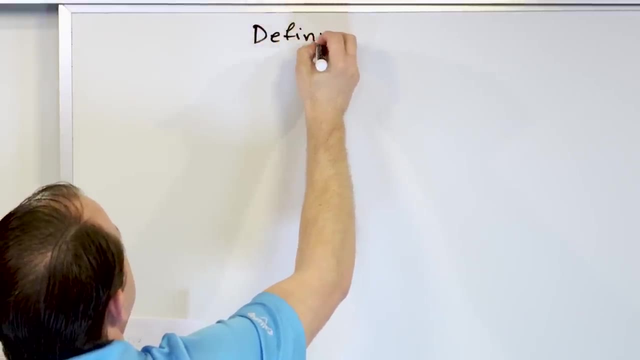 and we're going to get through all of that Now. first I'm going to give you the punchline. I want to tell you what an imaginary number is. All right. so this, right here, I'm going to write on the board. It's called the definition of the imaginary number. 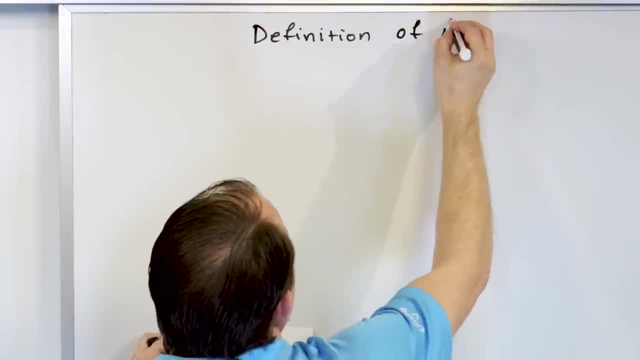 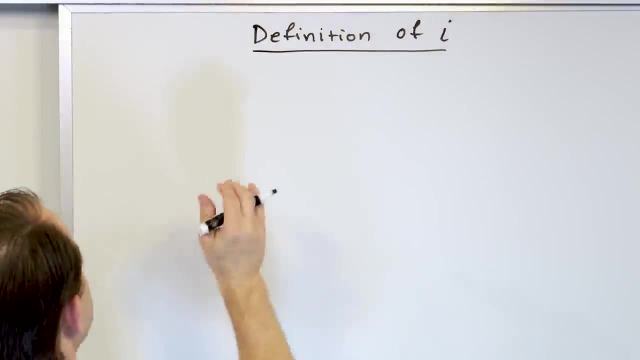 The definition of the imaginary number, which we call i. We use the letter i to mean imaginary number. Anytime you see i in mathematics, it means the imaginary number. So the punchline here is the following thing: The imaginary number i is equal by definition. it's defined. 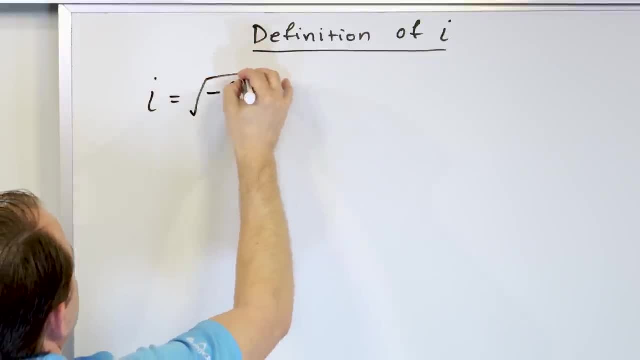 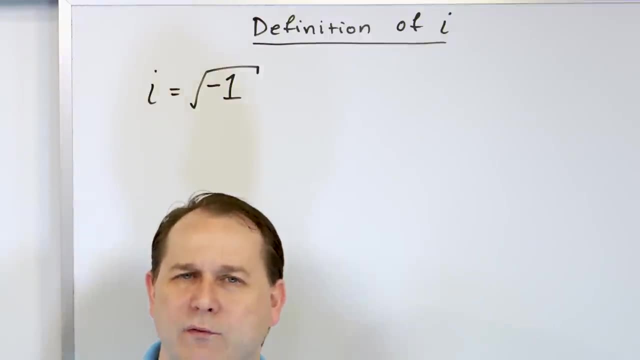 mathematically to be the square root of negative 1.. Now, I've been telling you since the beginning of talking about radicals that we cannot take square roots of negative 1, right. So when you first learn about imaginary numbers, first of all you think they're really, really scary. 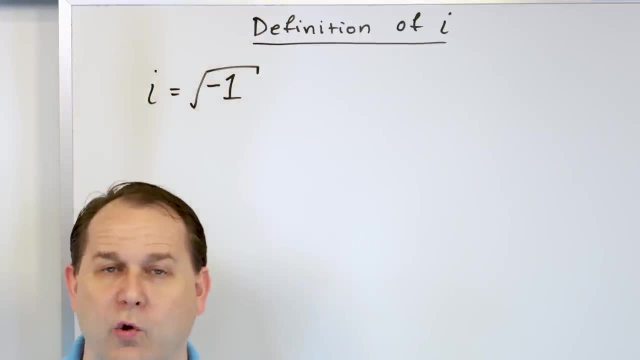 really, really complicated. but I'm telling you they're not complicated at all to work with. Just kind of follow along with me. Secondly, you're kind of scratching your head. How can we do that? How is that legal? We can't take the square root of a negative 1.. Well, the truth is you cannot. 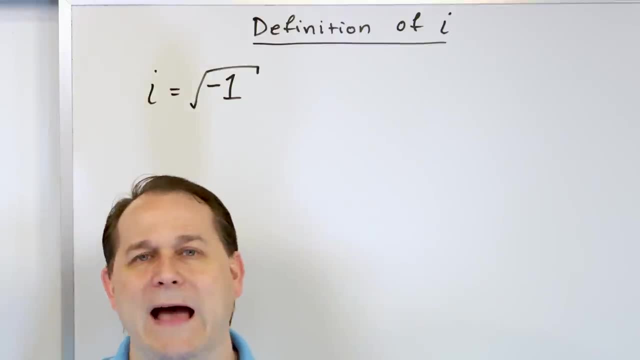 take the square root of a negative 1 and get a real number back. In other words, all of the numbers that you've ever been exposed to your entire life are what we call real numbers. Those are the numbers that we can kind of hold in our hand, for lack of a better word. 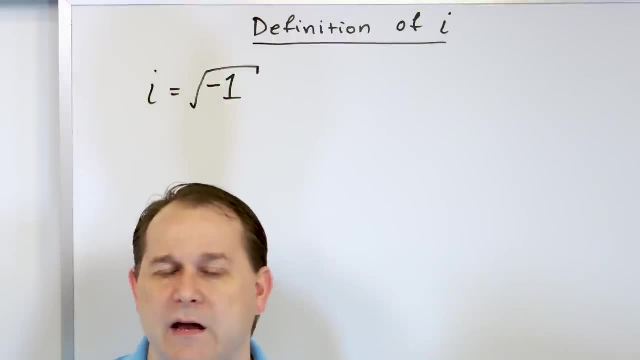 Numbers like 2 and 3, even negative numbers like negative 10, or fractions like three-fourths or one-half, or even non-repeating decimals like pi or like other. you know there's tons of other ones like square root of 2 and square root of 3 and things like that. Those have decimals that. 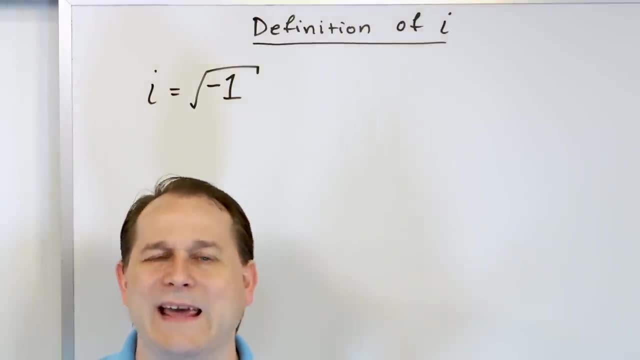 go on and on forever. Those are all called the real numbers. The truth is, you can't take the square root of a negative number and get an answer. that's a real number. So mathematicians over the years have invented a totally new kind of number. It's called an imaginary number. It's a. 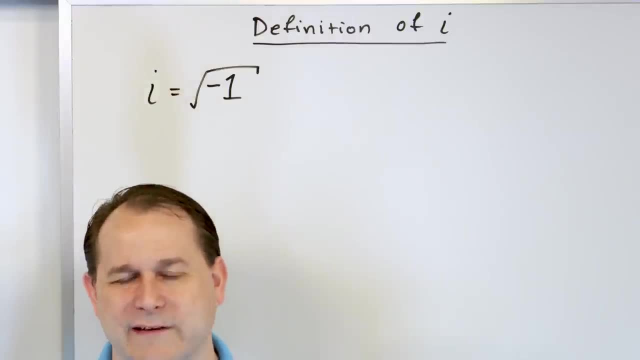 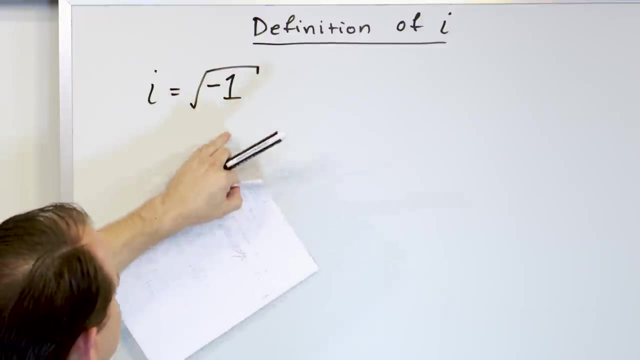 terrible name because it makes it sound like it's a fictitious thing that's useless. The truth is very, very useful, And we define the letter- i we're going to use it as a placeholder- to be the square root of negative 1.. Now, it is true, I cannot find a real number that will multiply by 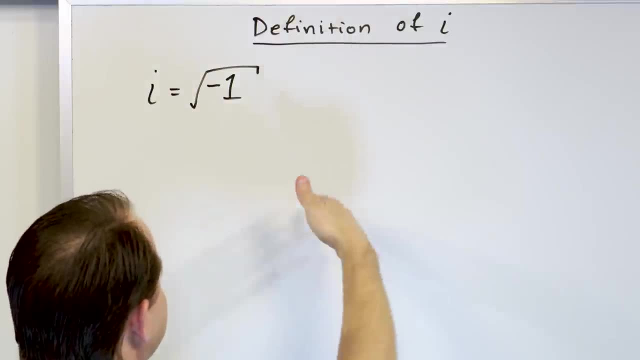 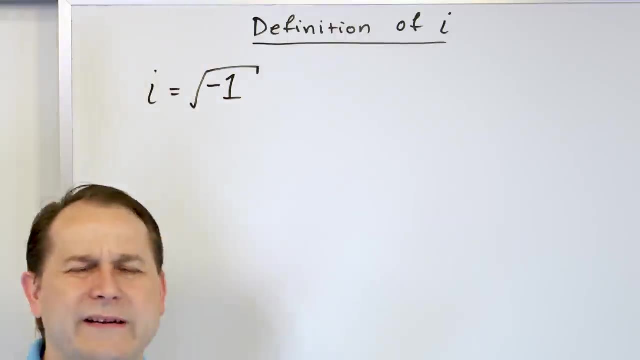 itself. you know, like we say the square root of 9 is 3 because 3 times 3 is 9.. We say the square root of 16 is 4 because 4 times 4 is 16.. We can't say that the square root of negative 1 is some. 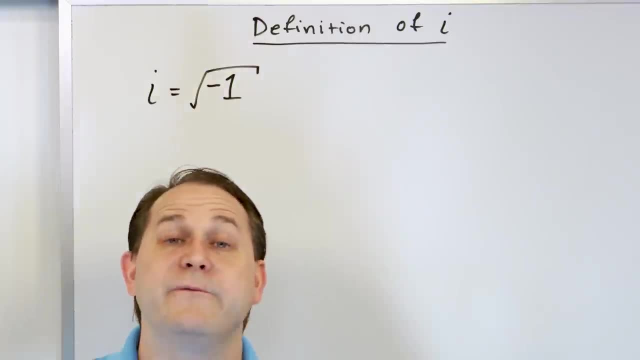 number times some number, because there is no number that does that, We have to invent the square root of a negative number. We're going to have to get used to seeing the letter i running around When we're simplifying expressions. you can kind of think of i as like a variable: You. 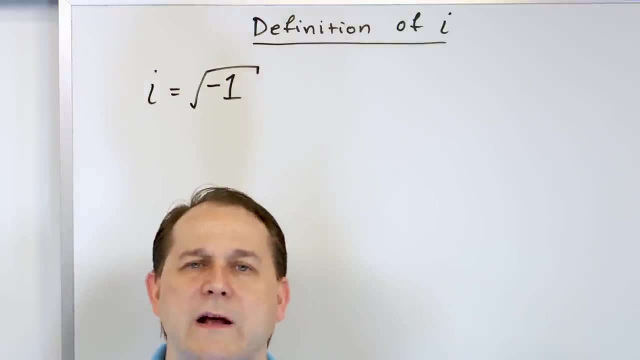 can combine terms like terms, we have to have i involved, and so on. We're going to be squaring and cubing and dividing and multiplying by i. We're going to be doing all the same things. we do with all variables and numbers all the time, But in the back of your mind anytime. you see. 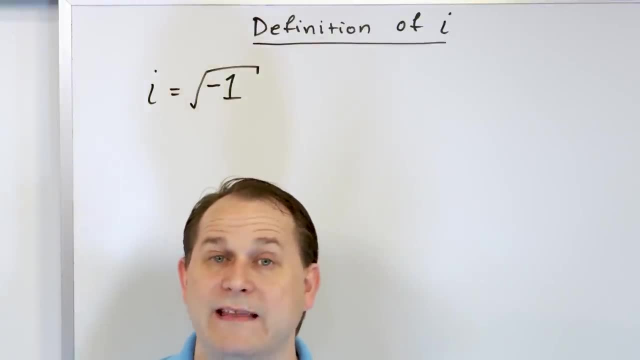 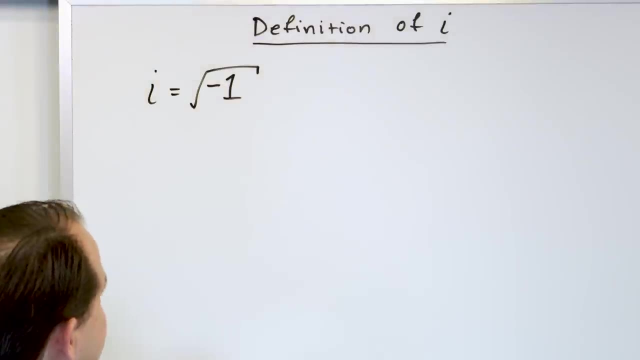 the letter i anywhere on a paper. in math, you need to remember that that is the square root of a negative number or the square root of negative 1.. And it's defined like that, defined like that as a definition. This is not something that you. 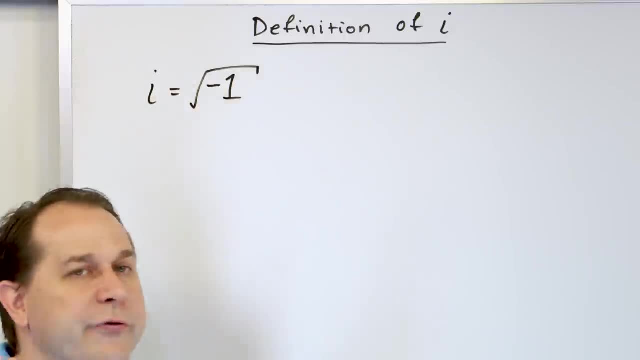 discover under a rock somewhere. It's something that's mathematically defined. The reason is because it's useful. Imaginary numbers we will see are very, very useful. All right, if you define the letter i, this imaginary number, to be the square root of negative 1, it's not a real number. 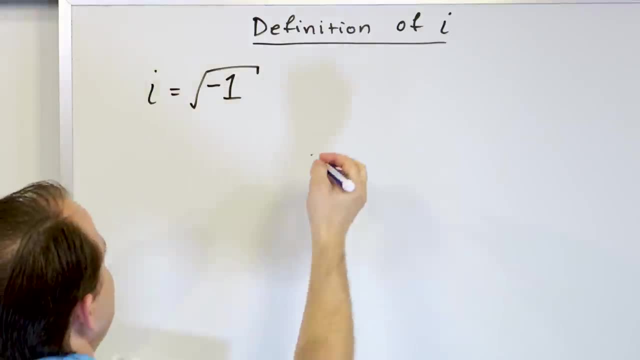 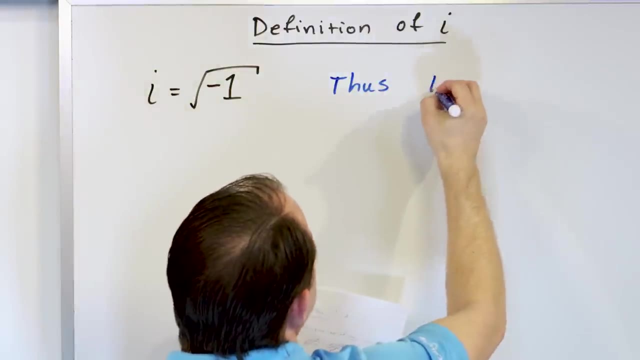 that this is, This is an imaginary number, right? Then, because of that, we can say the following thing: Thus, if you square both sides of this, then we also know that i squared is equal to negative 1. How? Because, if I square this, 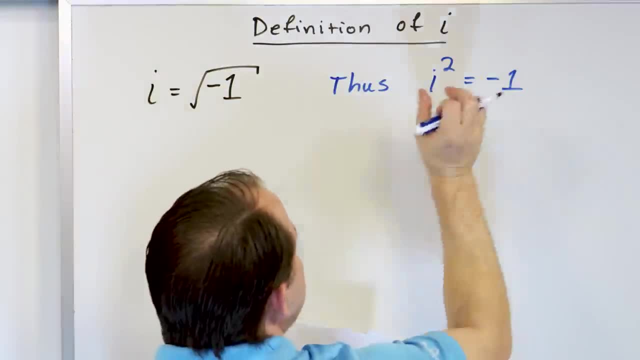 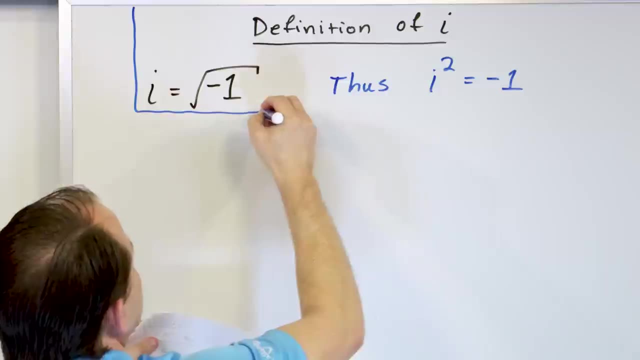 I'll get the i squared. If I square this, they'll cancel with the square roots And then I'll have a negative 1 back. So this is equally important as this. So I'm going to circle this and we're going to reference it throughout the lesson. It's so important. I want you to stop for a second and 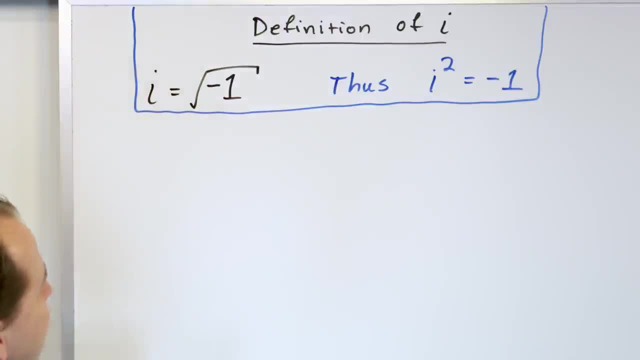 absorb this. It looks and it is very simple, but there's a lot of depth into what's on the board here that we're going to see as we work through the problems. Anytime you have the square root of the i squared, you're going to be able to reference it throughout the lesson, And so 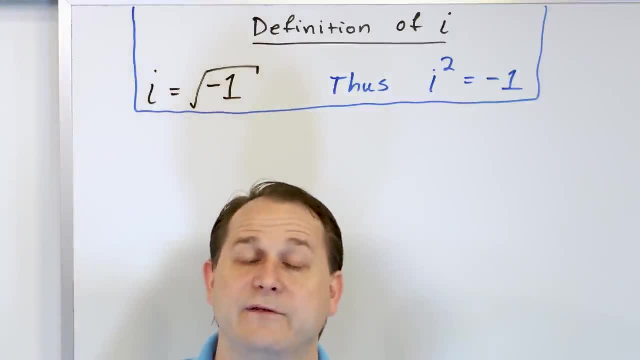 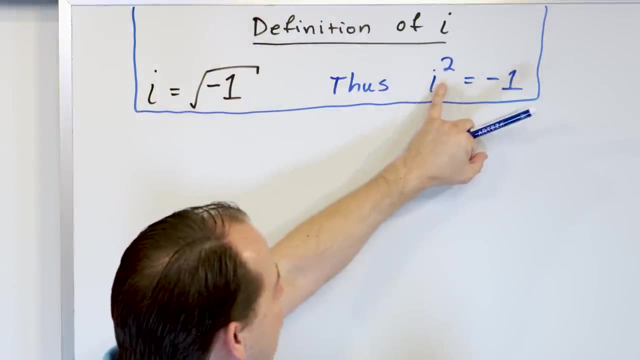 negative one. of course it's i, but the concept of i allows us to take the square root of any negative number we want. but we're going to get i somewhere in the answer and because of that, anytime you square i, you get back a real number which happens to be negative one. it turns out this: 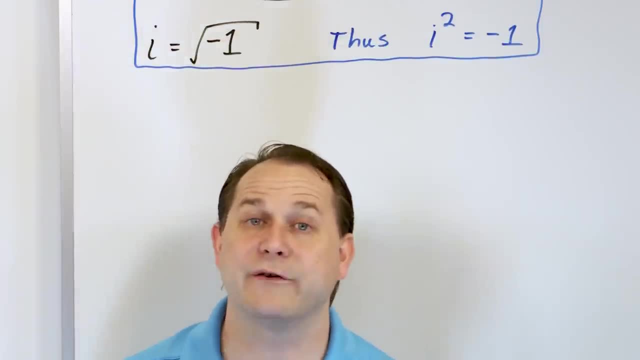 this property. right here is the secret sauce as to why they're so useful, and i'll give you a little bit of a preview. imaginary numbers are not something you can hold in your hand, right? but if i have an imaginary number in this hand, and i have an imaginary number in this hand, 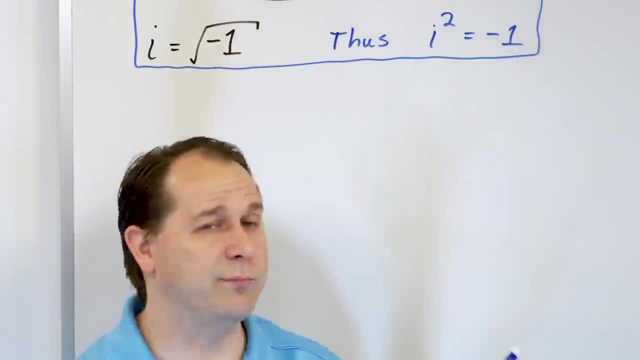 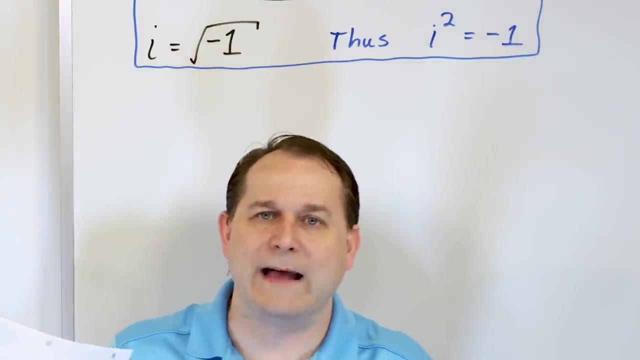 oftentimes, if i combine them together- in this case what's written on the board- is by multiplying them, i have an imaginary thing, times an imaginary thing, which are not things i can hold because they're imaginary numbers. but when i multiply them together, i don't have an imaginary number anymore. 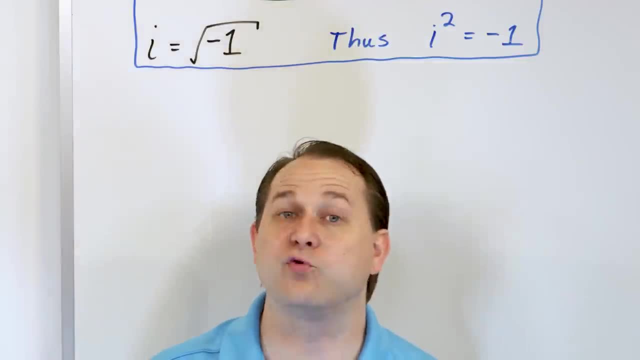 i have a real number back. this negative one is just a negative one. it's a real number, and that is what- probably one of the biggest punchlines as to why imaginary numbers are useful- because i can work with imaginary numbers over here, and i can work with imaginary numbers over here neither. 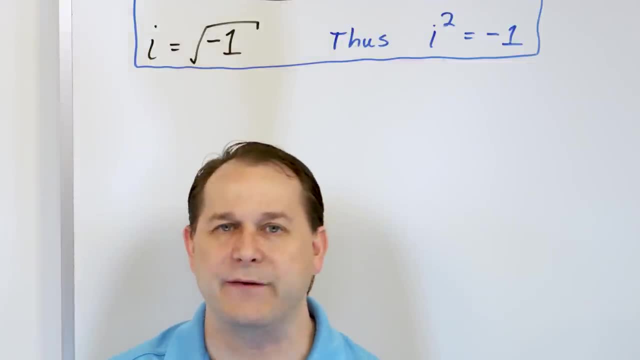 one of the position of the actual numbers on the original numbers matches ever the imaginary numbers, and this is interesting because on the original numbers it's easier to make me work on imaginary- of which represent real numbers, but I can combine them together and often my equations will combine them together. so, poof, they're not imaginary anymore. 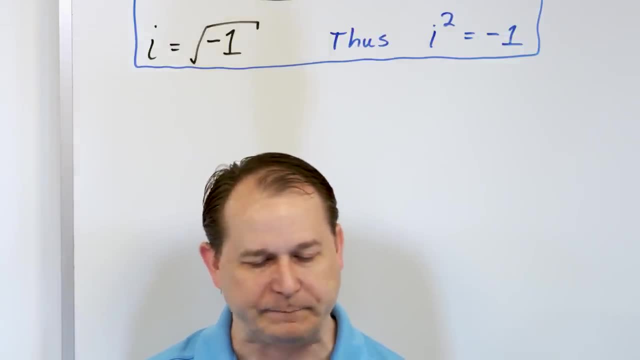 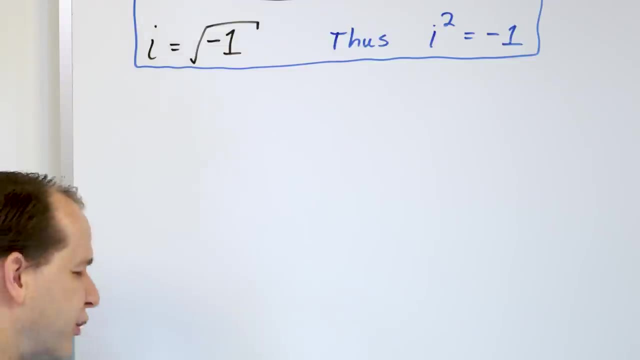 they're real, so that's actually one of the reasons why they're so useful. so this is the punchline and I want to leave it on the board and I want to motivate why we actually need imaginary numbers. it turns out that all of the equations we've learned how to solve all up until now in algebra have required 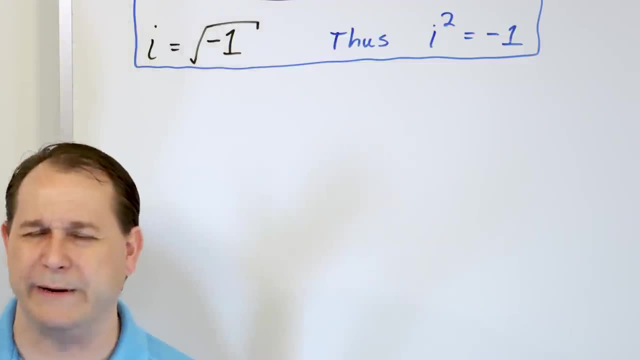 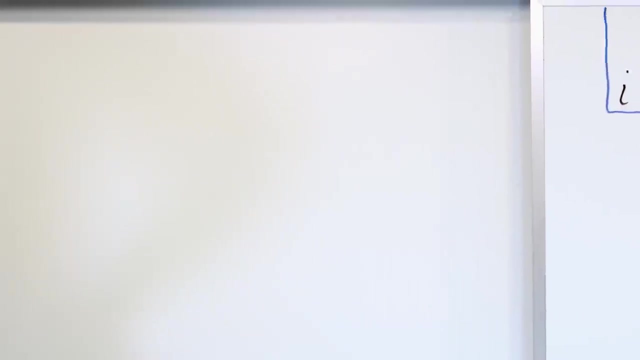 different kind of numbers. now it's a little bit of history of mathematics here, a little bit. okay. some equations require positive numbers to solve. some equations require negative numbers to solve. some equations require fractions to solve. some equations require imaginary numbers to solve, which is what we're gonna get to. I want to go down that with you because I think it's very. 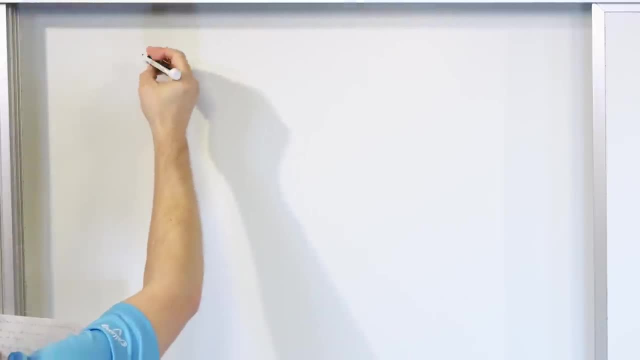 important that you understand where this comes from. so I'm gonna talk about real numbers for a second. because real numbers- let me see if I can write real numbers down. real numbers are the numbers that you've been exposed to your whole life, all the way from you know first grade, all the way up. 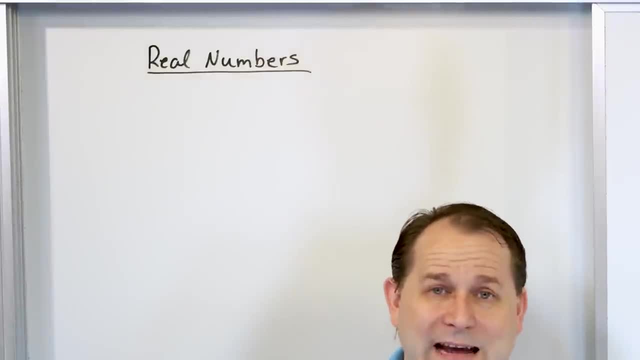 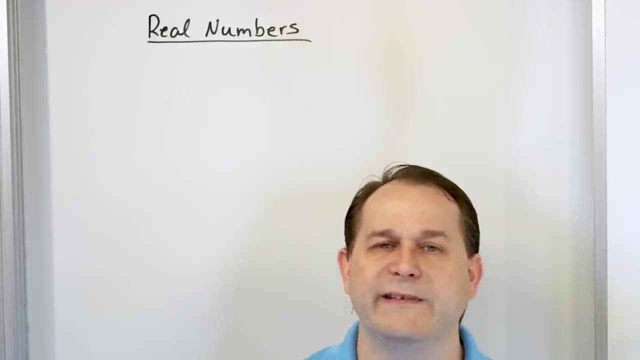 until now real numbers. every number you've ever seen, even if it was negative, it's still a real number. even if it's a decimal is still a still a real number. they're all real numbers, right? so all the equations that you've ever learned how to solve only required real numbers, numbers to solve them. but 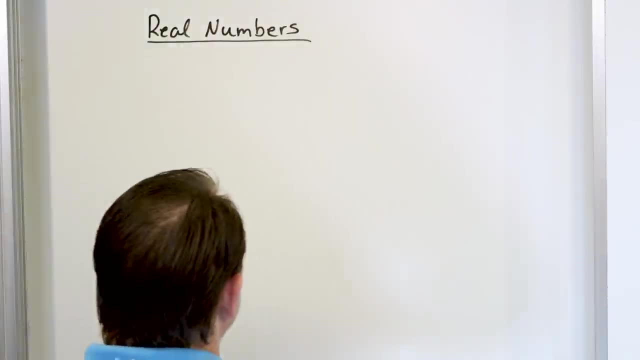 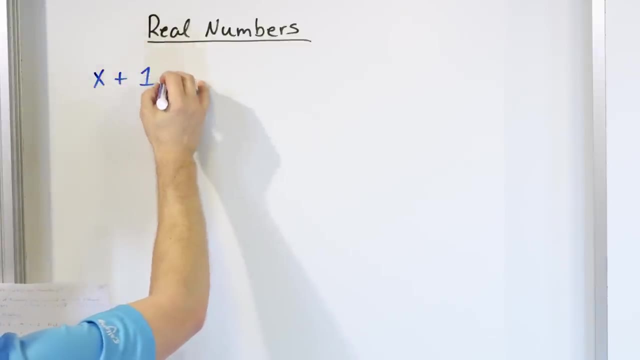 there are different types of real numbers, so let's talk about a few of those right? let's take a couple of equations, right? let's take a very simple equation. let's say we have the equation X plus the number one is equal to three. you all know how to solve that equation: you just move the one over by. 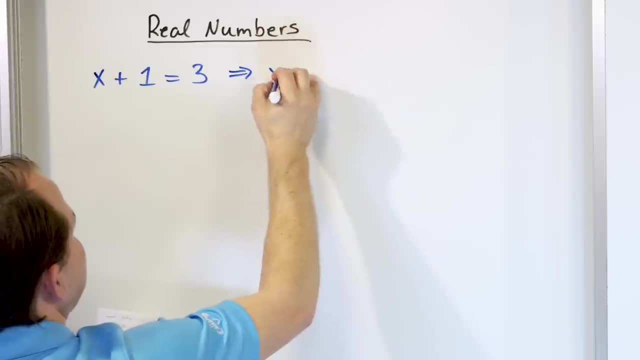 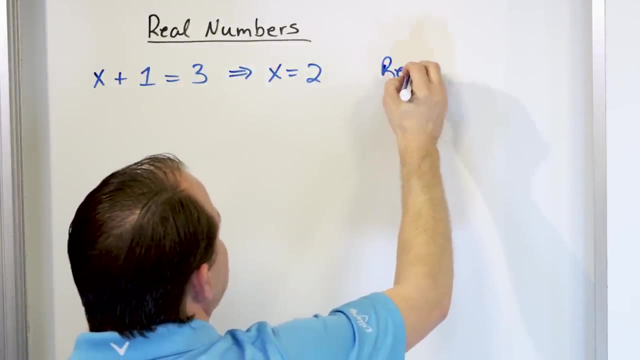 subtraction three minus one is two. so what we found here is that X is equal to two. now, what kind of number is two? well, it's a real number. of course it's a real number. what kind of number is it? it's a real number. I'll put that down. but it's a positive. 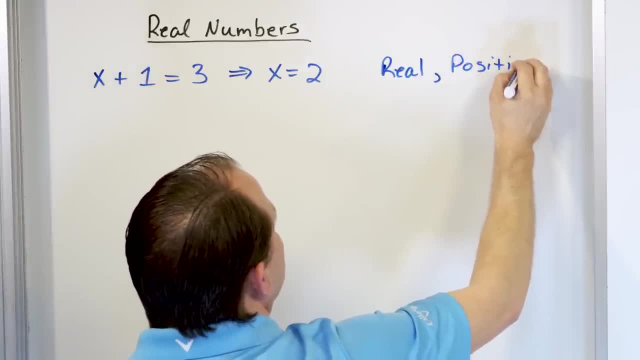 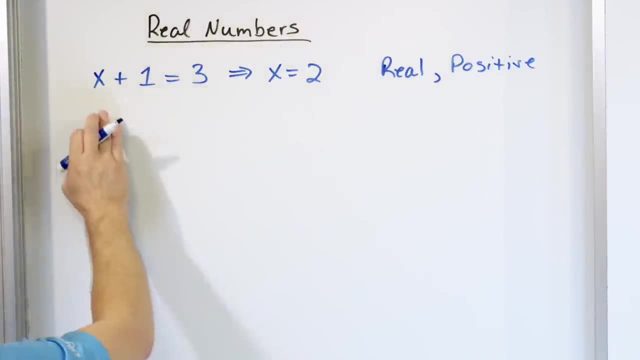 number. so that's a type of number that was invented a long time ago to solve certain kinds of equations, equations that look like this: something plus one is equal to a number, where a positive number is the value of the variable. so we needed a, a positive real number to solve that. 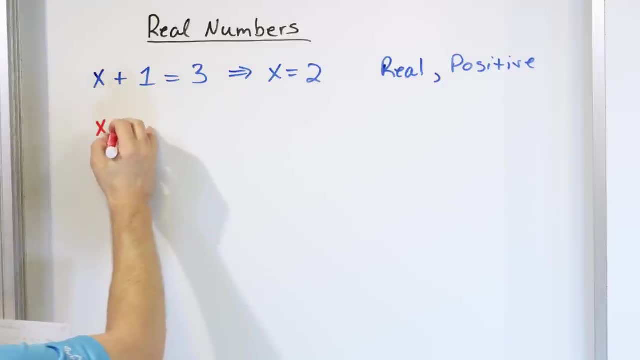 type of equation. let's pick another kind of equation. let's say we have X plus the number two is equal to one. well, this looks the same, but if we solve it it's slightly different. if we subtract two, then we'll find out that X is not equal. 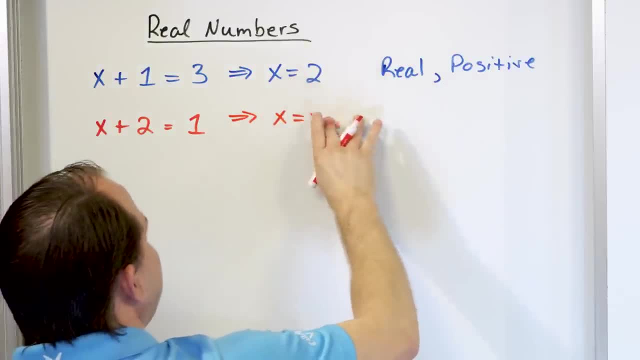 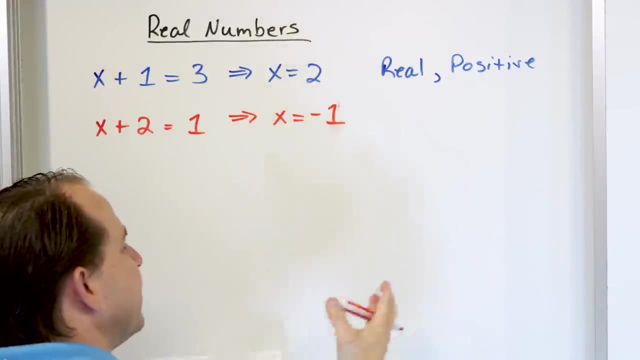 to a positive number. X is equal to, not negative, two. of course, X is equal to negative one, right, because negative one plus two, of course, will give me the one. now, this is also a real number. negative numbers are real as well. however, this one's slightly different. it's a negative number. 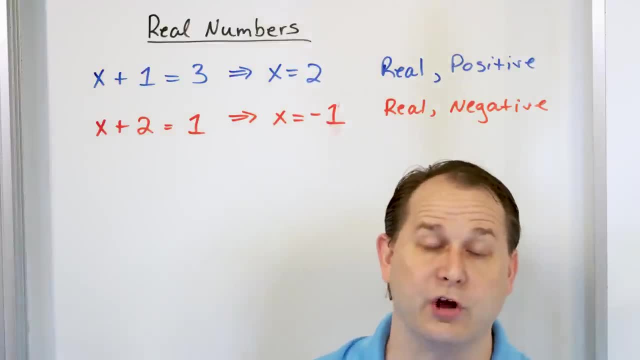 now I need you to think back to maybe a thousand years ago or two thousand years ago, when algebra and mathematics were really first started to be the start to be solidified right. the idea of a positive number is easy to understand: I have five eggs in my hand. easy to understand: I have sixteen buckets of. 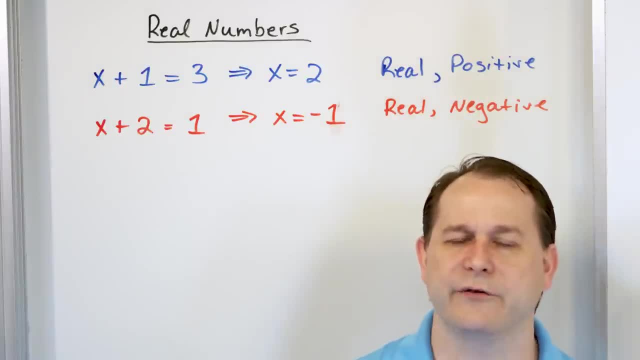 rocks or whatever. I have sixteen pencils. that's easy to understand. positive numbers are easy, but at some point in history somebody must have thought: hey, the idea of a negative number is useful too. it sounds crazy to you because you're so used to dealing with negative numbers, but there was a time when nobody knew. 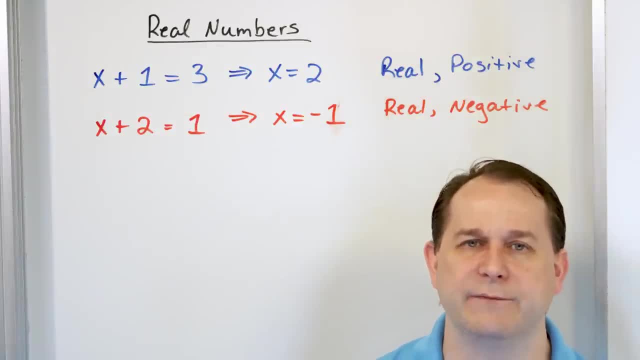 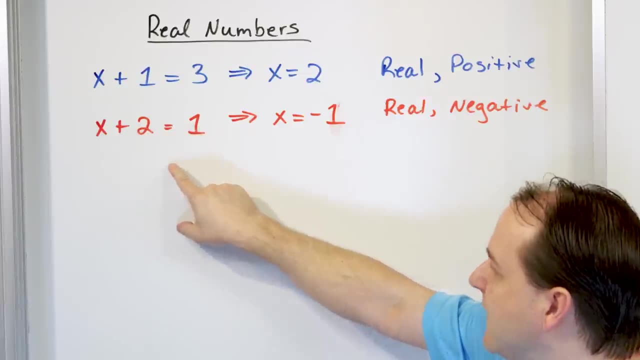 what a negative number was. somebody had to invent the idea of a negative number. why, in order to solve an equation like this- when I subtract something bigger from something smaller, then I can't use a positive number- I have to introduce the idea of kind of owing somebody. I always say negative numbers is like if I 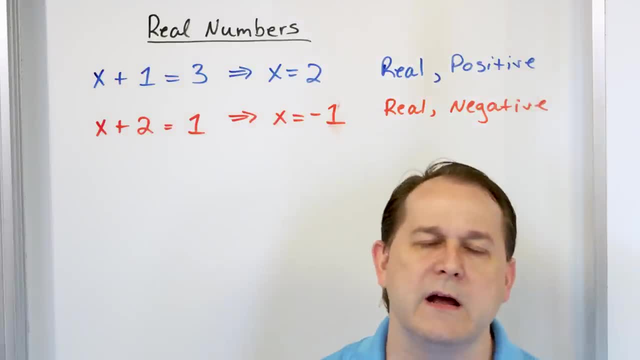 owe you something. so if I get an answer of X is equal to negative one, it doesn't mean I have one dollar in my bank. it means I am bookkeeping keeping that I actually owe you negative. I owe you a dollar, so I don't have that dollar. I actually owe it to. 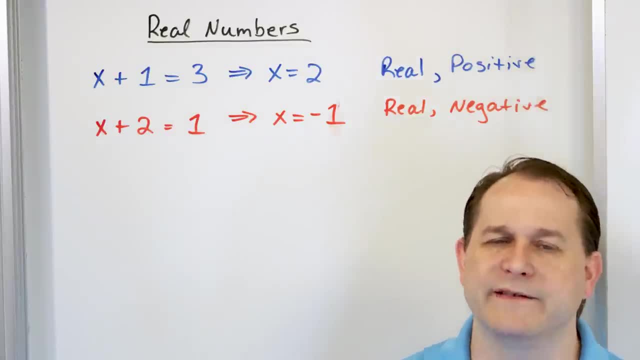 somebody else. that's the idea of what a negative number is, but that number was not something that we're born understanding. you have to be taught that, and we, and it's a useful idea to solve an equation like this, which is a different kind of equation. right, it requires negative numbers as an answer. 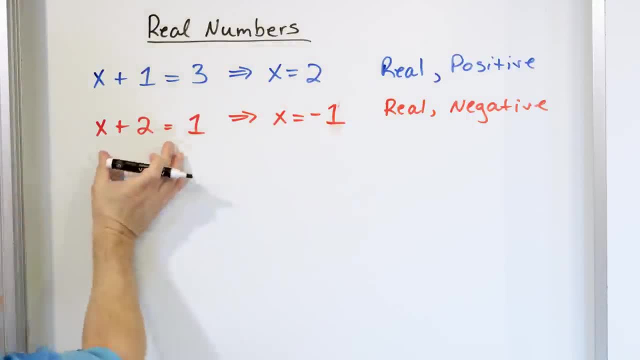 or as a, as we need to invent this in order to solve this kind of equation. so let's continue on. let's take another kind of equation a little bit down the way in history, somebody's tried to solve an equation like this: x plus 1, 4th is equal to 1 half. you all know how to solve this, no problem, I'll. 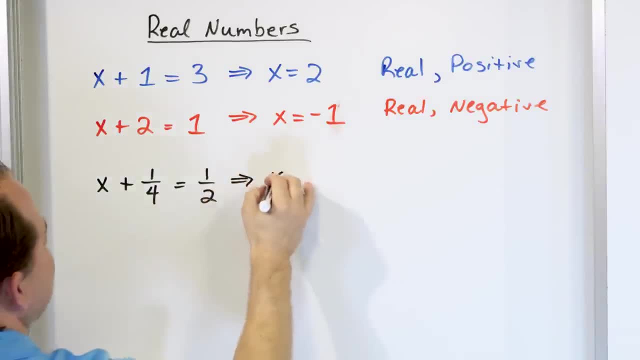 just subtract the 1 4th from both sides. what am I going to get? I'm going to say that x is equal to well if I take 1 half minus 1 4th. of course you can do the common denominator, but you all know 1 half minus 1 4th is equal to 1 4th, right? 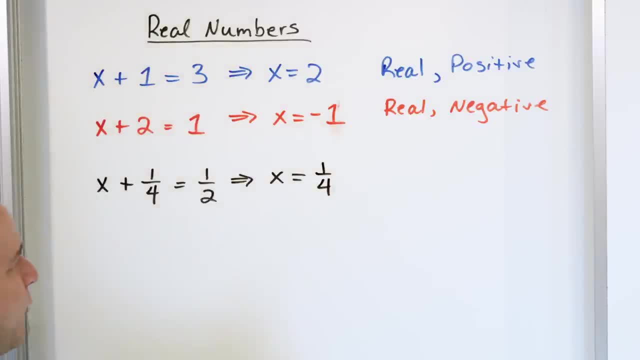 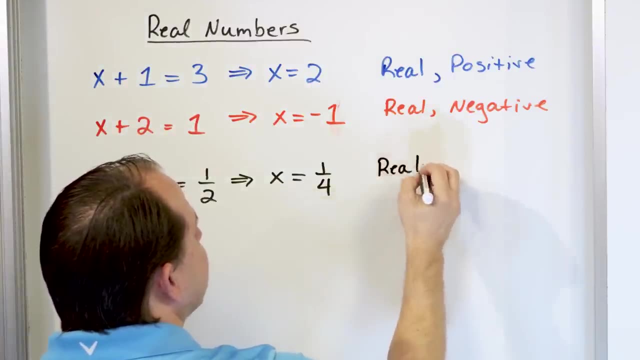 again, this is a real number. I can have 1 4th of a sandwich. I can have 1 4th of a of a candy bar. of course it's a real number and it's a positive number also. well, I'm not writing down every little attribute of all these numbers. it's a. 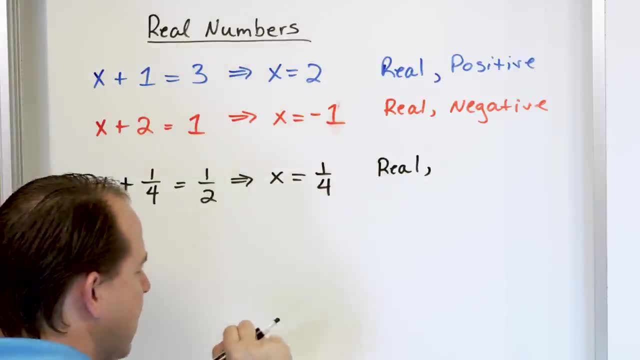 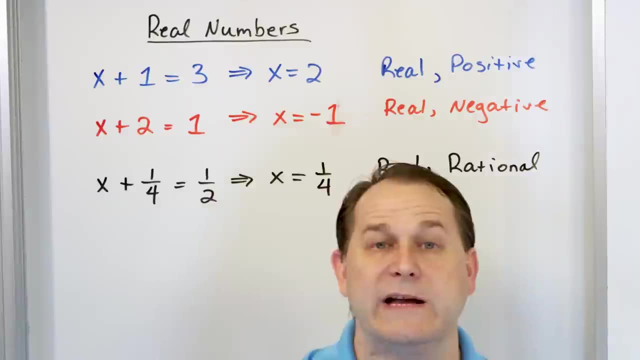 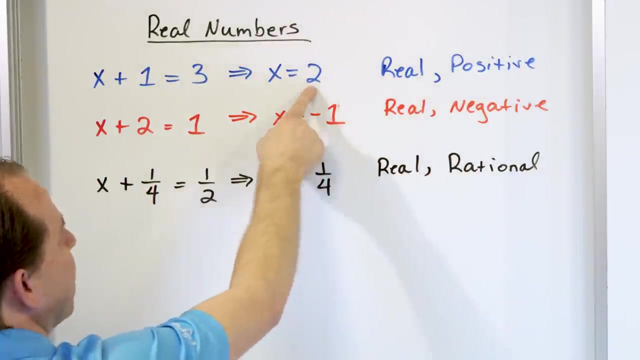 positive number, just like this 2 is. however, it's different than the others because we call this rational. a rational number, remember, is a frat, is a number that can be written as a fraction, any fraction. so 1, 4th, of course, is a rational number, but I didn't write it down for these two. these two are also. 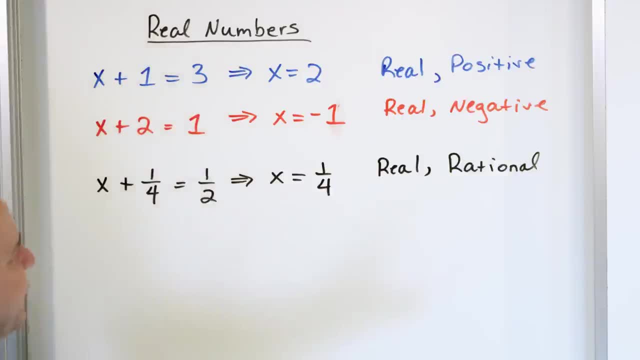 rational numbers, because 2 can be written as 2 over 1. that's a fraction. negative 1 can be written as negative 1 over 1, so that's a fraction. so let's take a little bit of an aside to talk about these rational. of these rational, they give you some examples. 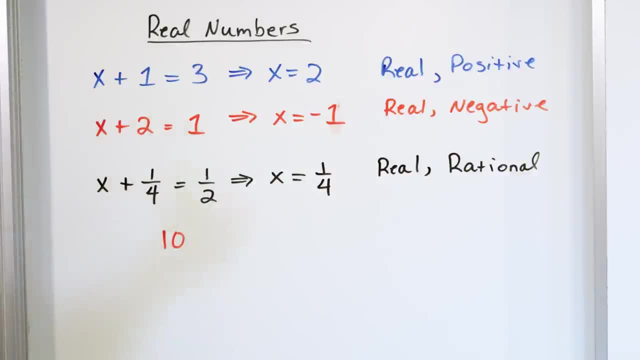 some more rational numbers. the number 10 is a rational number because I can write it as 10 over 1. the number 3, 7th, is a rational number because it's a fraction of course. the number negative 2, 3rds, that's a rational number because that. 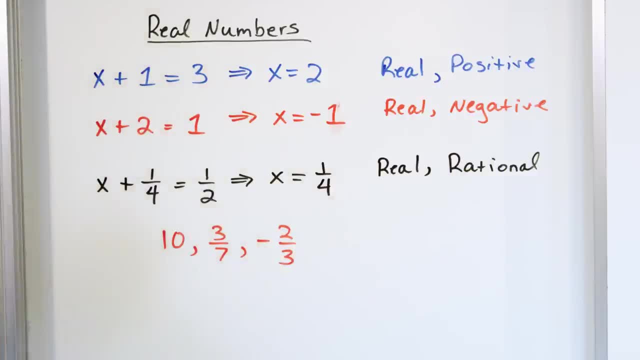 obviously is a fraction that happens to be negative as well. that's fine, it's still rational. let's take something crazy: 1, 0, 2, 8, 1028 divided by 37, that's a fraction, because it's a crazy numerator and a crazy denominator. let's 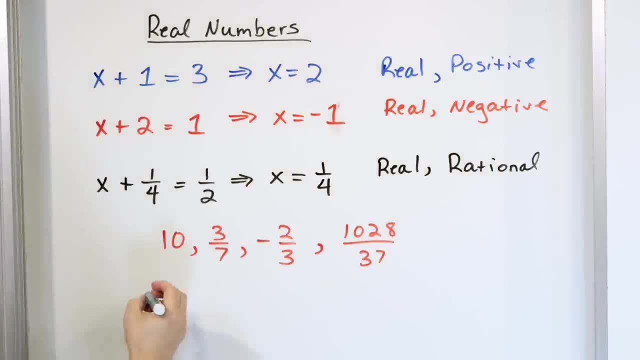 keep on going, because we can make a little bit of a difference between the number to the number 3 and the number 4. so we're gonna make up a few more and there's a point to this, I promise. let's take a look at 0.75. you might say well. 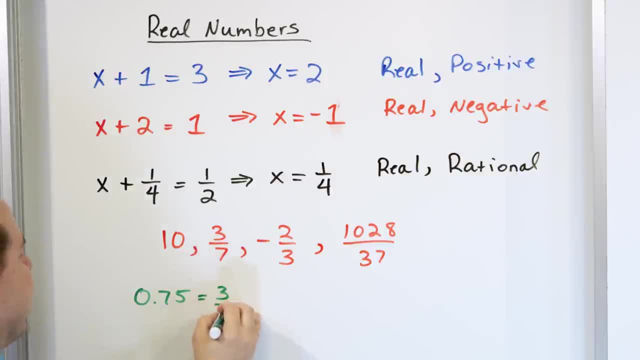 that's not. that's not a fraction. however, you know you can write this as 3, 4ths. that's a fraction. so this decimal is disguised, it's a rational number 2 and turns out that other decimals are rational, for instance 2, point 1, 2, 5, any 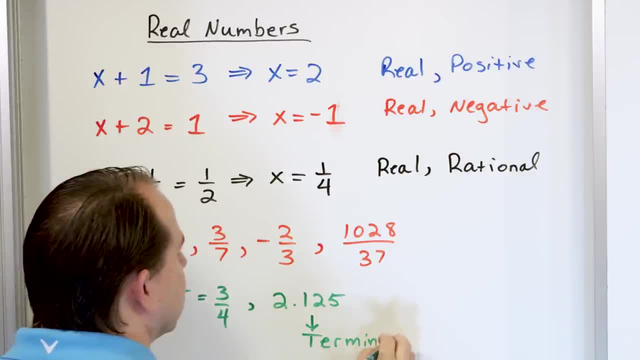 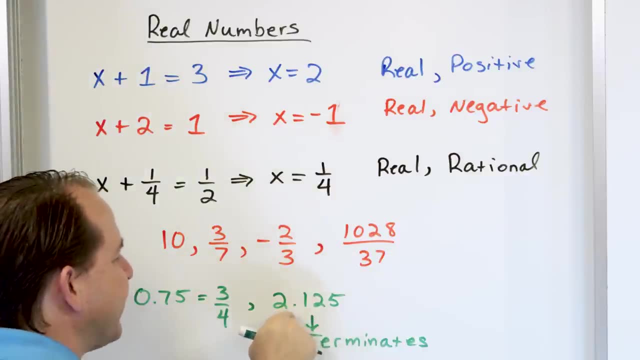 decimal that terminates terminates any decimal that terminates like this. that can also always be written as a fraction. so this is a rational number, but I'm not two. I can go find a fraction that's equal to this, right, Let's take our last crazy one. What? 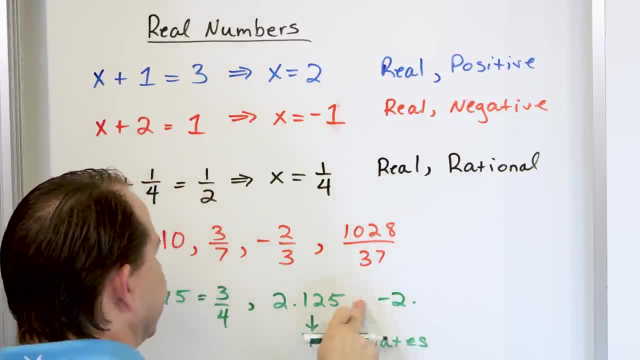 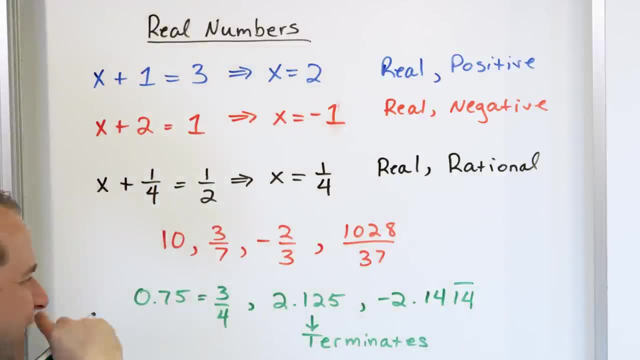 about two negative two point. uh, I don't. that's not an equal sign there. Sorry about that Negative 2.1414, but I'm going to put a repeating bar over the last one four. So this is 2.1414141414141414. 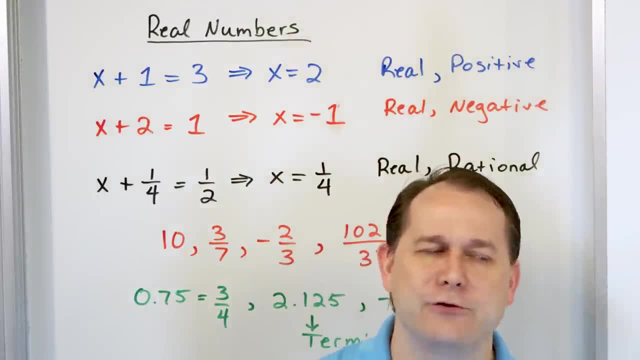 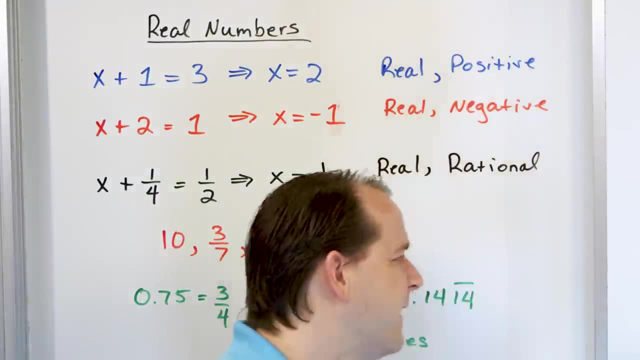 goes on forever, As long as you have a repeating pattern in your decimal. you may have learned this in previous lessons in algebra or in other math classes. As long as it's some sort of repeating pattern, then it's always rational. I can find a fraction that this is that that's equal to this. 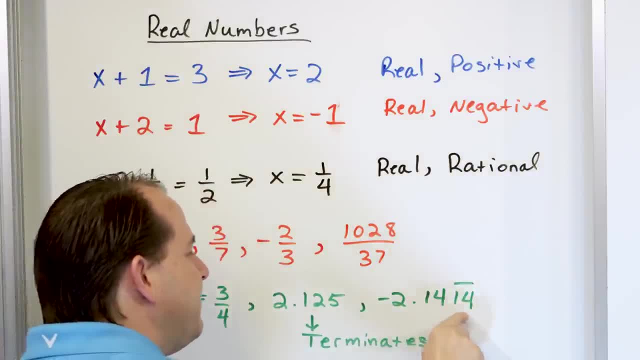 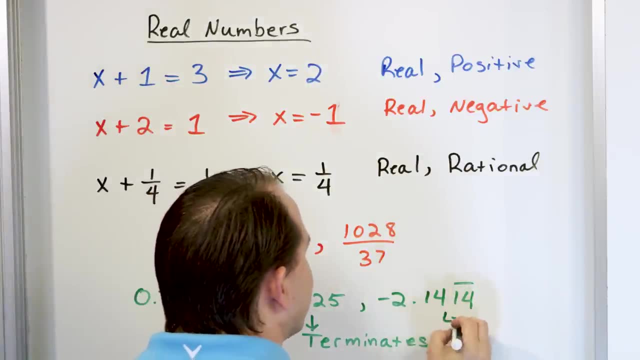 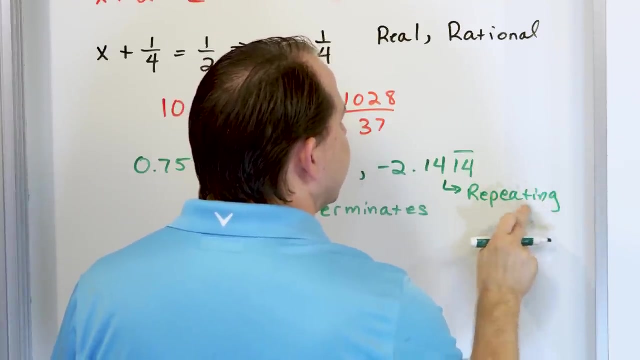 even though the decimal goes on to infinity, as long as it is repeating like this, I can call it. I can find a fraction that's equal to that, All right, So I'm going to write down: this is a repeating Decimal. Let's put the G here: Decimal. 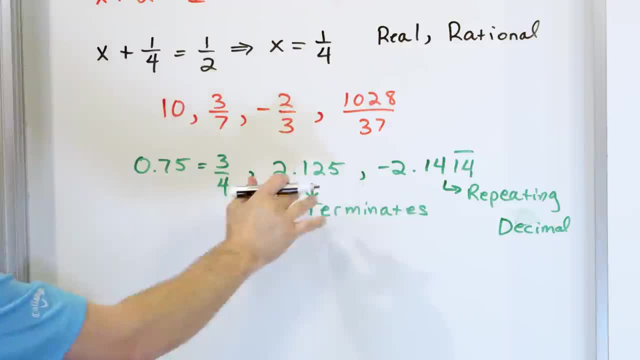 Why am I going through all this stuff? Because all of these, every one of these things, pretty much every number that you've really been exposed to up until now has been a real number and it's been a rational number. So these are all rational, right, But the point is is that throughout, 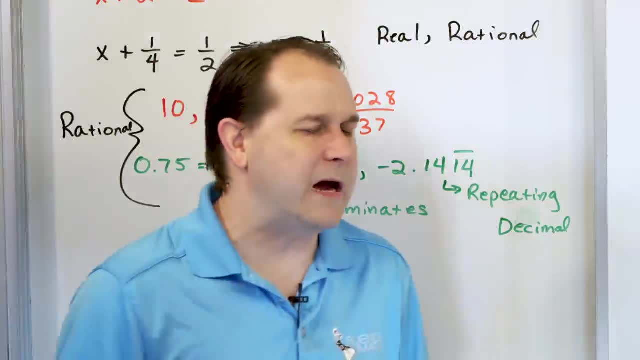 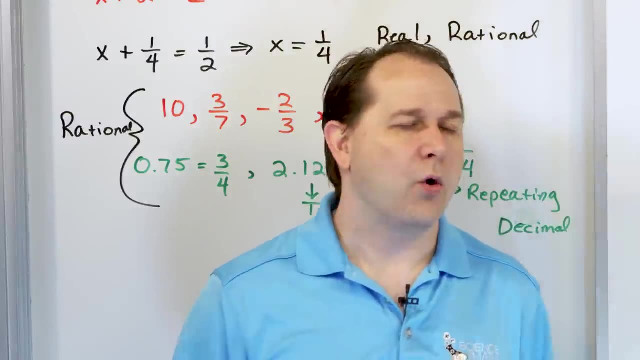 history. first, we didn't need to know about fractions. At some point in time there was some person that decided that it was useful to know what a half of a loaf of bread was and represent it as one half right Or three quarters of a dollar is worth something. So somebody had to. 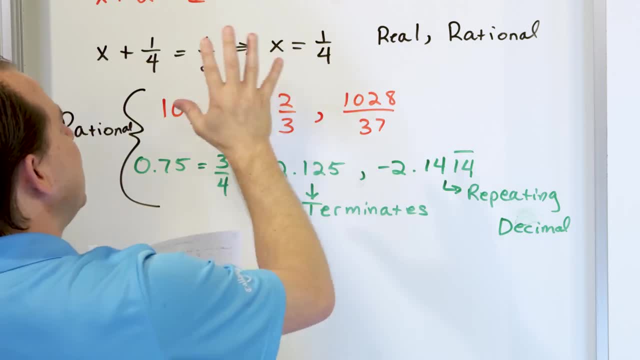 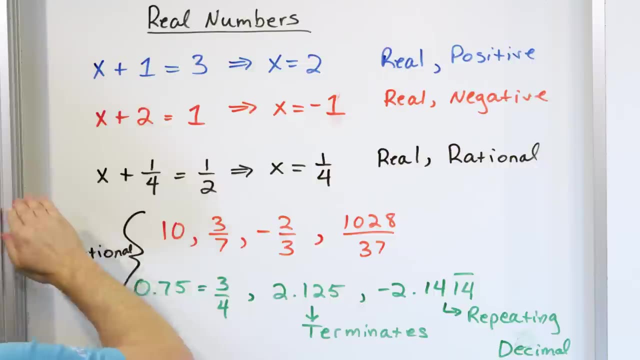 invent fractions. But these, these uh, different types of numbers that we've used, have all been invented to solve different kinds of equations. This one requires real positive numbers. This one requires real negative numbers, This one requires real rational numbers. And then, once we figure, 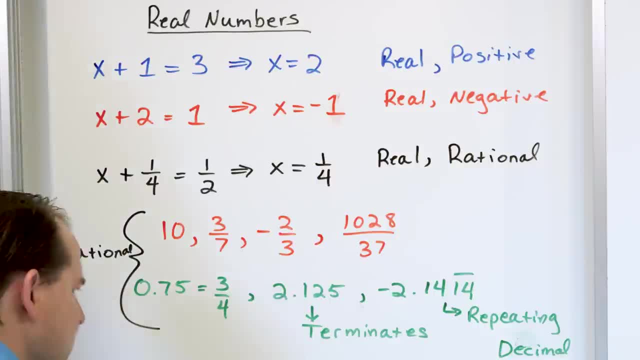 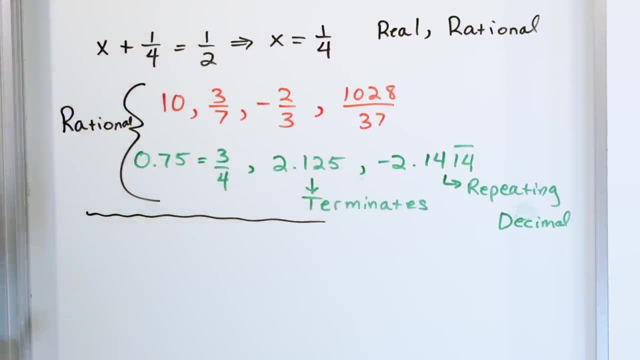 that out, we realized these are also rational numbers too. But then a long time ago, probably the ancient Greeks- I'm not totally sure, but probably the ancient Greeks um- figured out that some numbers do not terminate like this: The decimals don't stop. And also, if the decimals go, 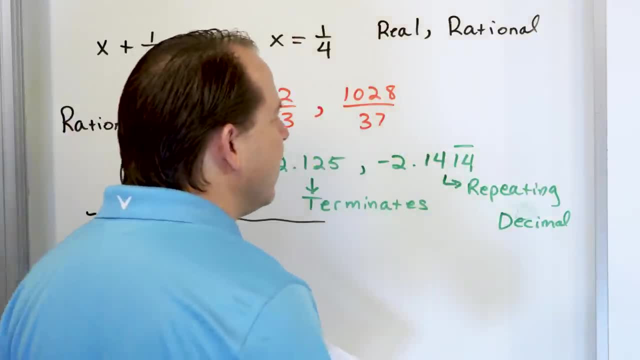 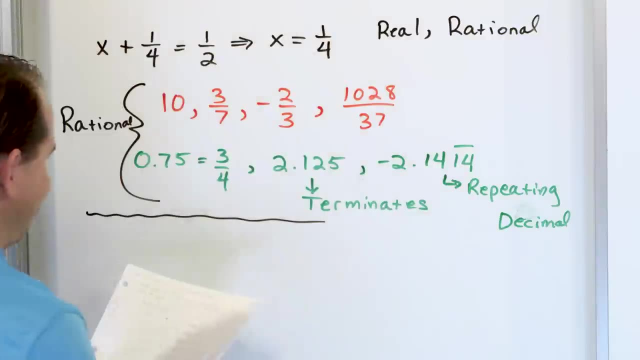 on and on forever. there are some special numbers that don't have any repeating pattern, Like this was one four, one, four, one, four, on forever. There are some numbers that have infinite decimals but they don't repeat in any pattern that we know about, And those are uh. 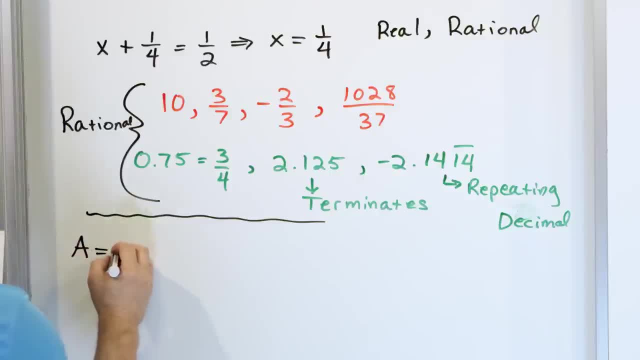 useful to solve certain kinds of equations as well. So the famous equation: the area of a circle is pi times r squared. You know that equation? Of course you do. Everybody learns that equation back in fifth or sixth grade, right? But in order to solve this equation we need to invent a new. 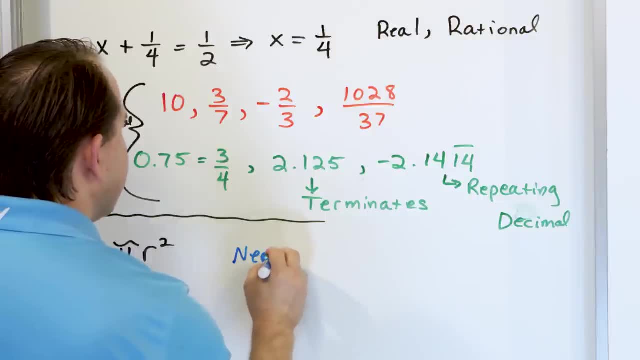 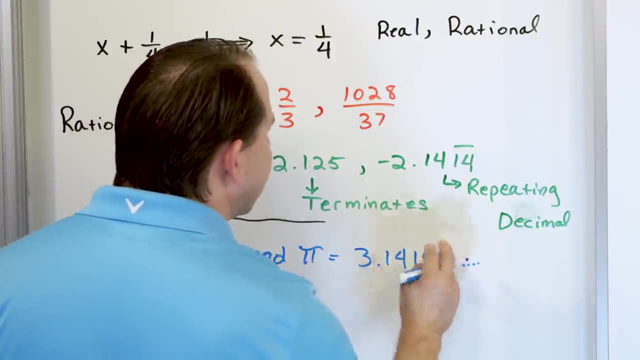 kind of number right. So we need whoops, we need pi right, Which can be a decimal, And you know, pi has been approximately written as 3.14159. dot, dot, dot, dot, dot. It goes. 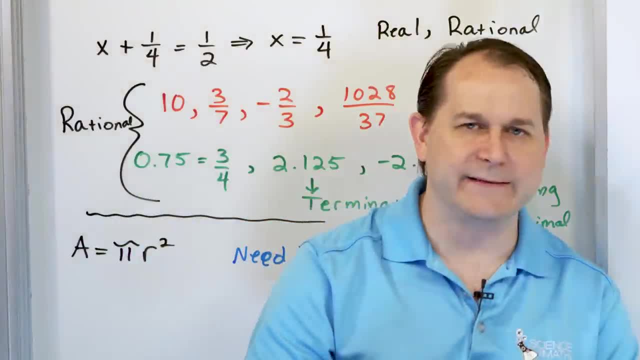 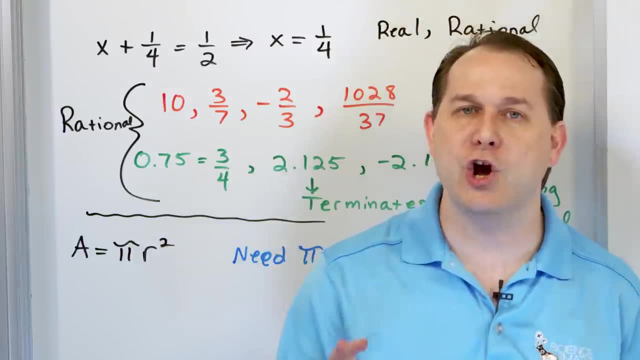 on and on forever, But the pattern of the decimal, this one, four, one, five, nine, it never repeats. We have super computers calculating pi out to 100,000, million, trillion decimal places. There is no pattern to pi. It's called an irrational number because the rational numbers can be. 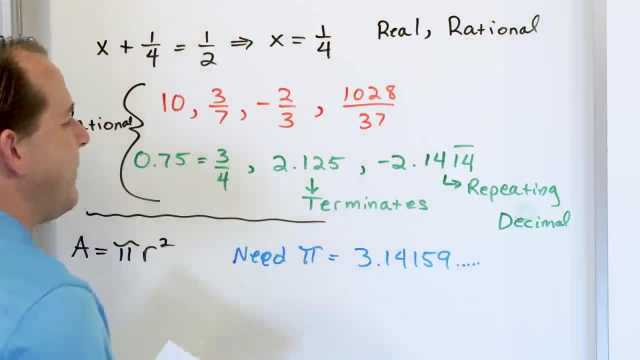 written as fractions because they have decimals that either stop or they go on forever in a pattern never needed before. but we need this number to solve this kind of equation. The area of a circle requires an irrational number, So this is called this. 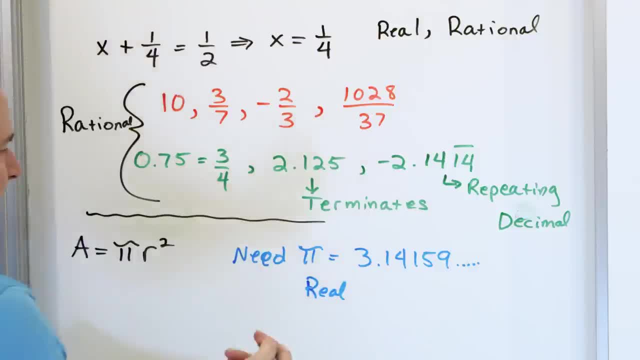 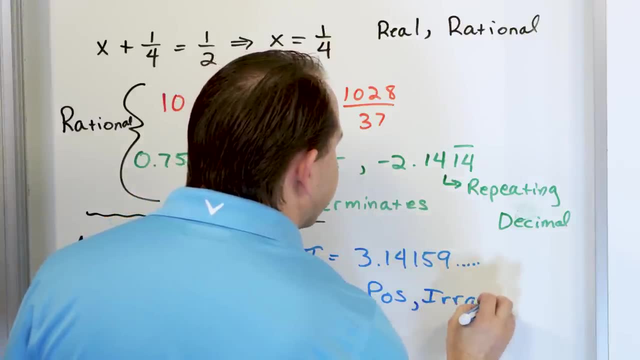 is real. of course this is a real number, right, I can hold it in my hand. of course It's a positive number- I'm gonna put POS for that. but it's a new kind of number called an irrational number And that means I cannot write that as a. 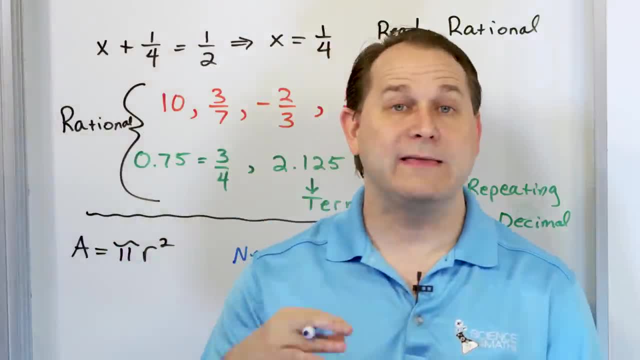 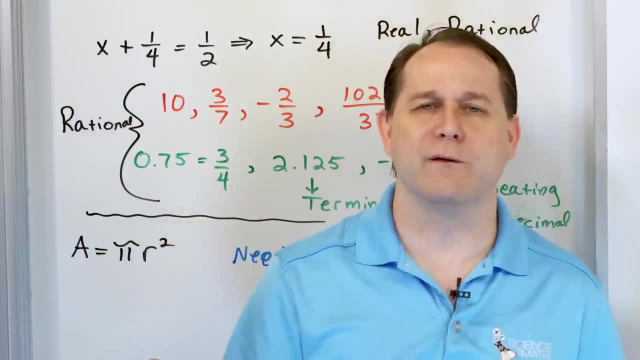 fraction. There is no way to write pi as a fraction. You may think: well, I should say there's no way to write pi as a fraction of whole numbers. You can't write it as 22 over 7.. Some people say pi is 22 over 7.. That's just an. 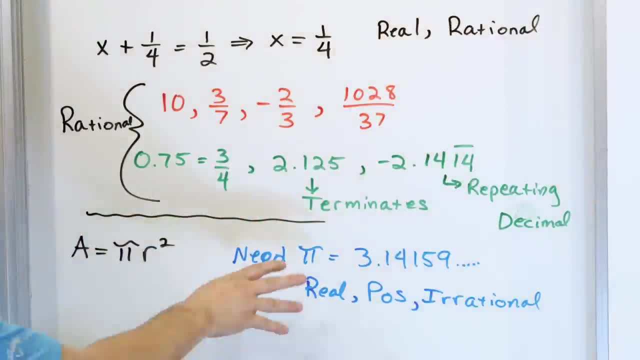 approximation. It's not the true value of pi, right, But this is not the only irrational number that we've discovered. We have tons of irrational numbers We have. let's talk about another equation. What about? x squared is equal to 2? This? 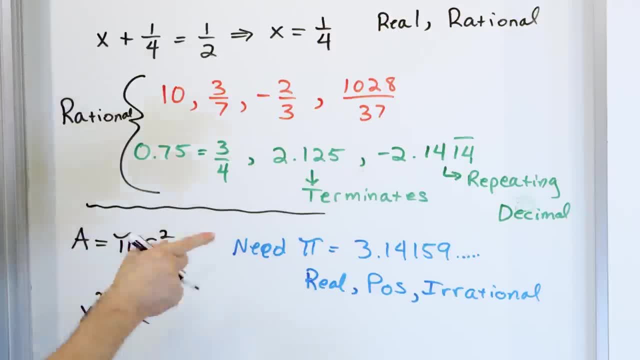 is another kind of equation. How do I solve this equation? I'm gonna take the square root of both sides right. So that means I'm gonna say that x is equal to plus or minus the square root of 2.. We've learned about that. and if 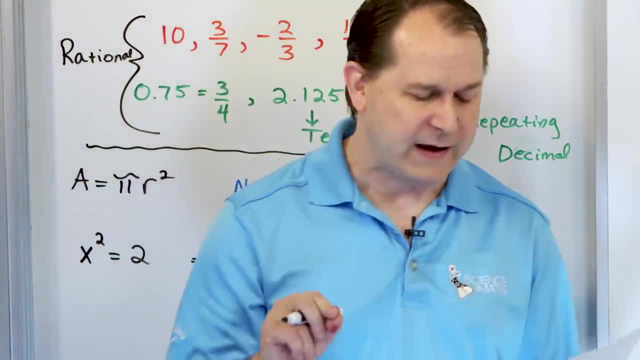 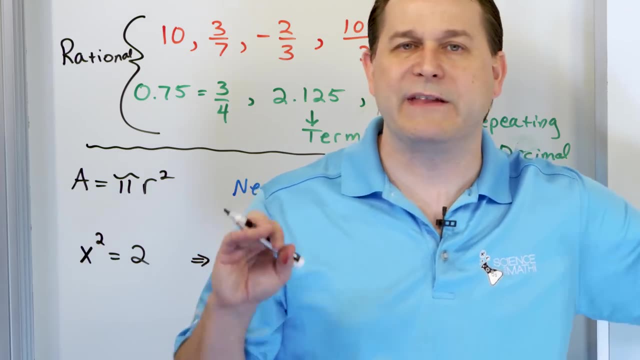 you take the square root of 2 and you stick it in your calculator and you look at the decimals. there is no repeating pattern to the square root of 2.. It's an infinite number of decimals, that numbers that go beyond the decimal, but there is. 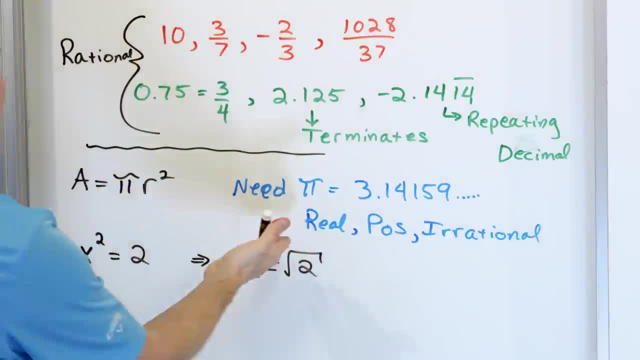 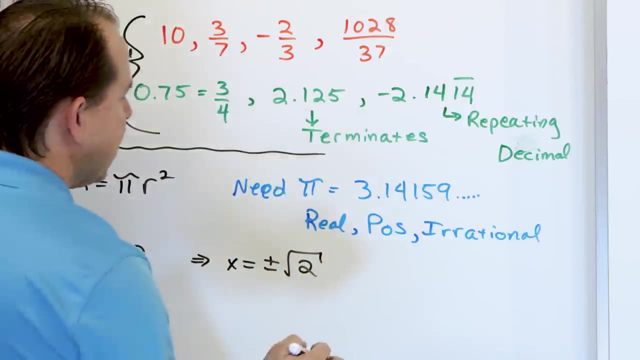 no pattern, just like pi has no pattern. It is a irrational number. We cannot write the square root of 2 as any kind of fraction. So plus square root of 2 or minus square root of 2, let's say. well, we could just say the square root of 2 is: 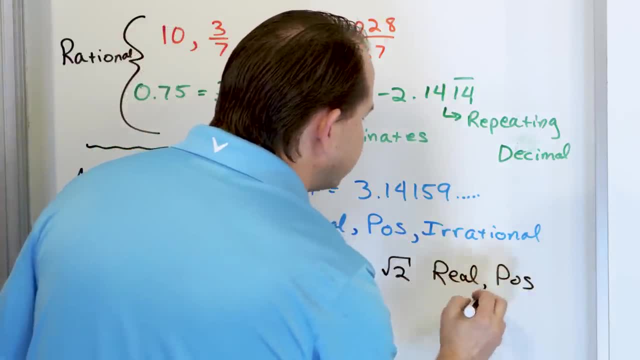 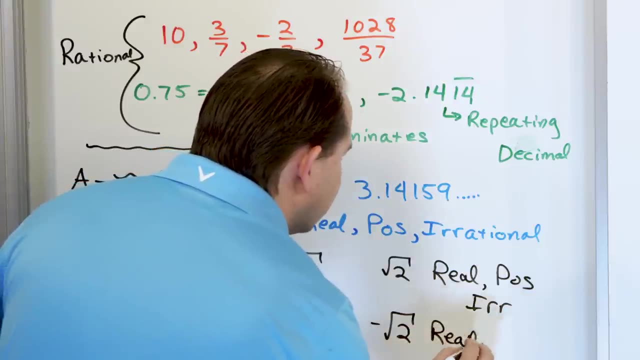 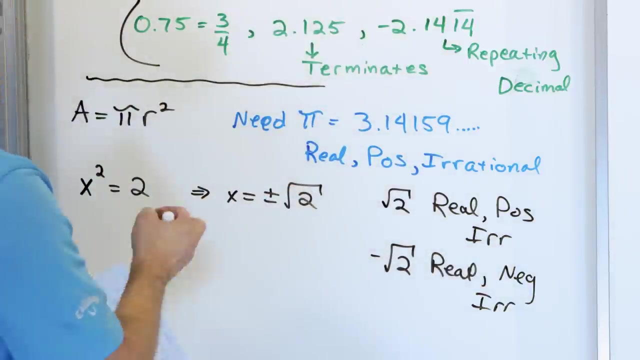 real, positive and irrational. I'll put I r for that- and negative. square root of 2 is real. whoops, instead of positive, it's negative. and it's also irrational because you cannot write it as a decimal, All right and it just in case you're curious. the square root of 2 is something: 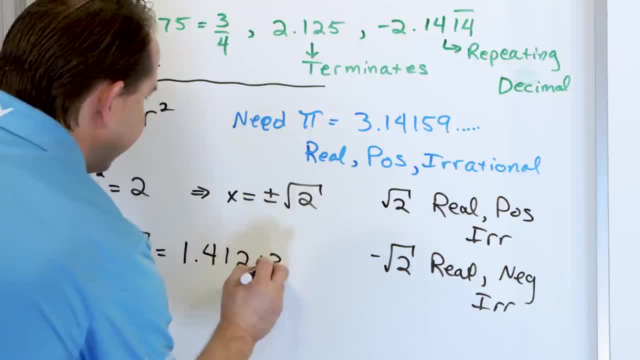 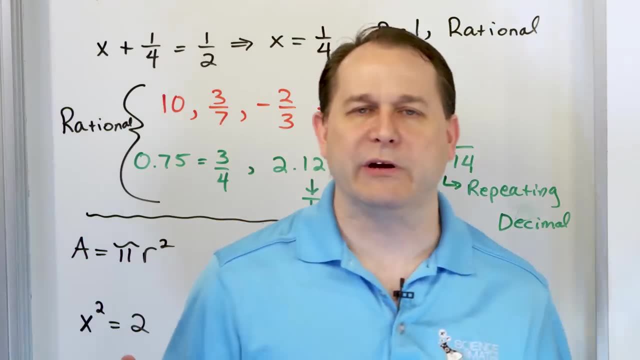 like 1.412135.. it does not repeat. It goes on and on forever and ever. We can calculate them. Now why am I going through this stripped-down memory lane? I think you can probably figure it out right. The reason is because all of these different 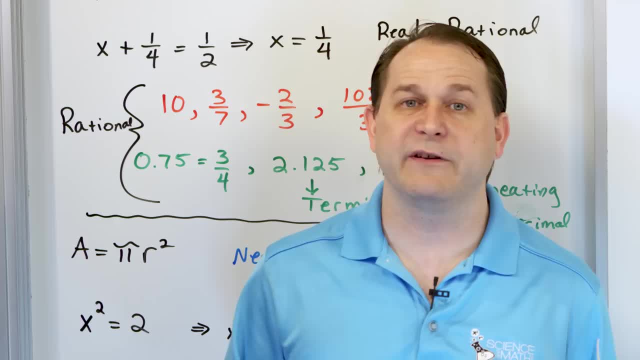 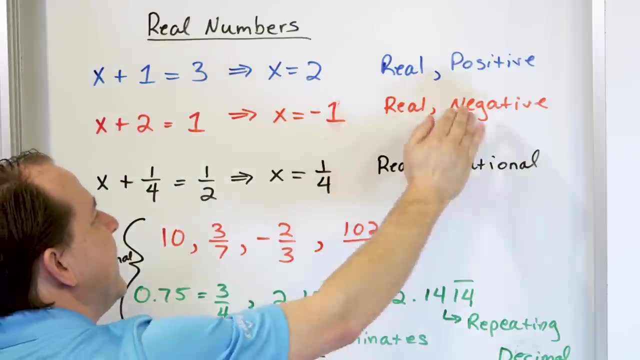 kinds of numbers that we have in math were invented at some point in time to solve certain kinds of equations that we needed to solve. The real positive numbers were used when we needed to solve that equation- The real negative numbers- we had to invent a negative number. 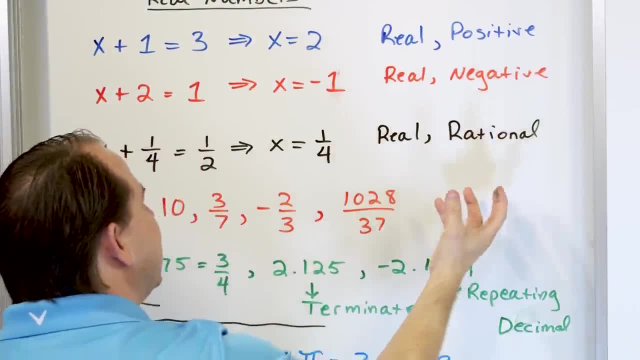 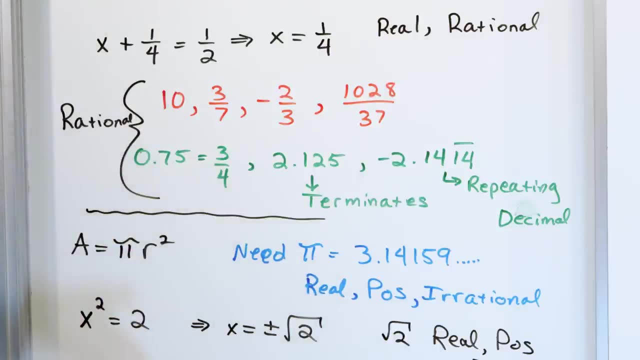 to solve this kind of equation, We needed to understand the idea of a fraction. in order to solve equations with fractions, We called them rational numbers, And then we had to have irrational numbers to solve certain kinds of equations that we have outlined here: Decimals. 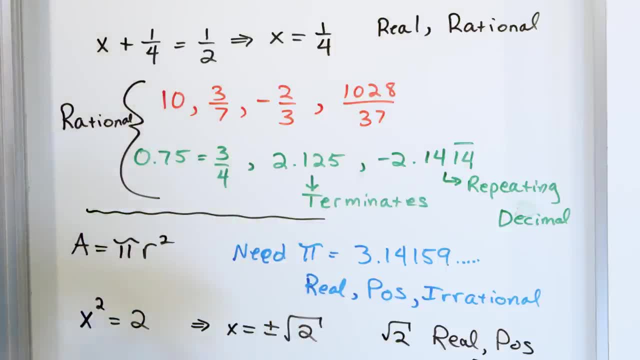 that go forever, that you cannot write the number as any kind of a fraction. And now we're taken to the very final part of the equation, which is the number of decimals that we need to solve, The famous i, the imaginary number. We invent the concept of. 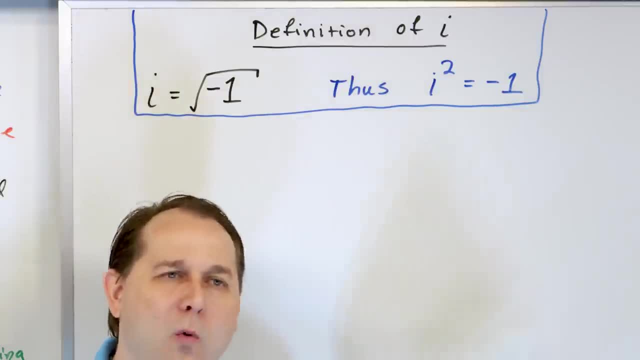 i because it is useful to solve certain equations that require i as a solution, that require the square root of negative numbers. That is the reason why we have i, because we have to have it to solve certain kinds of equations, And these equations that we're going to learn. 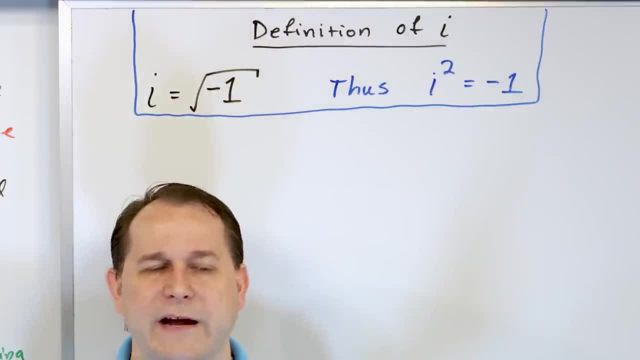 in algebra we're going to solve tons of equations that have i as an answer. right, You're going to get them, you're going to circle them, you're going to say great, But the truth is, we use i probably more than almost anything else in math and higher-level learning to 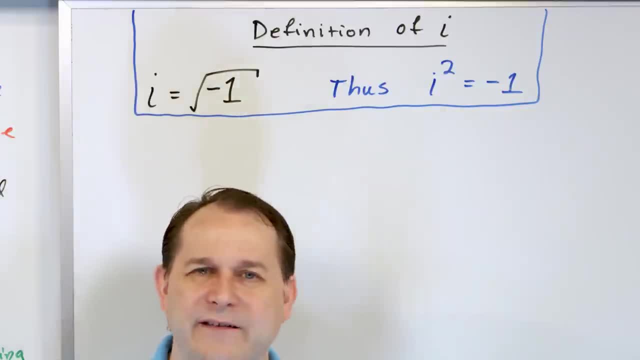 solve all kinds of things: Quantum mechanics, advanced physics and chemistry. almost always the solution to very common equations in advanced math actually use the concept of i in the solutions And I'm going to talk more about that at the very end where I'm going to give. 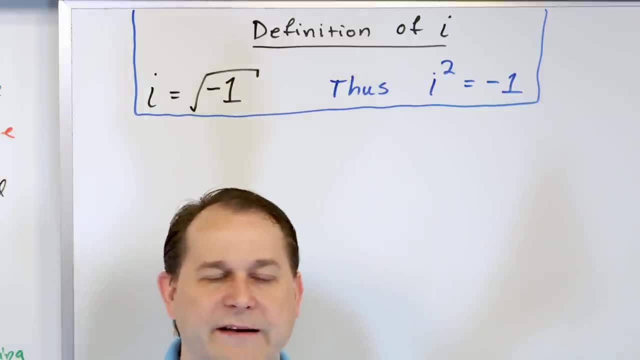 you a concrete example of that. But the idea is, we invent this concept of i to solve equations. What kind of equations do we need to solve? right, Let's solve this equation Very simple. I'm just going to put it to you like this: What if you have the equation x, squared is? 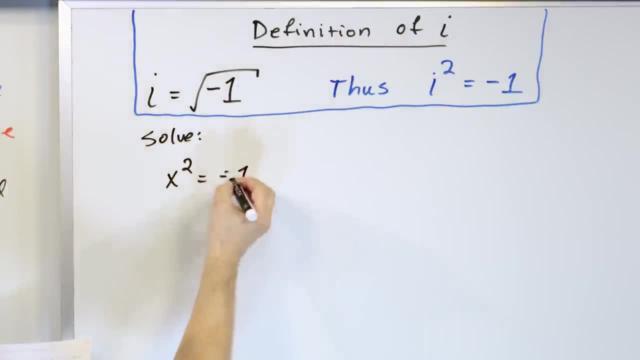 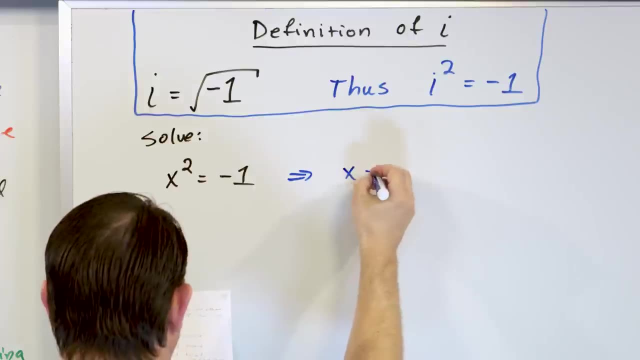 equal to negative 1?. How do you solve that? Well, in the previous lectures we would have just taken the square root of both sides. That's exactly what we're going to do. We're going to say that x is equal to, plus or minus, the square root of the right-hand side, negative 1.. But then 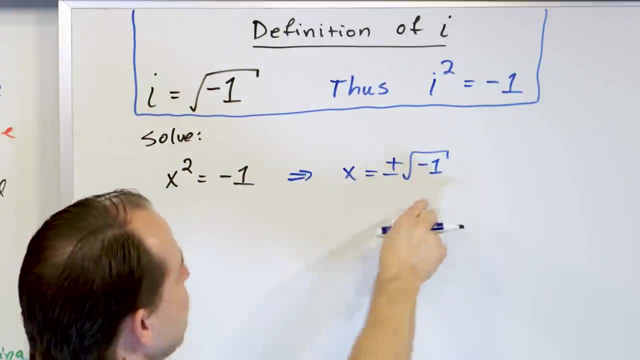 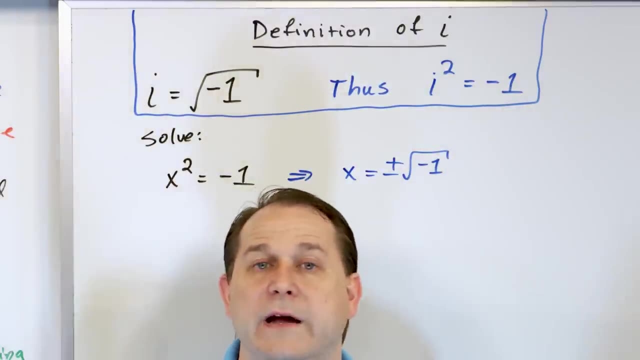 we say, well, we don't know how to take the square root of negative 1.. There is no real number that actually can be multiplied by itself to get me negative 1.. So up until now we just stopped And we said, well, we can't do that, It's undefined. But in higher math, 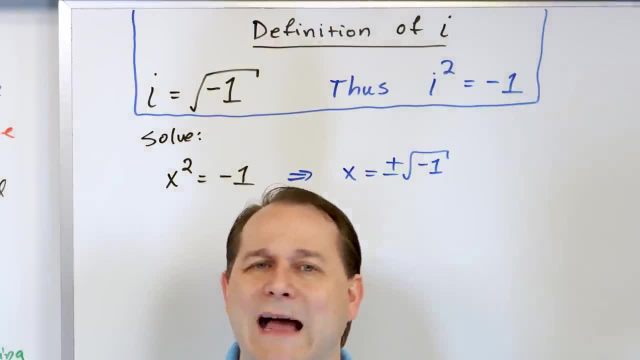 which is where you're at right now. we don't say it's undefined, We say there's a new kind of number to solve this equation, Just like we needed those new kinds of numbers to solve those equations. And this number is called the imaginary number. So we don't stop there, We go further And we say: let's. 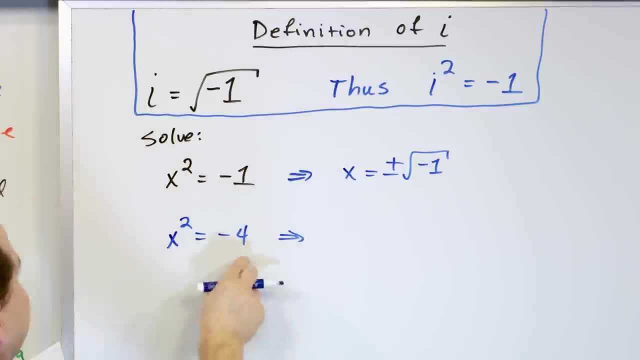 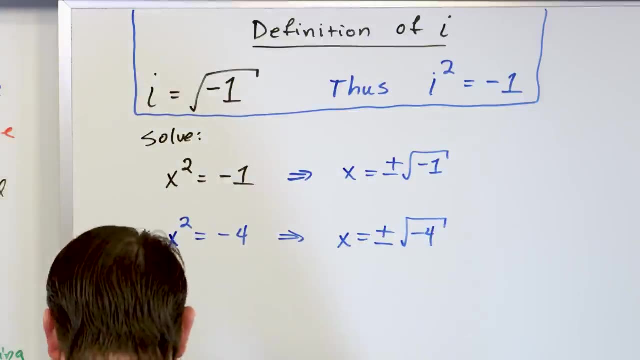 take another equation: x squared is equal to negative 4.. We do the same thing. We're going to take the square root of both sides. We say x is equal to plus or minus the square root of negative 4.. In the past we would have stopped there. We would have said well, 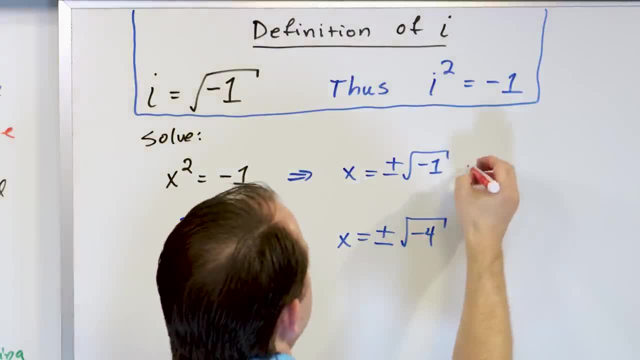 we don't have any answers, We're going to stop, It's undefined. But now we go further. We say that really x is equal to negative 1.. And we say: well, we don't have any answers, We're going to stop, It's undefined. But now we go further. We say that really x is equal. 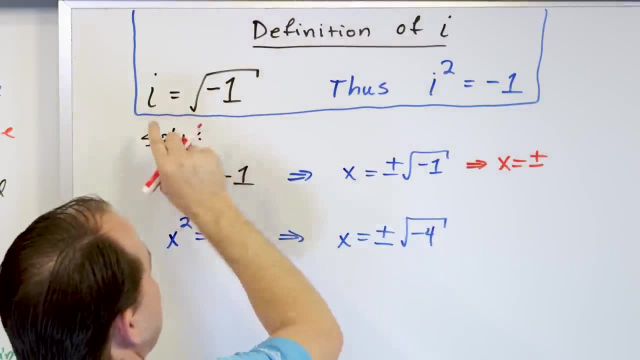 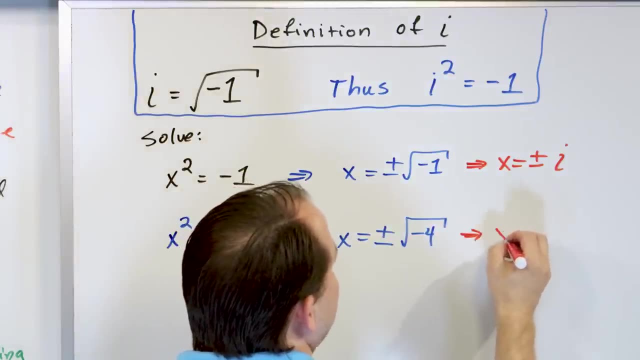 to plus or minus the square root of negative 1, which we're defining to be i. So we say plus or minus i. That's the answer to that equation Over here. we're going to do a lot more problems here. What we have here is the square root of negative 4.. You can kind of 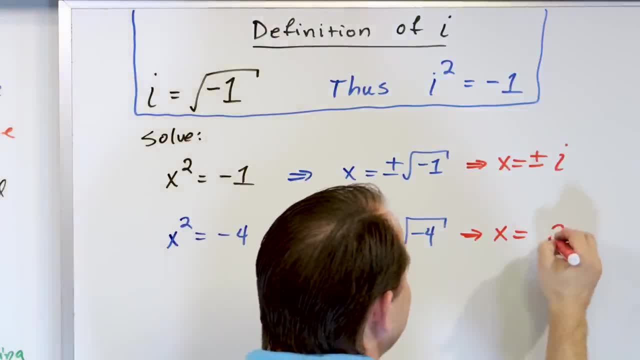 think of. we know how to take the square root of 4.. That's just 2.. But the square root of the negative 1 is still in there. When we take the square root of that, it's i, So it's. 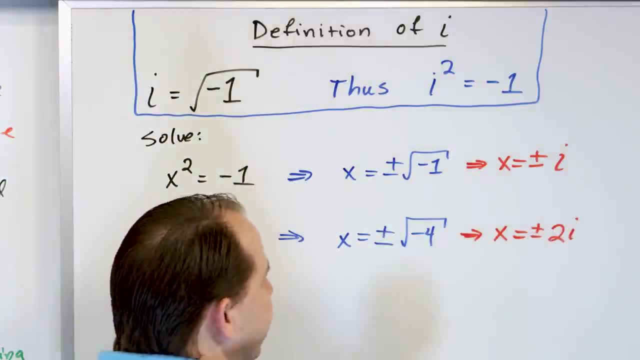 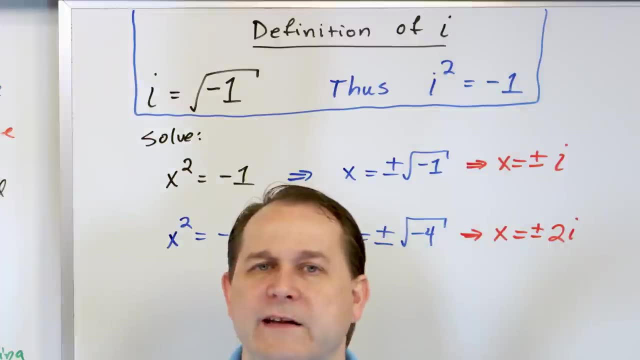 really 2i And we still have the plus or minus. So you see, the punchline is: when you take the square root of negative numbers, you're going to have the square root of negative numbers. You take them ignoring the negative sign, You just pretend the negative sign's. 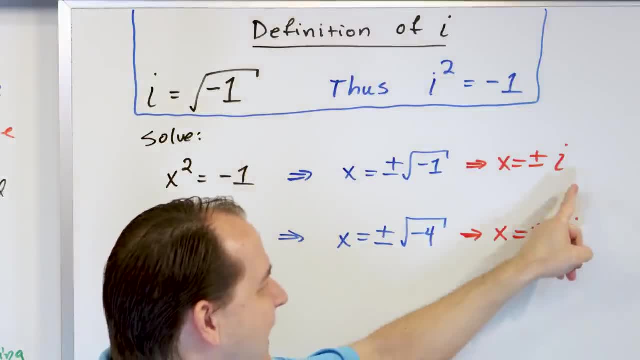 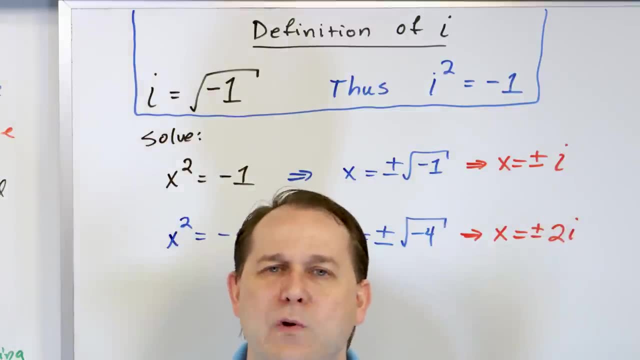 not there. You just write the number down, just like always, But then you tack an i on there because the negative inside of it produces an imaginary number. So this is not a real number. You cannot have 2i potatoes. You cannot have 6i strawberries- It's an imaginary number. 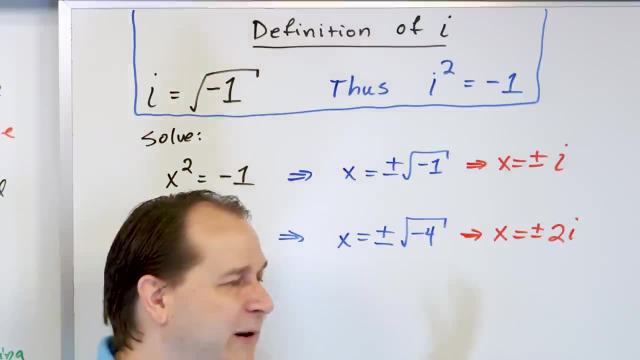 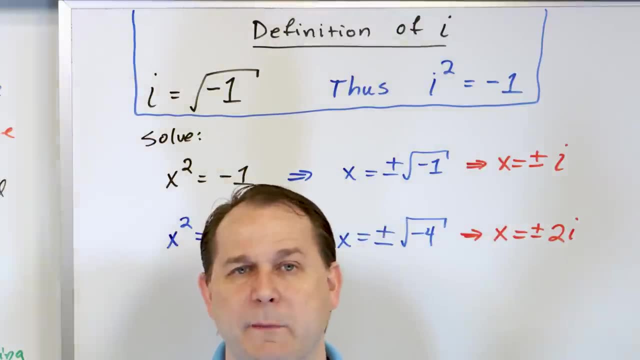 It doesn't exist in a tangible form that you can touch. However, as I've mentioned before, if I have 4i potatoes over here, as a solution of some equation I may have to multiply it with some other number of potatoes over here. When I can multiply those imaginary numbers, 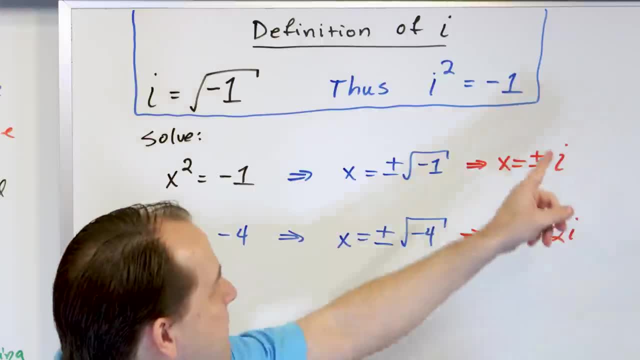 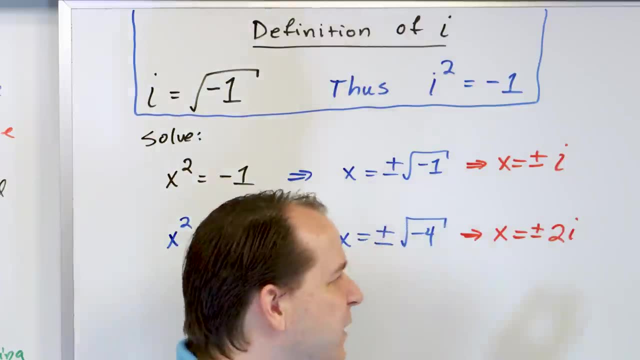 together, I get a real number back, Because when you square i, you always get a real number back. You get negative 1.. That's why imaginary numbers are useful. We say they don't exist initially, but now we say, hey, we're going to define an imaginary number, We're going 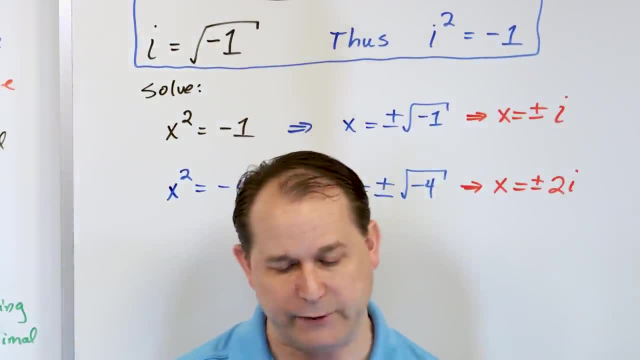 to keep track of them, But then sometimes they'll combine and give us real numbers back anyway. All right, Now what I want to do is solve some very simple additional problems. to give you practice, I'm going to be taking the square root of negative numbers And then, at the end of the 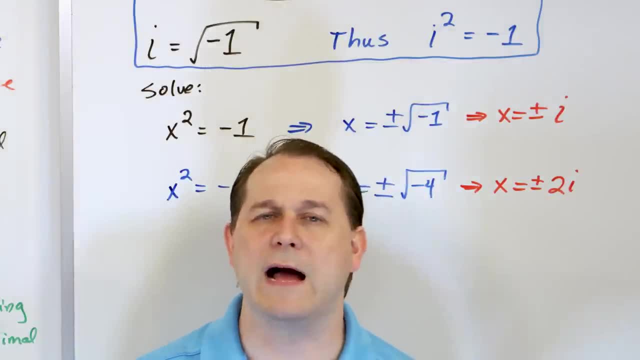 lesson. I'm going to do a little bit more into the philosophy of why imaginary numbers are useful for modern day stuff. So stick with me till the end and we'll get there. Let's solve some additional problems. Let's go over here. Let's say we have the square. 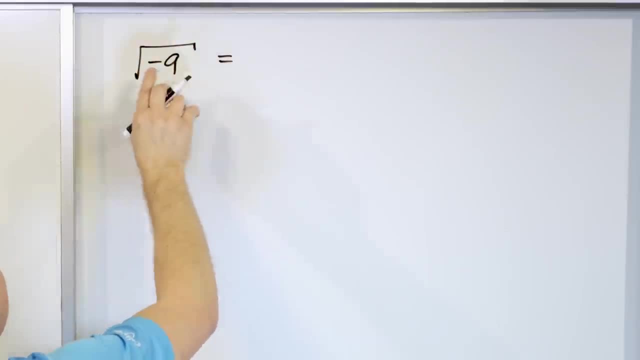 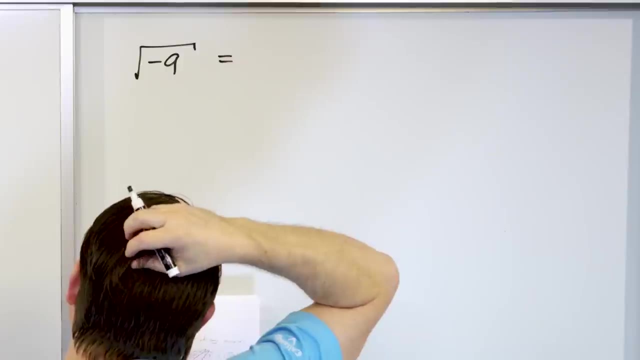 root of negative 9.. As I said, you just ignore the negative. You pretend that it's the square root of 9.. You already know what that is. That is a 3,. right, You know what the square root of negative 1 is. That's just going to be i, So let me. 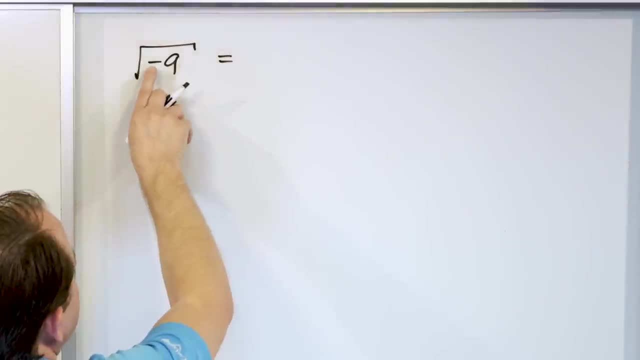 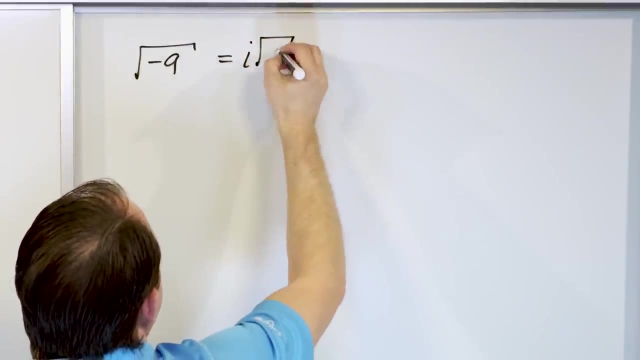 just take it a little bit more, step by step. If you take the square root of the negative inside- kind of pull it out and take the square root- you're going to get the i of the negative 1. But you'll still have this square root. 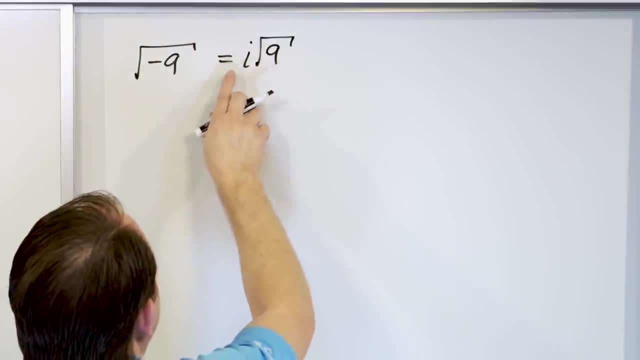 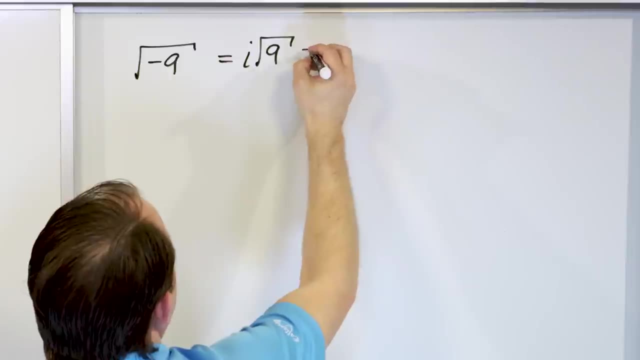 of 9 left over. So this is equal to the i. That i comes about because we're taking the square root of the negative 1 in there. Poof, it turns into an i, But the square root of 9 is still left over, which you all know is 3.. So you can write it as i times 3, if you. 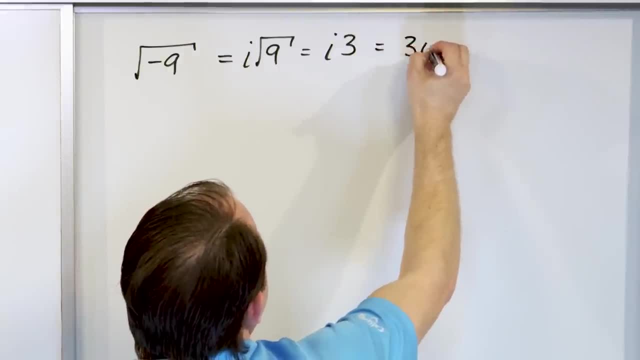 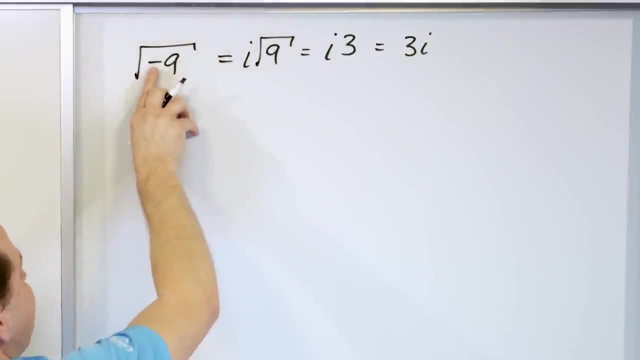 want. But the way we write imaginary numbers is we always put the number in the square root of the negative 1.. We always put the number first. So we say that the square root of negative 9 is 3i. So what you do is you take the square root of the number and then, any time you have, 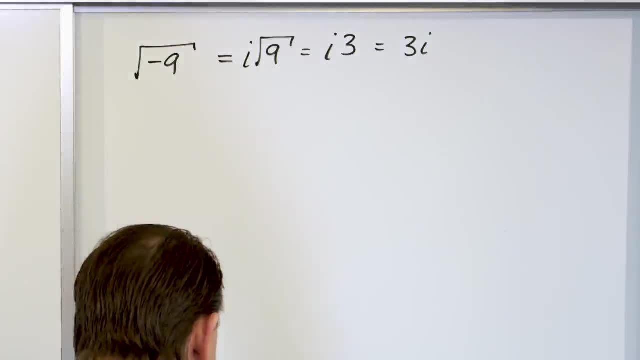 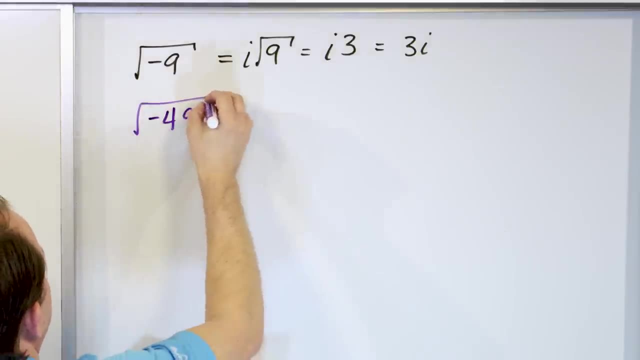 a negative there. you just have to tack an i at the end. That's all you do. It's extremely, extremely easy to work with imaginary numbers, So let's take some more rapid fire examples. Square root of 49.. You know what? the square. 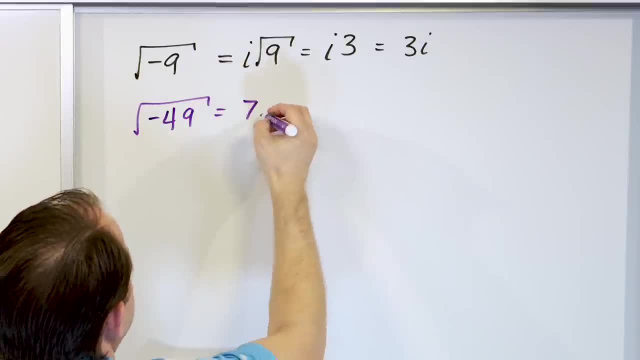 root of 49 is It's 7.. But you have that negative, so you have to take the square root of that too, so you get 7i. That's the final answer of this problem. This is the final answer of this problem. 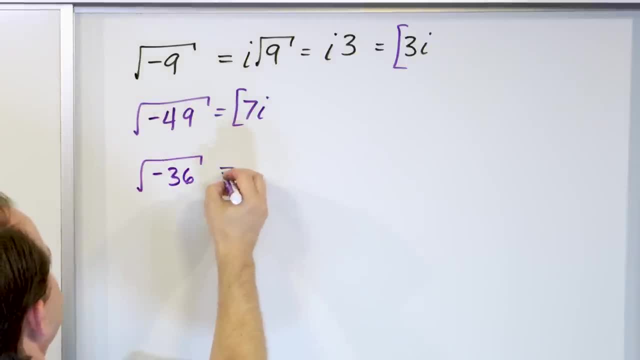 What if I have the square root of negative 36?? I think you can see the pattern here. We know that 6 times 6 is 36.. And the square root of negative 1 there is the i. So that's not a real number. This is an imaginary number 6 times the base number that we call i. What? 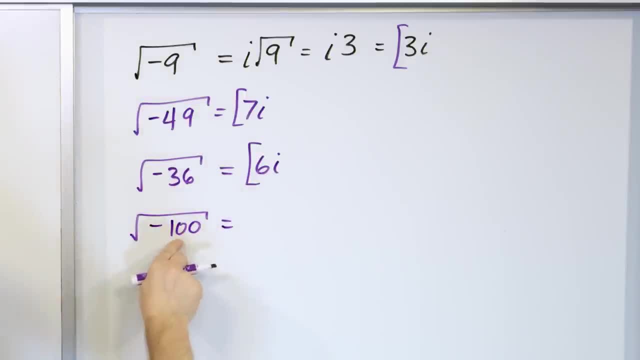 about negative 100?? We're going to take the square root of this. Well, we know how to take the square root of 100.. That's 10.. And the square root of the negative there means we have to put an i there, So that's a 10i Right Now. we learned. up until now we've 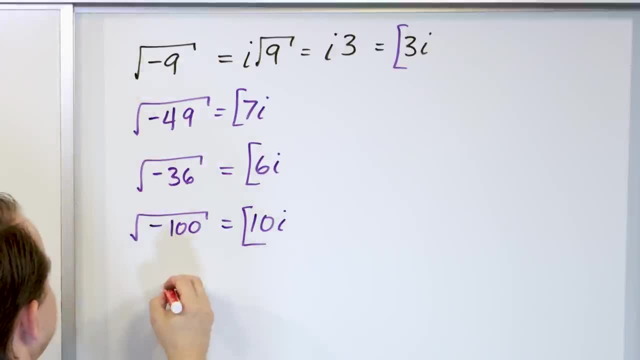 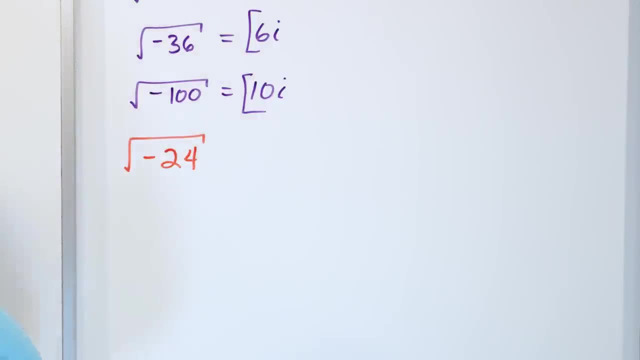 had to take the square root of much more complicated things than these simple things. We've learned how to take the square root of things like 24.. But what if you had the square root of negative 24?? So what you're going to do is you're going to completely ignore the negative. 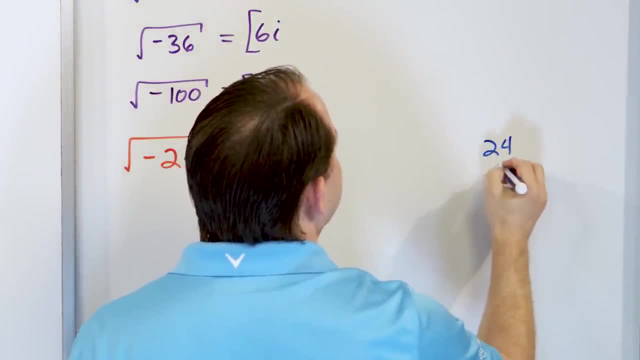 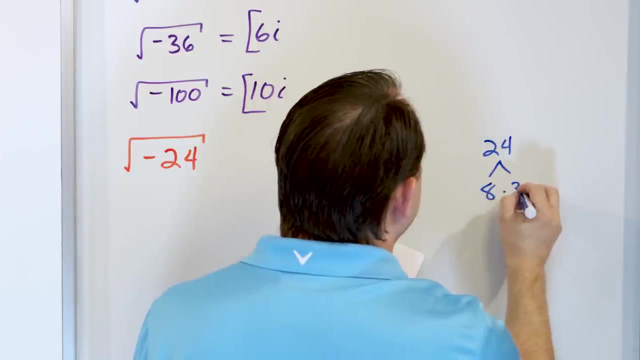 sign there, You're going to come over to the side of your paper and you're going to write that 24 down and build a factor tree. like always, You're going to ignore the negative. So for 24,, you know that 8 times 3 is 24.. But you know that 8 is 2 times 4.. And you 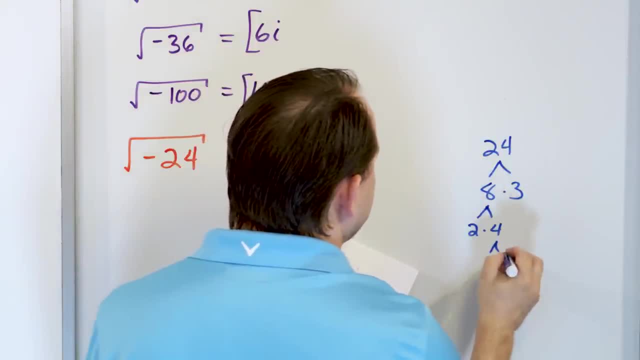 know that 4 is 2 times 2.. So you've got your tree built, You're looking for square roots. So that's a pair. I still have a 2 into 3 left over Right, So what you have is when: 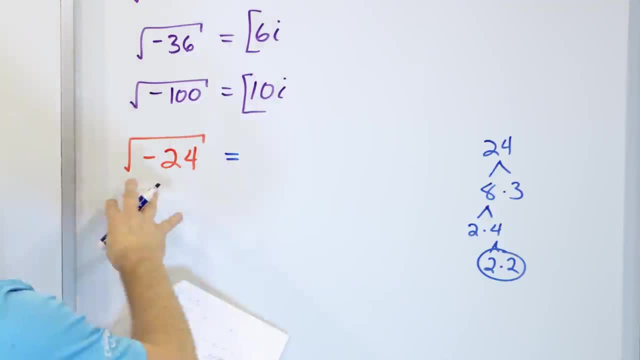 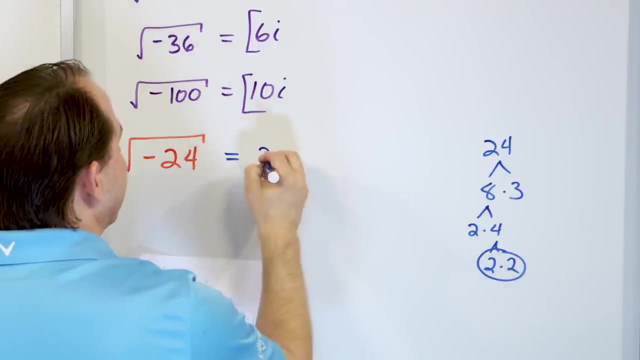 you write the answer here, the square root of negative 24, you just pretend that the negative is completely gone. And so if there was no negative there at all, I would take a single 2 out. I would have a square root of 2 times 3 is 6.. Right, I would have that. 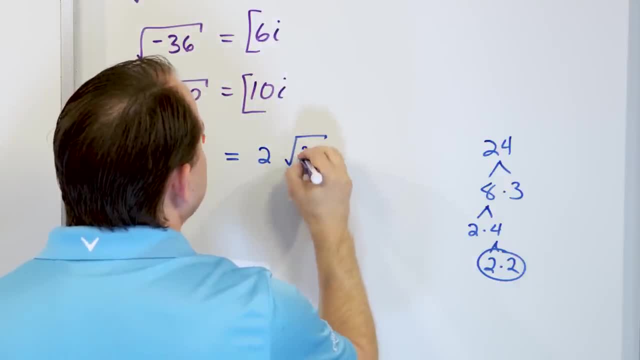 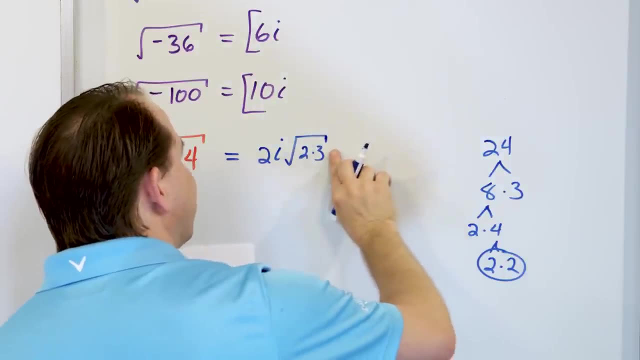 left over. Let me write it explicitly On the inside: it would be 2 times 3 left over. However, because I took the square root of that negative, I still have an i here. Right, We don't usually write the i after the radical. I mean it's all multiplied. 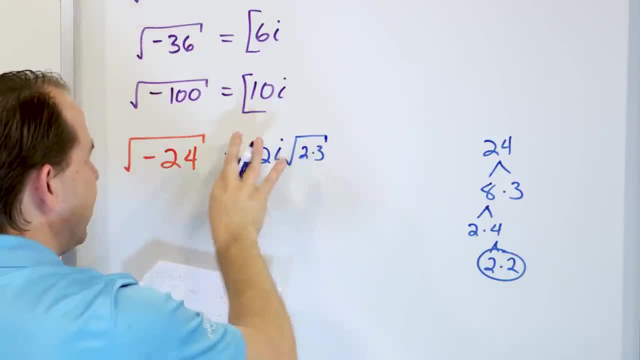 It doesn't really matter if you put the i here, We put it in front of the radical to keep it away, Because if you put the i at the end you might accidentally leave it under the radical And you don't want that, Right i's. do not imaginary numbers, do not live. 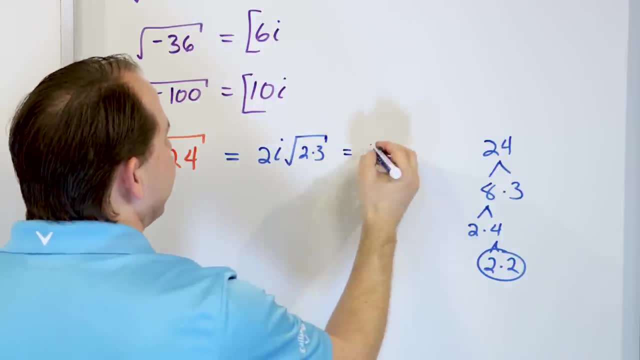 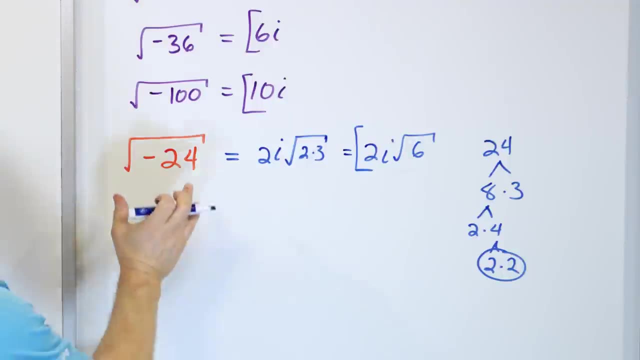 under the radical in general. So 2i times the square root of 2 times 3.. So it's 2 times i times the square root of 6.. This is the answer to this problem. So, whereas before we don't know what the square root of this negative 24 is, here's: 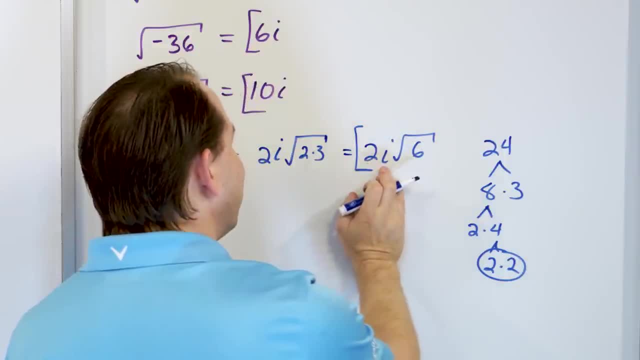 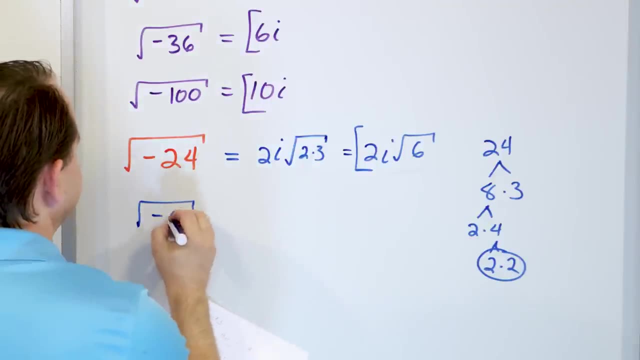 where you can see all we're doing is we're writing the square root as if it were positive under the radical, but then tacking an i on because it's an imaginary number. So working with these imaginary numbers is exceedingly easy. Right? What if you have the square root? 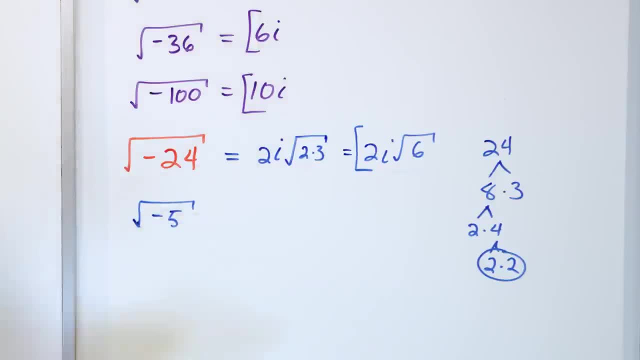 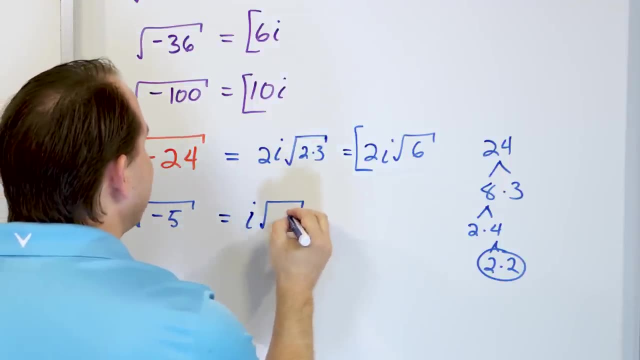 of negative 5?? Well, we can't simplify the negative 5.. There's no factor tree that's going to help us, But we can take the square root of this negative 1 in there, So that comes out as an i, But what's left over is what's underneath this, The square root of 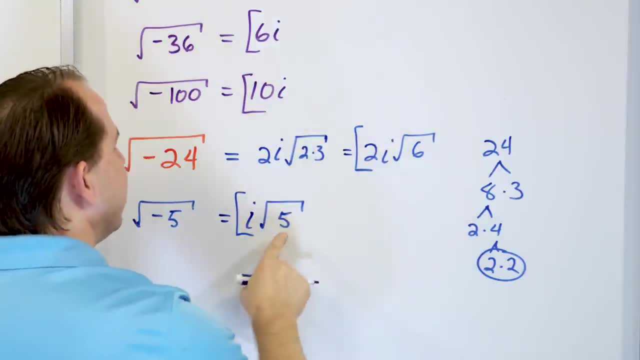 5 is left over, Just like we had a left over 6 here in our answer. we have to leave it as a square root There as well. So at the end of the day, you should never, ever, have negative numbers under. 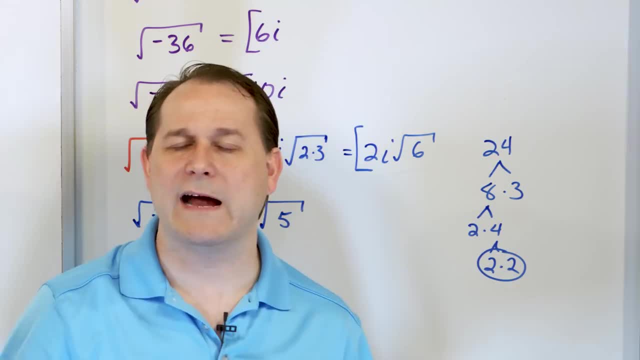 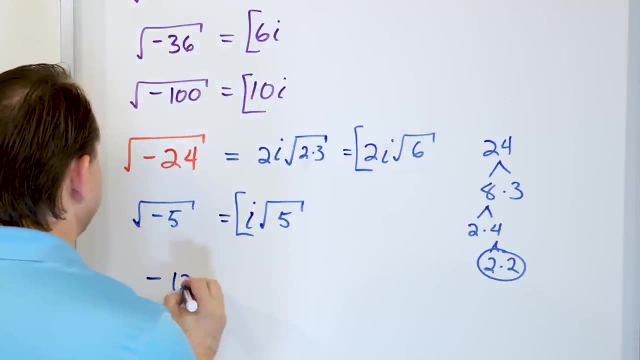 a radical. If the only thing you do is just pull the negative 1 out as an i, then that's fine. Can't do anything else with the 5. Leave it there under that radical. What about the square root of negative 12? Right, Same sort of thing. You pretend this. 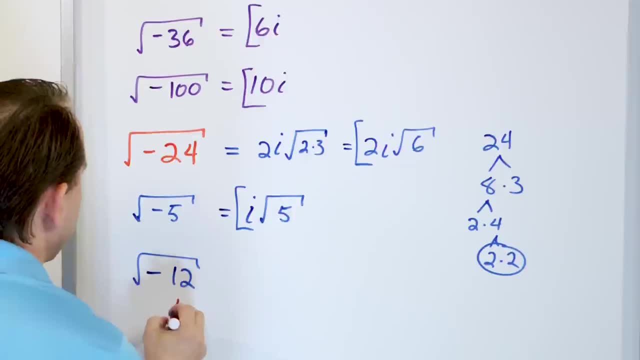 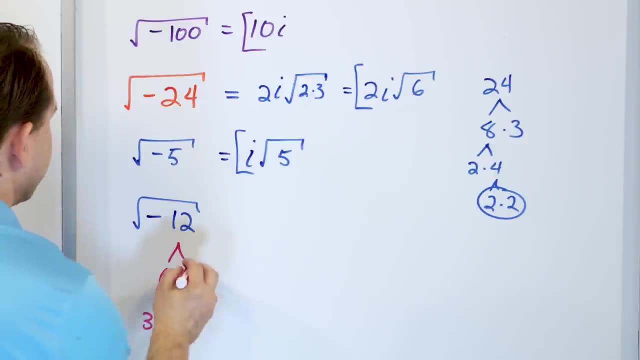 is a positive number. You go over here, Or I guess you could go underneath if you want, But just ignore this. When you build your factor tree, ignore it. You can say 6 times 2.. And 6 is 3 times 2.. You're looking for pairs, So there's your pair right there. So 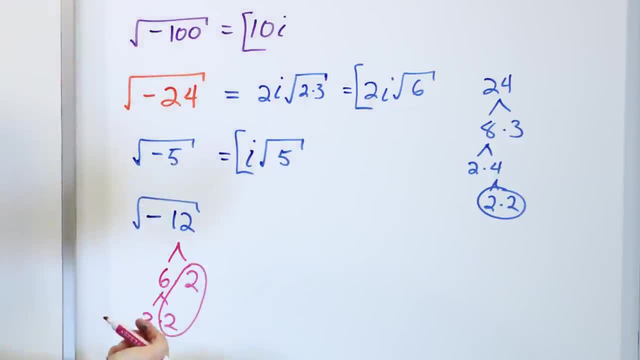 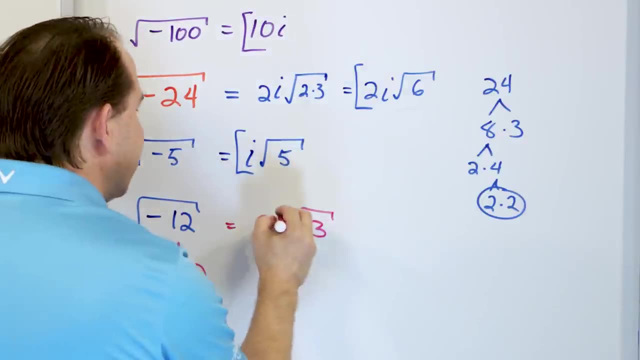 if there were no negative number there, the 2 would come out, And then underneath you would have a square root of 3, which is left over, But you still have the square root of this negative 1, which means an i comes out, So it's 2 times i times the square root of. 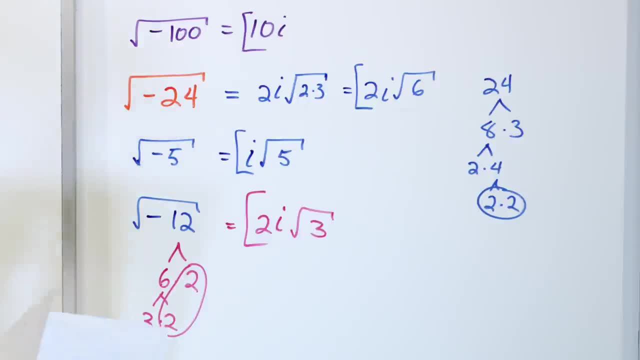 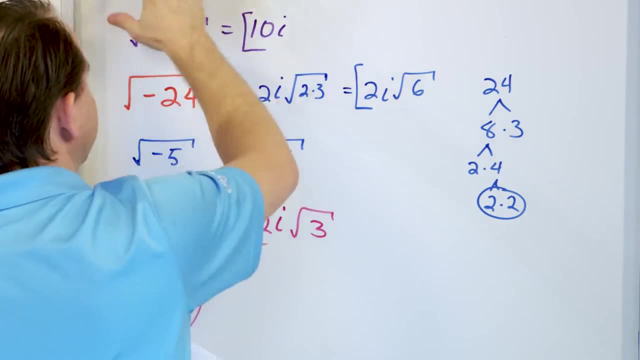 3. Now on this page, what I have done is I have tried to show you a basic idea about how to take square roots of negative numbers. So you just do the factor tree as usual, And if you have a negative under there, you just. 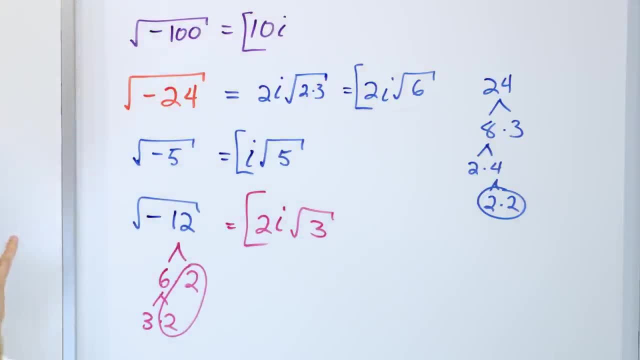 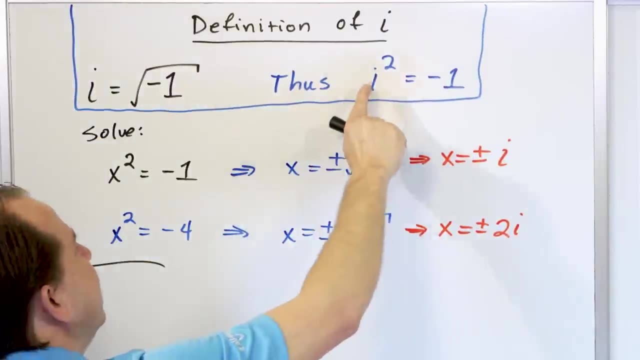 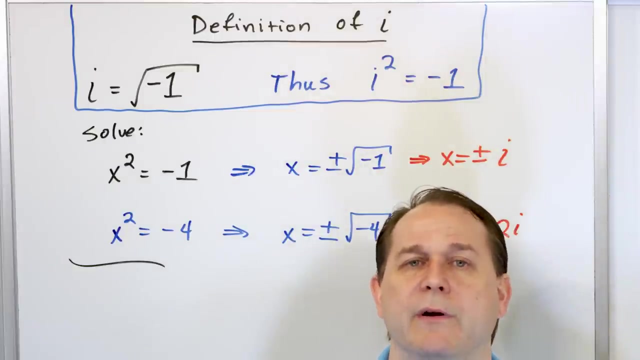 tack an i on Extremely simple. All right. But we also learned another property of this imaginary number. Because it's defined this way, the i squared the i times itself is not imaginary anymore. It's equal to a negative 1, which is a real number. 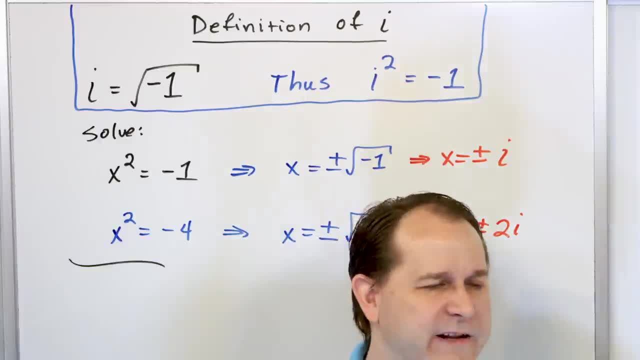 So any time in an equation you see an i squared, then in the very next step you just substitute negative 1.. You don't have to think about it, You don't have to derive it or calculate it. If you have an i squared you just write down negative 1.. 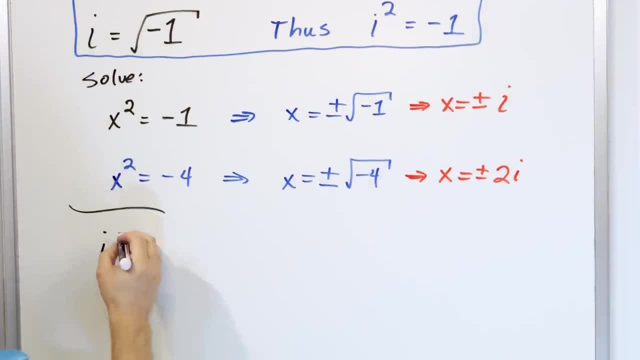 So because of that, we can do some simple problems here. So let's just get some practice. The simplest one is: what is i squared? You just replace it with negative 1. You don't have to think about it, You don't have to prove it. 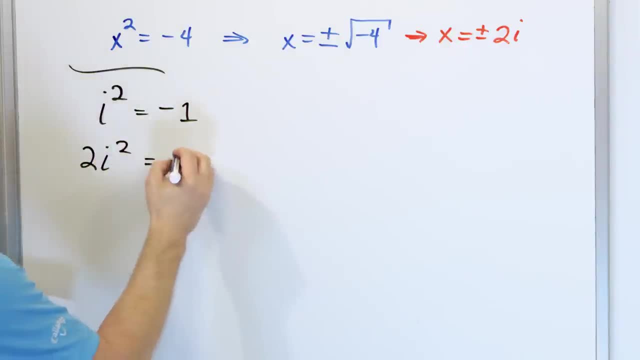 What if I have 2 times i squared? Well, the 2 is totally normal, But the i squared is negative 1.. So you just substitute for i squared, negative 1. And the answer to this is negative 2.. So you see what I mean. how you have two imaginary numbers multiplied together, But at the end 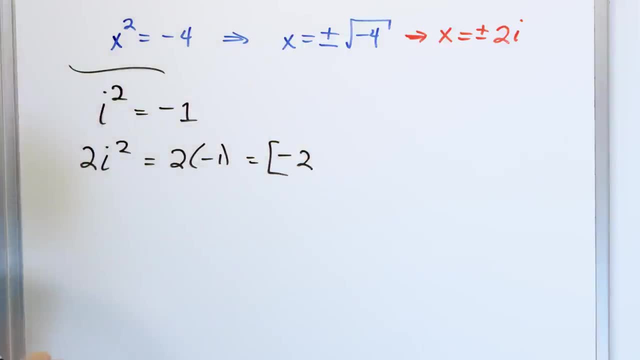 of the day. you don't get an imaginary number back, You get a real number. You get a real number back. Right, Same thing we got here. What if we have 3i wrapped up inside of a parentheses and that whole thing squared? Well, we treat it as we do anything. You pretend this is. 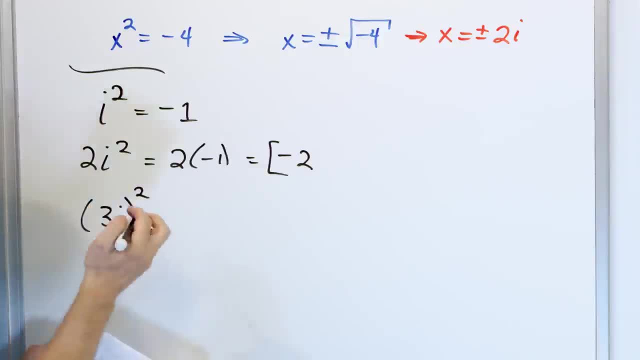 kind of like a variable. The exponent will apply to the 3 and to the i separately, So you'll have 3 squared times i squared. Same rules of algebra apply to complex numbers, to imaginary numbers. 3 squared is 9.. And you're still going to have this i squared. 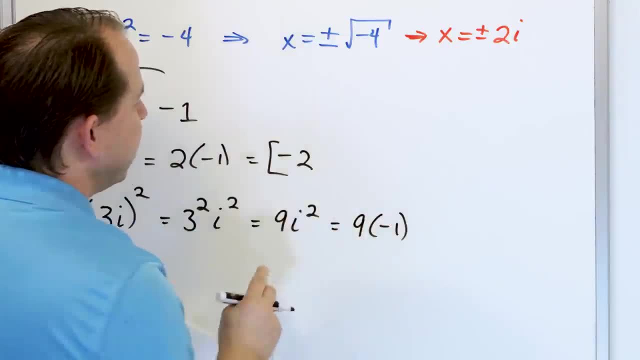 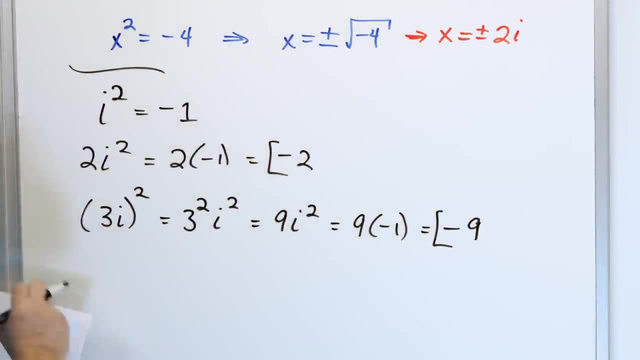 But any time you see an i squared, you substitute negative 1.. Any time you see i squared, you put negative 1 there, So it's negative 9.. This is the final answer. So when we have 3i quantity squared, we get a real number back which is negative 9.. 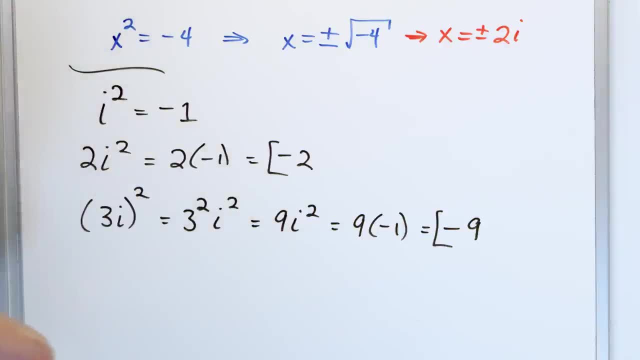 Now it turns out that these imaginary numbers, if you have them in a fraction, they can cancel, just like variables can cancel. So, for instance, 4 times, i squared in the numerator with i on the bottom Right. So I'm going to rewrite it just so I don't clutter up my problem statement. 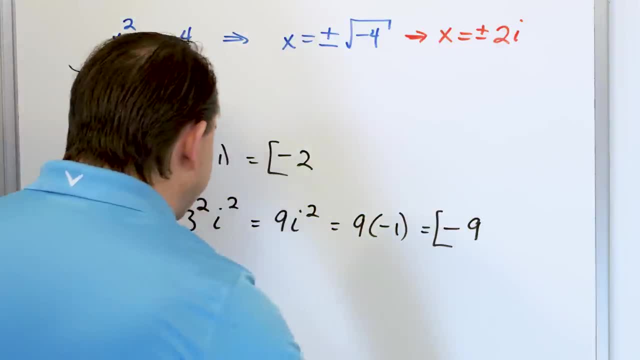 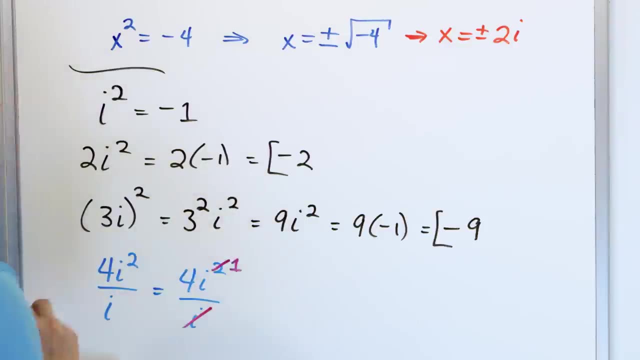 So this is 4i squared over i. So if these were variables, if this was like 4x squared over x, what you would do is you would say: well, I'm going to cancel this one And I'm going to cancel with this one, I'm going to leave an exponent of 1 left behind. Basically, 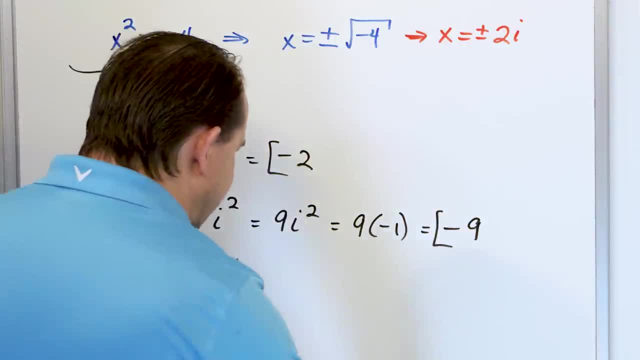 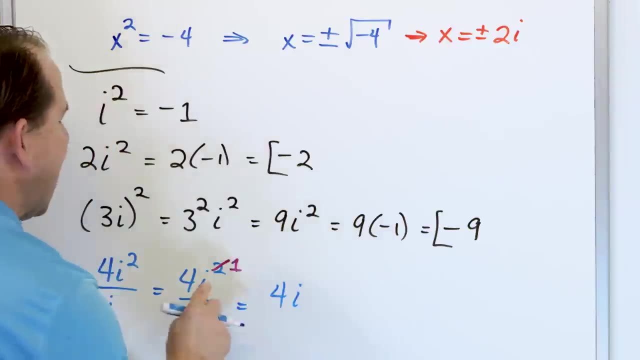 I'm dividing away one of them, And the same thing is true of imaginary numbers. So I had an imaginary on the bottom and imaginary squared on the top. All I'm left with is the 4 and the i on the top, To the first power. it's basically gone, divided away in the bottom. 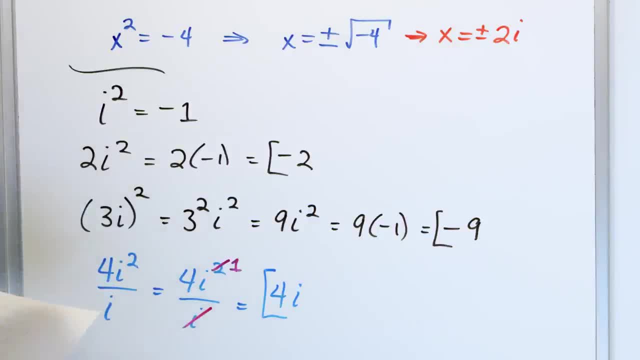 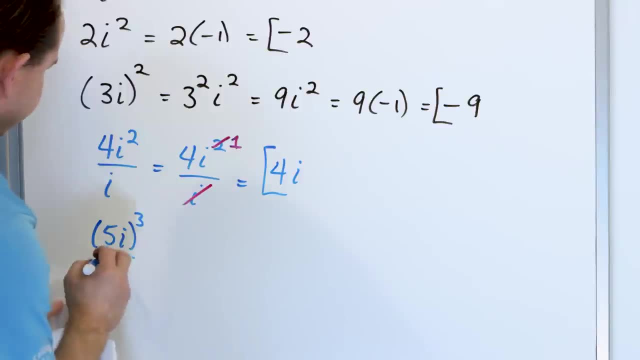 So I get an answer of 4 times i. OK, What if I have something more complicated? What about 5 times i? I have a 3-quantity cube, But on the bottom I also have an i. How do I handle that? Well, 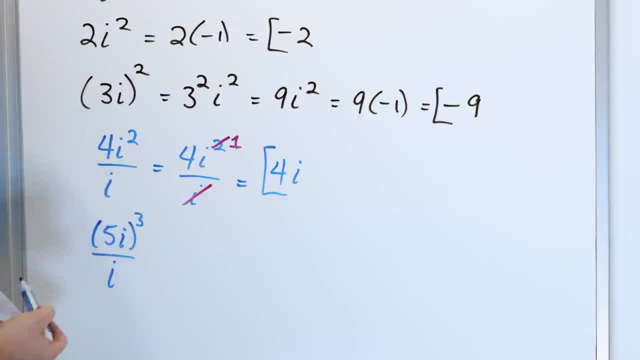 I still have this. numerator 3 is going to apply to the 5 as an exponent. It's also going to go in and apply to this. i Right, So you have 5 cubed times i cubed, And on the bottom, 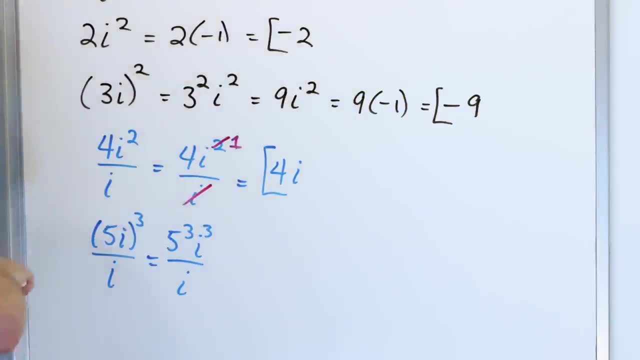 you still have this, i Right, But notice that I have the same variable, Just like it's not a variable- It's an imaginary number- But you can treat it as a variable. That could cancel with this, leaving me 2 behind. 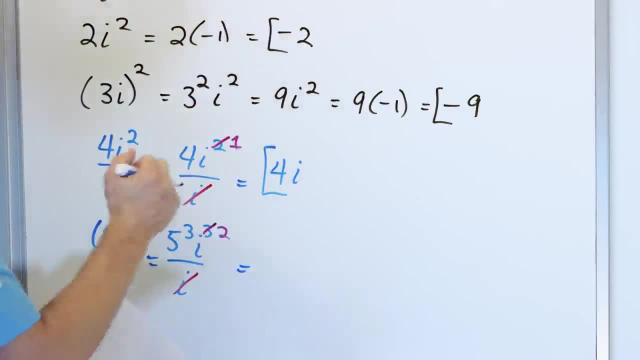 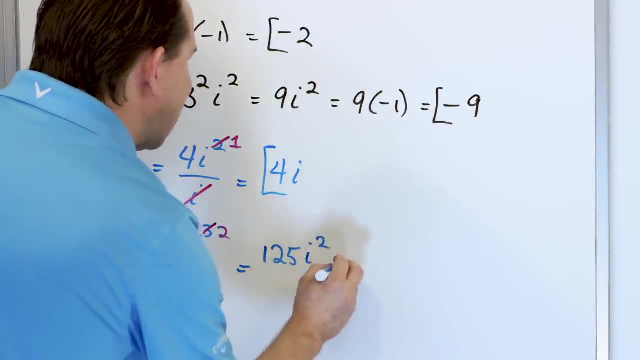 So what I have left with is 5 cubed 5 times 5 times 5 is going to be 125.. But what's left over is i squared. But we now know that i squared is very easy to remember Any time. 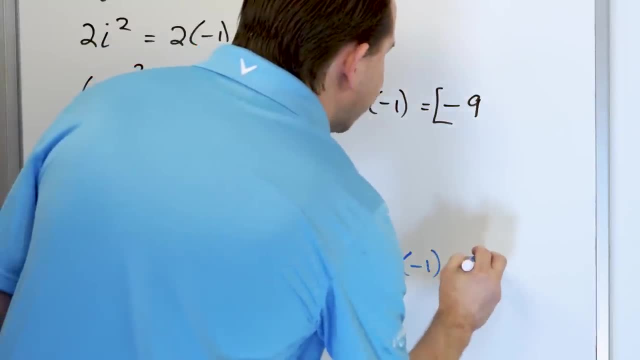 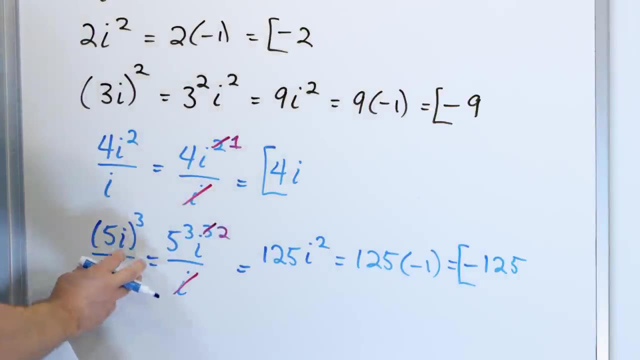 you see it, you just replace it with a negative 1.. So what you have is negative 125.. So this whole expression, which looks very complicated, with imaginary numbers everywhere, actually is not imaginary in the end. This is one of the things I've been trying to harp on to. 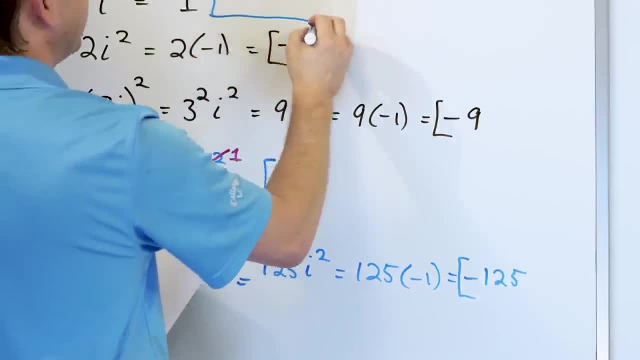 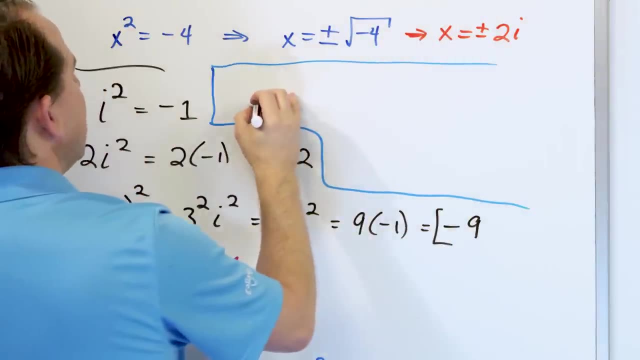 tell you. So when you're working with imaginary numbers, you'll get real numbers as your answers. The last one I'm going to do for you is a really interesting one. What if you have i cubed? Some students will look at that and say: I have no idea. You didn't tell me what i cubed. 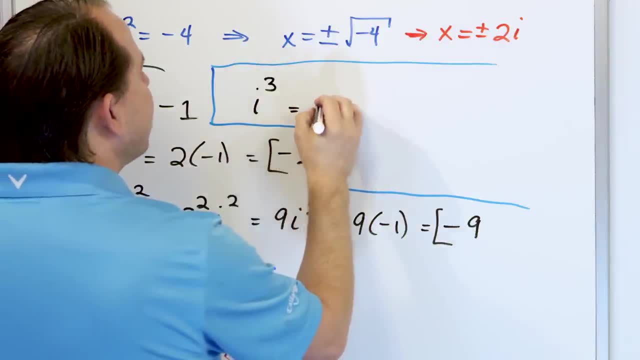 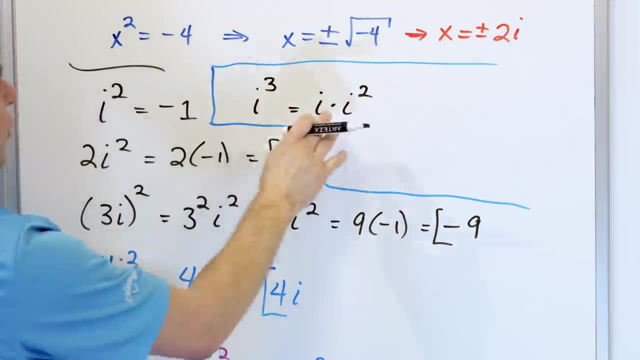 was equal to. Until you remember that i cubed can be written as i times i squared. Why? Because you can treat it as a variable. I can add these exponents, So of course it's equal to this, And I know that this i squared is negative 1. So really it's i times negative. 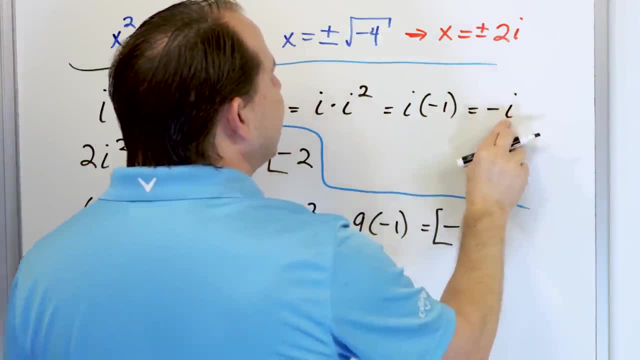 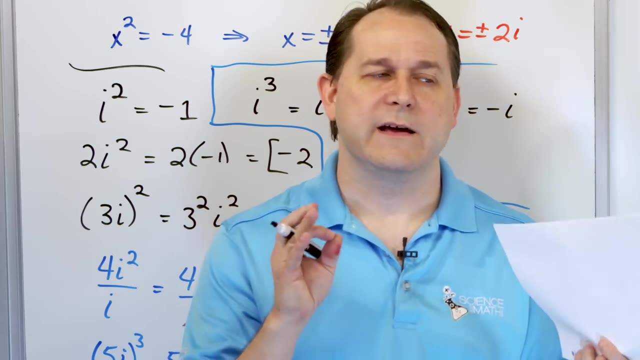 1, which means it's going to be negative. i So the imaginary number. i can be positive, It can be negative, It can have fractions involved, decimals involved. That's all fine. It's just a placeholder for the square root of negative 1.. And any time I see an, i squared. 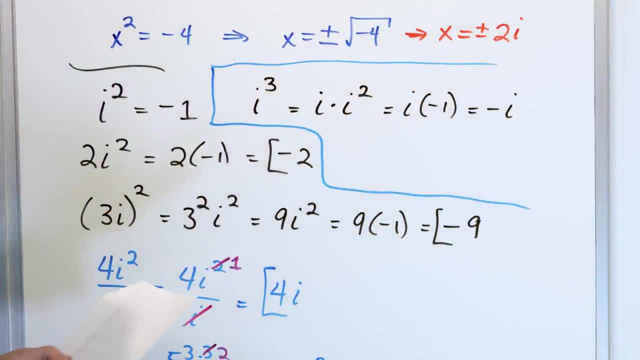 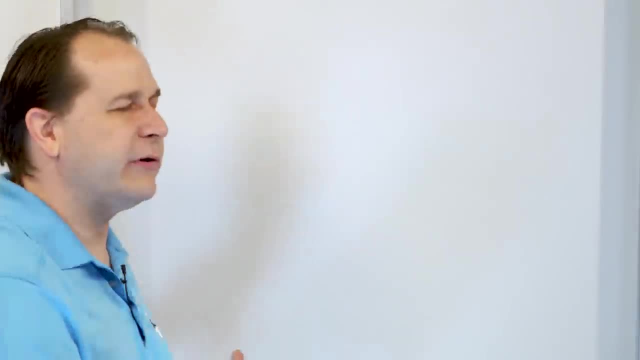 anywhere, I have to replace it with the real number, which is negative 1.. Now I've talked at great length, or at least in the introduction, to try to give you some motivation why imaginary numbers are so useful. What usually happens is you study imaginary. 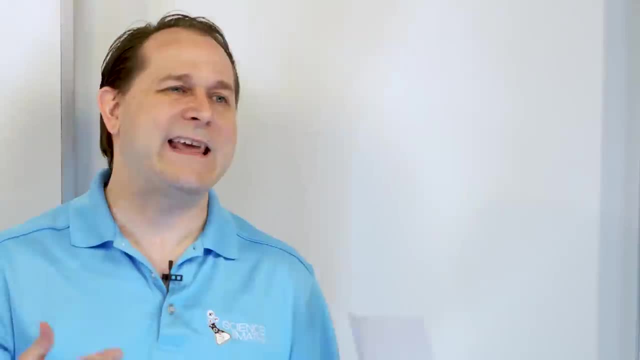 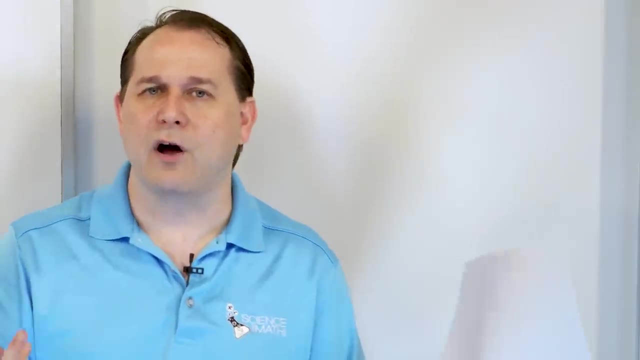 numbers in algebra And then in pre-calculus you do more with it, And then in calculus you do even more with it. And then, when you get in really advanced math beyond calculus, you take advanced math classes where we solve special equations, It doesn't matter what. 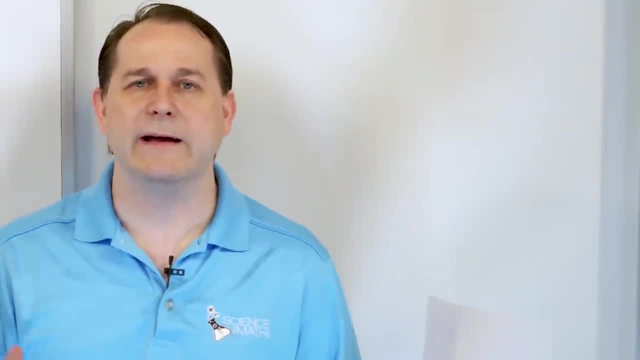 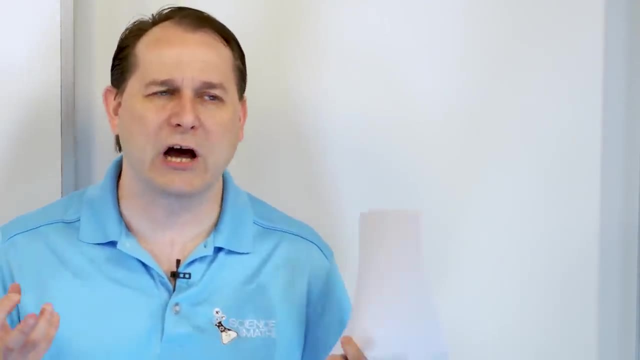 they're called? They're called differential equations, but that's the name of them. But anyway, they're equations And you deal with imaginary numbers every day And then finally, at the end, you understand why they're so useful and how common they are and how real. 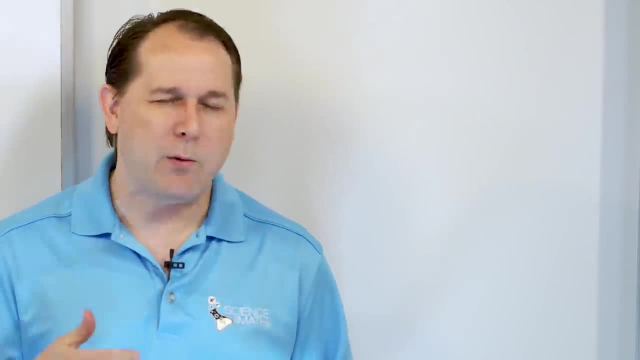 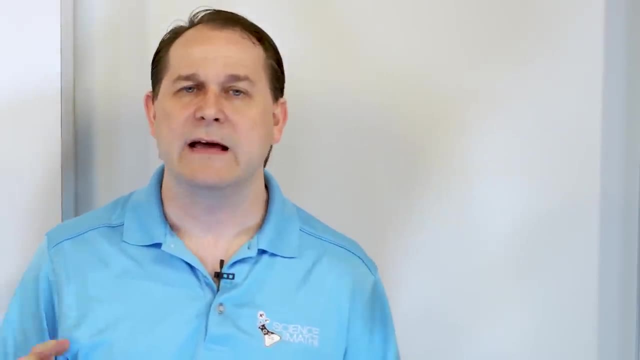 that they are in the solutions of our mathematics. But I want to short circuit that because I don't want you to wait. I want you to wait six years to figure out, or seven or eight years to figure out, why they're useful. I'm going to give you a quick 10 minutes or five minutes explaining that. 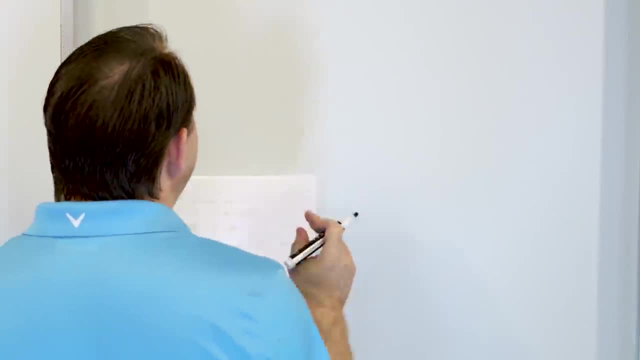 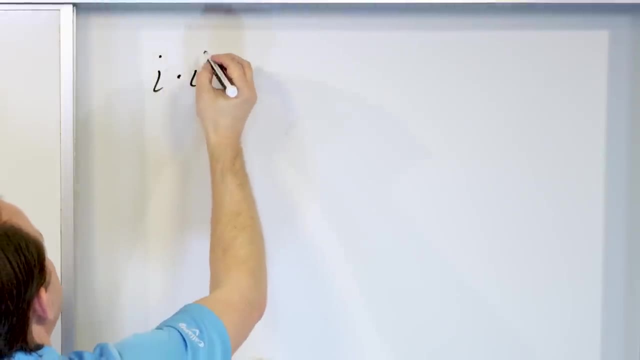 to you. So I've talked about in general the idea that I can have an imaginary number Like I have i strawberries, And I can have another imaginary number in my other hand, another i strawberries. So individually this is an imaginary number And this is also separately. 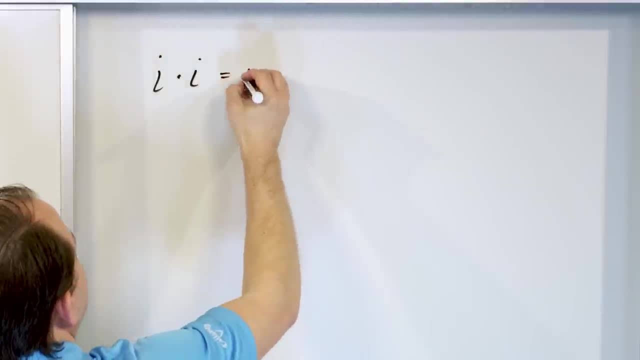 an imaginary number, But when I multiply them together, they form i squared, which I know is equal to negative 1.. So this is one of the main reasons why I'm going to talk about this, Because it's a real number. And this is one of the main reasons why they're so useful, Because separately they're not. 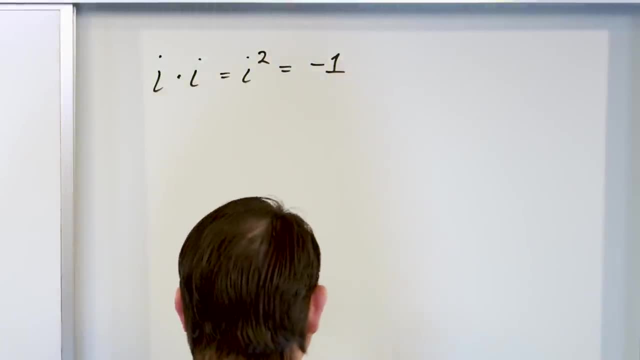 real numbers, But when I combine them together, they can give me a real number back, which is a tangible thing. This is something I can touch in the real world. I mean, yeah, it's negative, But it's still a number that exists in our everyday life So we can get as a 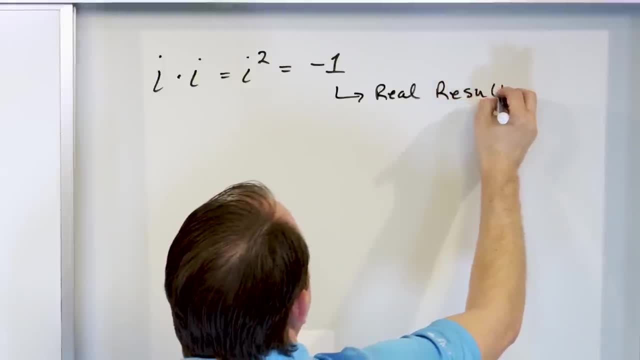 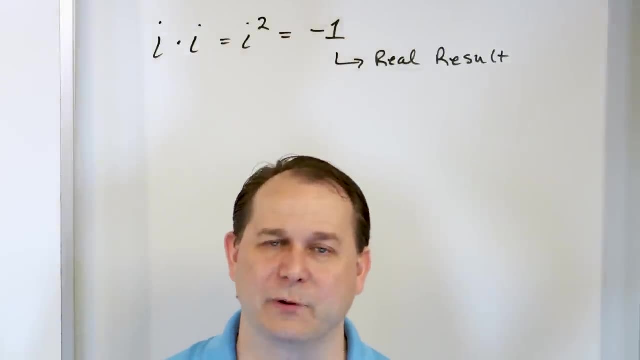 result, a real result. Now, this isn't too exciting. the i times i and all that. It's not too exciting. But there's one example I'm going to give you that's way beyond the scope of an algebra class, But I want to give it to you because it is so powerful. 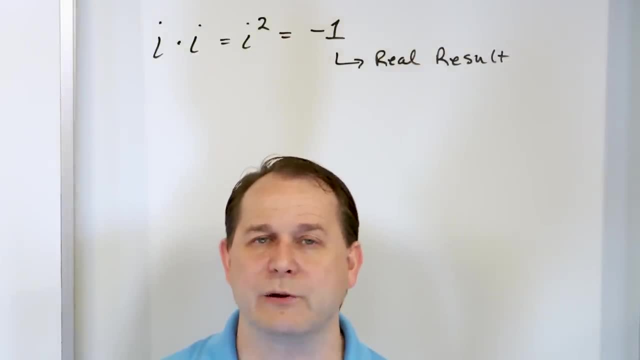 So powerful for you to understand how common imaginary numbers are in real world problems, I want to give it to you. I don't want you to wait until your second year of college to see it. All right, I want to introduce something to you that we're going to get to later in this. 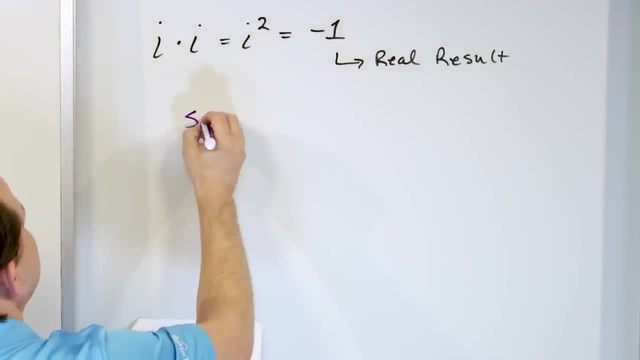 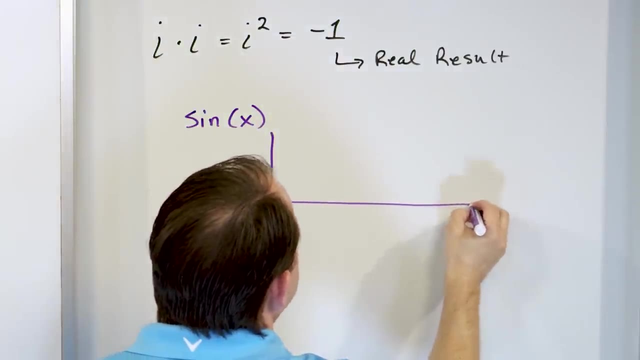 math class. in this algebra class, I want to talk to you about something called the sign of some number, right? So the sign. We're going to get to this in algebra later on in our set of lectures. I'm going to explain this to you in a future lesson, So this is not something crazy that you're. 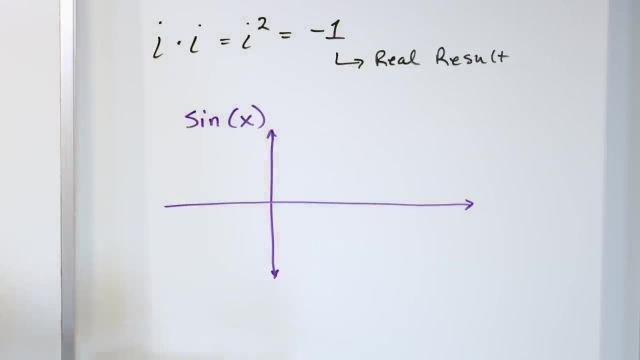 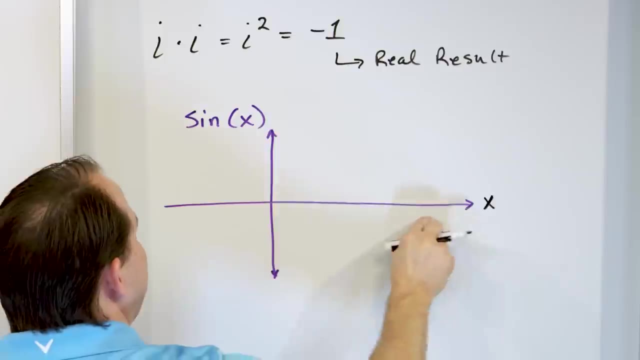 never, ever going to see. This is something quite common that you learn. So the sign is a special function. It's a very special function. Sine of x: This is the x-axis and this is the sine of x. It's very special. 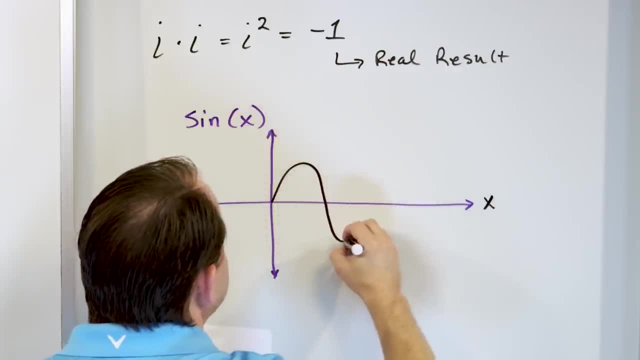 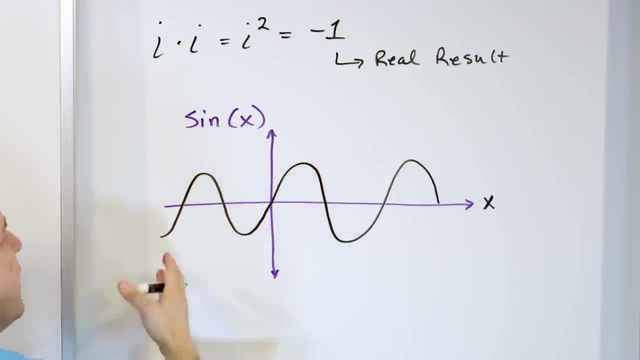 because it has this wavy shape to it. So it goes like up and then it goes down, and it goes up and then it goes down, And on the other side it continues the other direction. It goes down and up and down and so on. 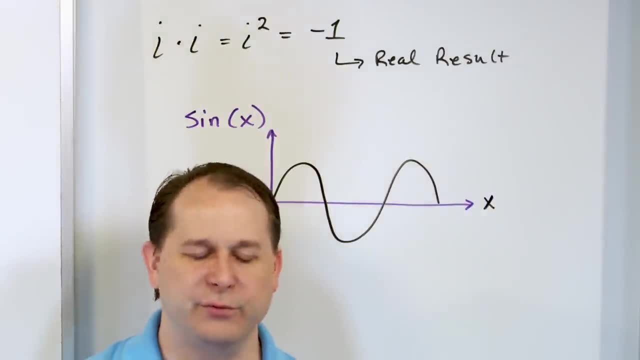 So you can see, it's this general wave shape, right, that you recognize. Why is this important to study this thing called a sign? Why is it so important to study something that has a wavy shape? Well, I'll try to explain it to you. You know light, we'll get into advanced. 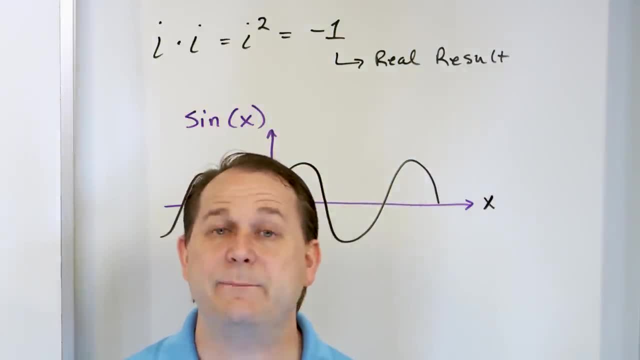 physics much, much later. but light. one theory of light is that it behaves like a wave. right, What kind of wave Here it is. This is the kind of wave that a light wave actually is. So later on in your education, when you write down what does a light wave look like, or what, 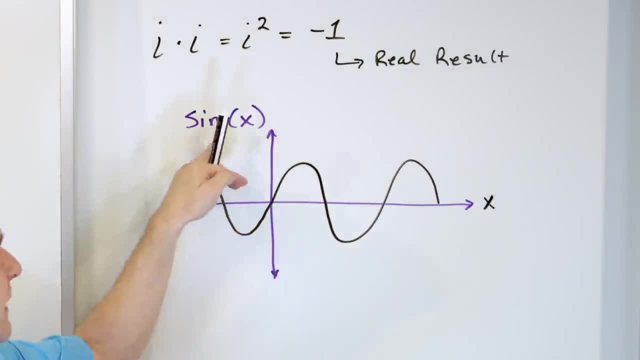 does a light wave behave like you're going to write down a sign, Write down its cousin, which is called the cosine. I'm not going to get into that because it's the same shape. A cosine is the same shape as a sign. It's a wavy shape, a very 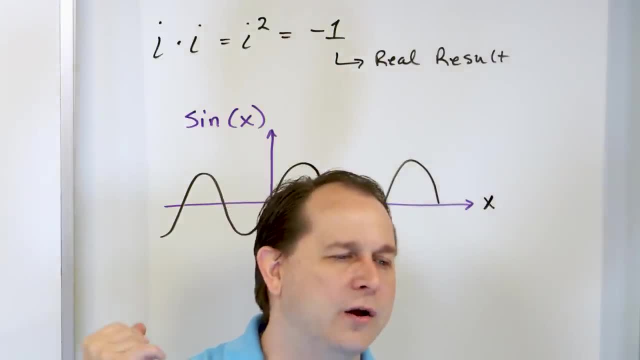 special shape that's extremely common in nature. All light waves are sine waves, right, which means X-rays, gamma rays, infrared visible light, the light that goes into your eyes, microwaves that you heat your food, radio waves, which your cell phone uses and your 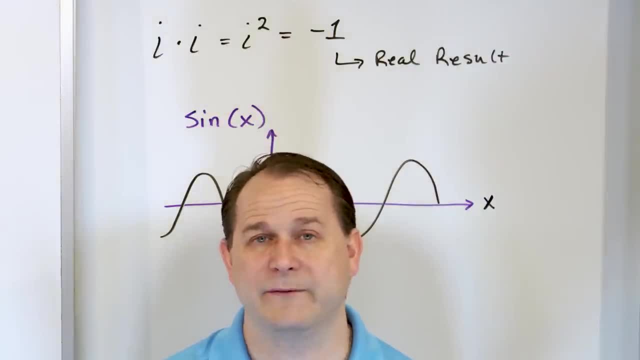 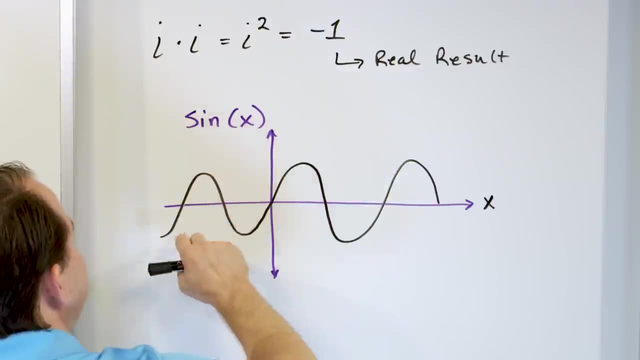 walkie-talkies to talk to people. All of those things are sine waves, right? I'm building it up for you because of the following thing: This sine wave is numbers that are plotted on the Y-axis here as a function of this. It's just like any other function. 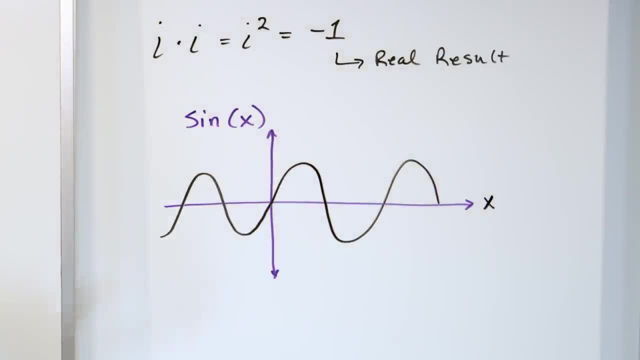 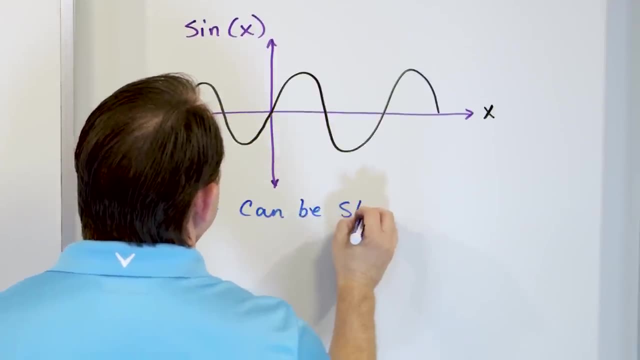 It just goes up and down, and up and down, and up and down. It can be proven in advanced math classes. It can be shown. I'm not going to show it here because it's way beyond the scope of this, but it can be shown that this thing 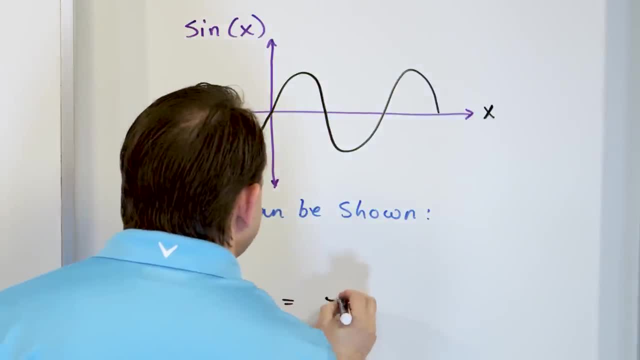 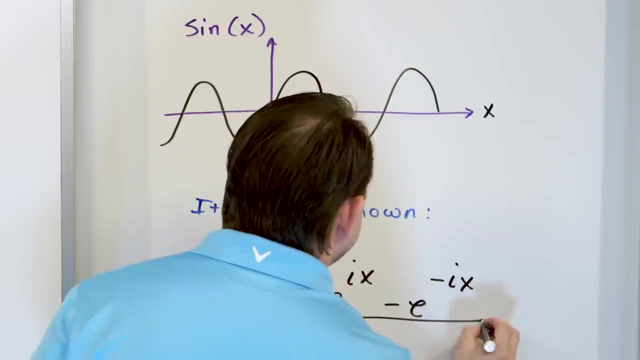 is a sine wave just as we know it. So you take the negative, negative, this theta that can be squared, and you divide this and then again looked like this: you divide it down and you multiply it and you get a sine. 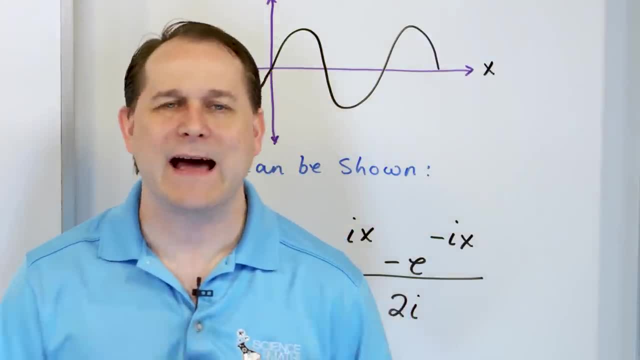 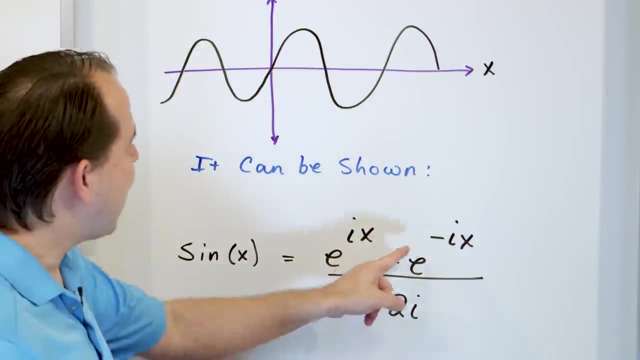 To redeem you of the sin setting that was coming from. the sine can be written like this: Equals e to the i times X minus e to the negative, i times x all divided by two times i. This is incredibly important for later mathematics. It's not important for algebra, I don't care. if you remember. this. I don't care if you toss it in there in the trash can and just forget about it. That's fine. When I'm trying to show you, though, is notice what you have here. E is just a number. We're going to talk about E as the sum of all of the sides of your rival. 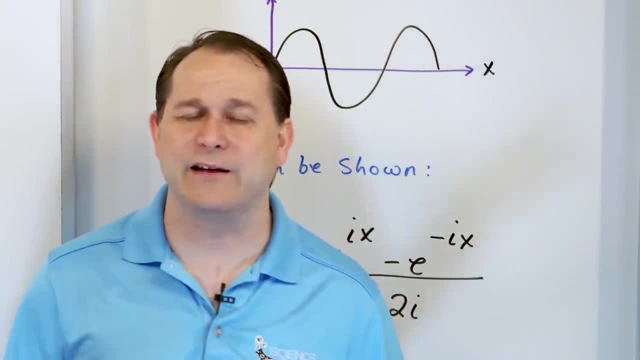 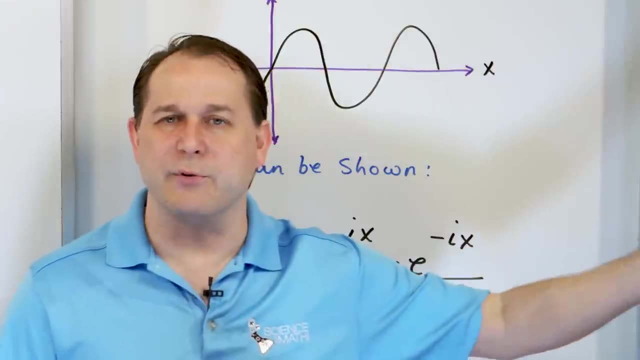 actually not too much longer from now. That's a number like pi. it's an irrational number that's very common in nature. It's not equal to pi. it's equal to about 2.7 and some infinite number of decimal places after that. 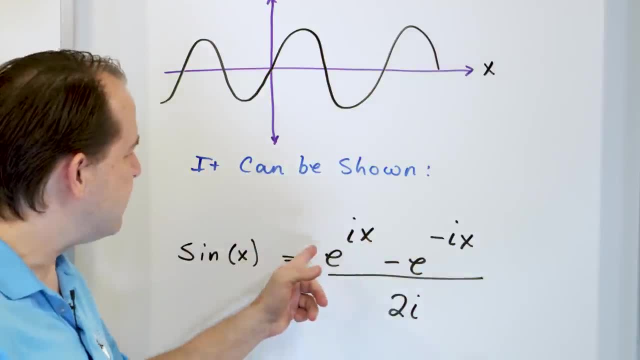 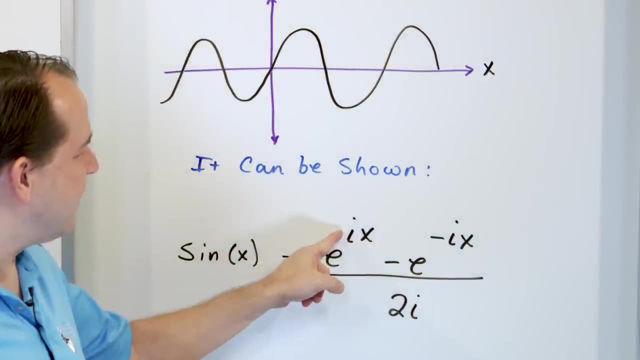 but it's just a number. So this E is not a variable, it's a number, It's some number to the, to the what, To the power of IX, so to an imaginary power. So this is an imaginary power. This is an imaginary power too. 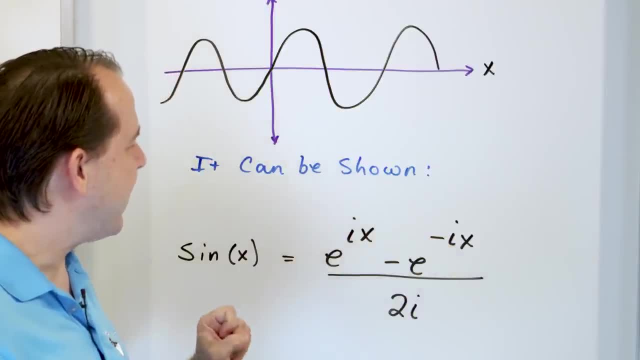 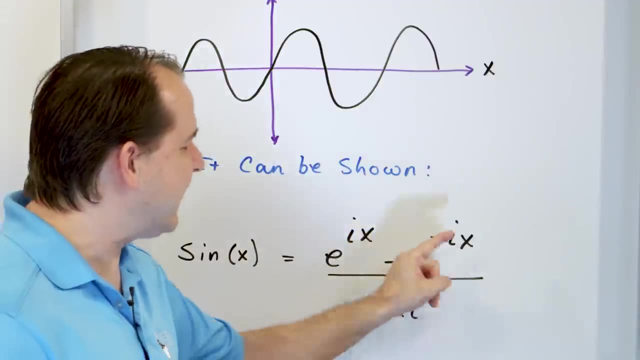 but it just has a negative sign in front. So if I take this guy to this imaginary power and then I subtract E raised to the exact same thing, but to the negative of a copy of itself, but to the negative imaginary power, if I take the answer to that and I divide by two times, I 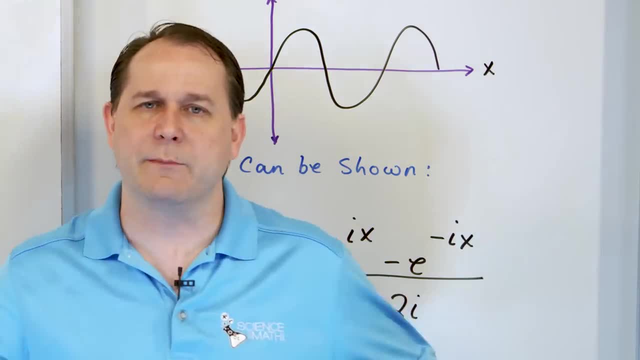 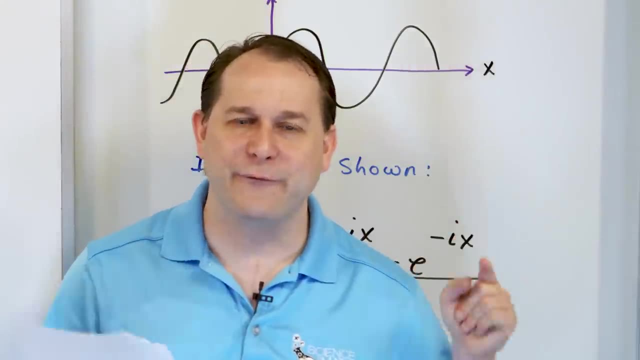 which is another imaginary number. See, I'm putting these imaginary numbers in a pot and I'm stirring them around in this function. What you get out is not an imaginary function, It's a real number. So imaginary numbers go in here. imaginary numbers go in here. 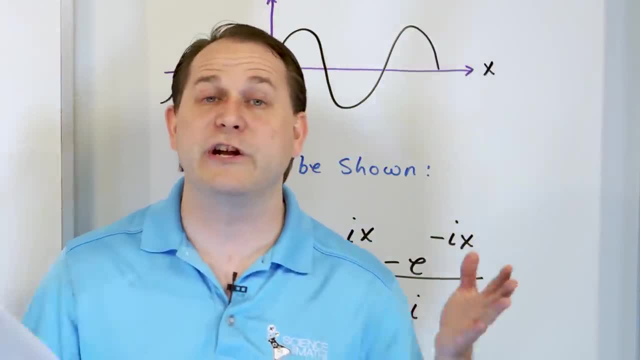 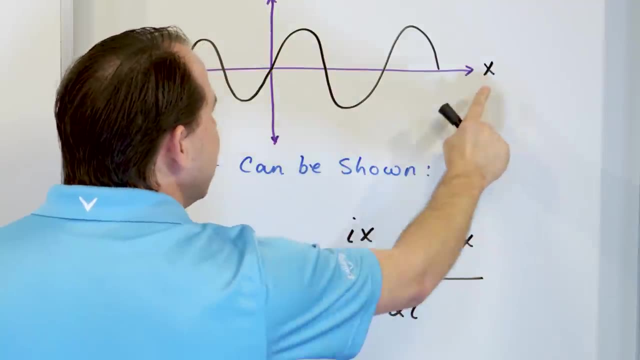 imaginary numbers go in there. What you get out is not an imaginary number. You get a real number back And that real number is a plot. I can plot this real number as a function of whatever I stick in here. See, this is X. 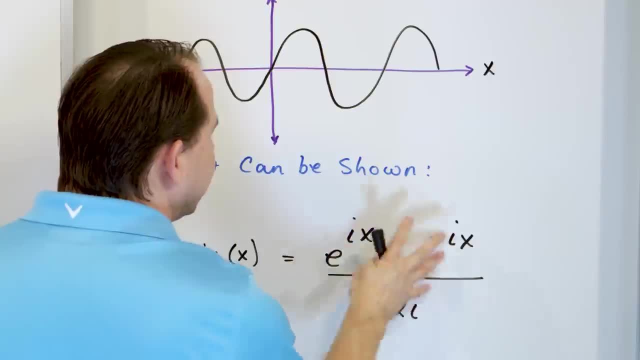 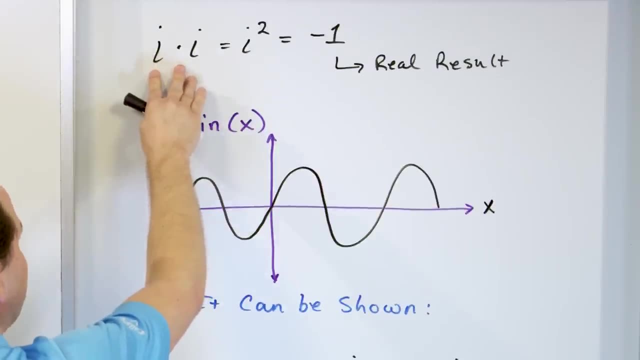 It goes in here. Well, you would put it in here, put it in here, calculate it all, get the thing, but you don't get an imaginary number back. Why? It's for the same basic reason that we don't get an imaginary number back here. 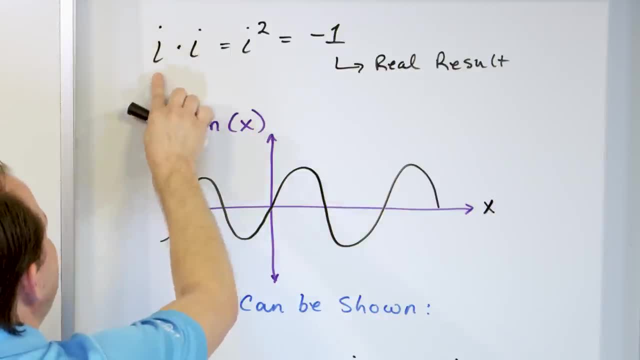 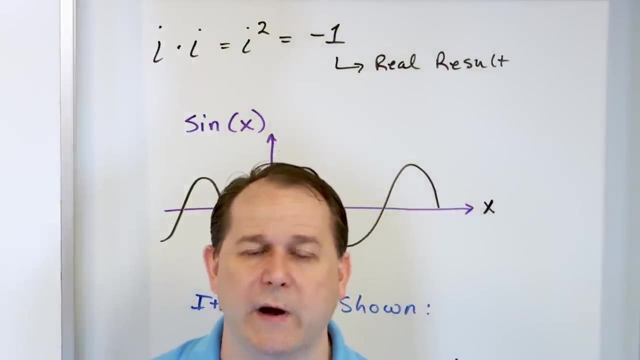 I mean, it's beyond the scope. I don't want to prove it, but basically you can see how you can combine imaginary numbers and get real numbers back. Well, I'm combining imaginary numbers in a much more complicated way and you're just going to have to take my word for it. 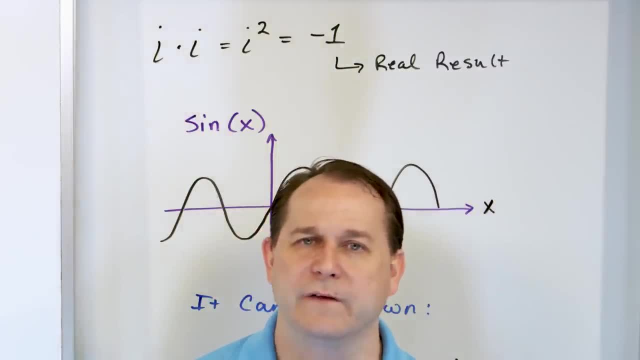 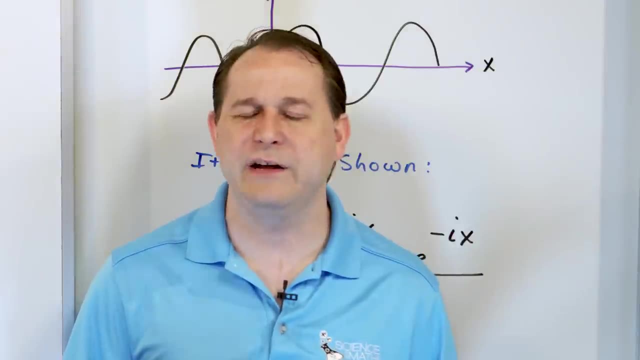 that you don't get an imaginary number back. So why am I doing all of this? Because when I first learned what an imaginary number was, I thought they were useless. I thought I would just circle some answers for the teacher and be done. 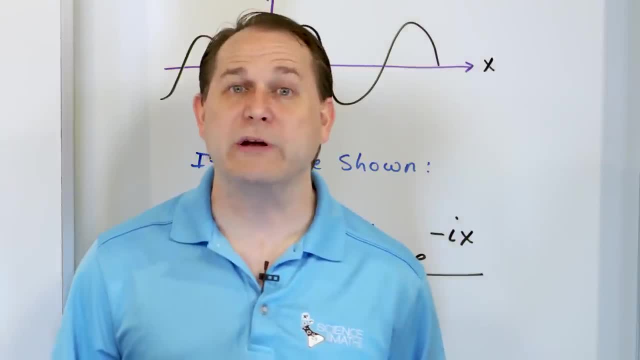 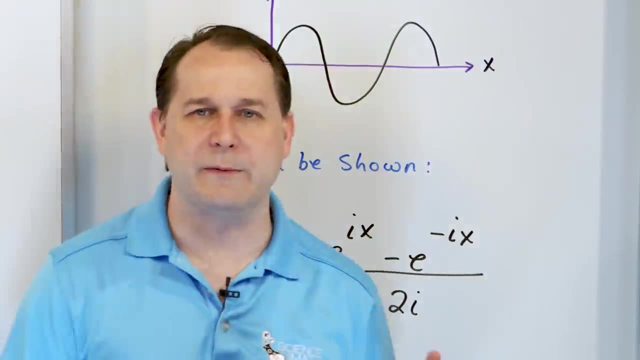 But it turns out that almost every equation that we solve in real life looks like some kind of wave, And if it looks like some kind of wave, that's a sine wave. then it can be written as imaginary numbers, And so a lot of times you'll get an equation. 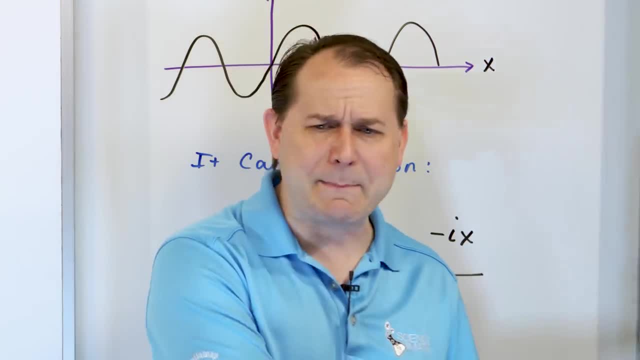 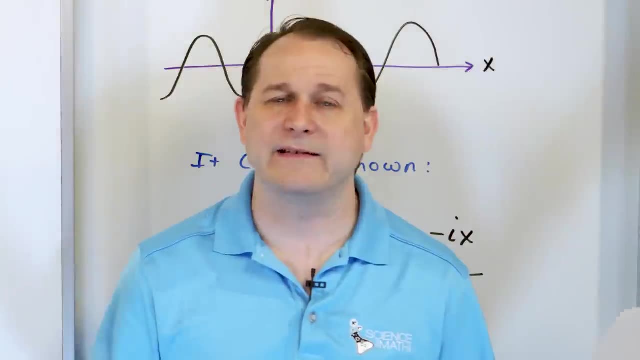 you'll solve it. you'll get some imaginary numbers in the answer and you might have to take that and multiply it by another equation which has some other imaginary numbers. When they get all mixed together, sometimes what pops out is not an imaginary number at all. 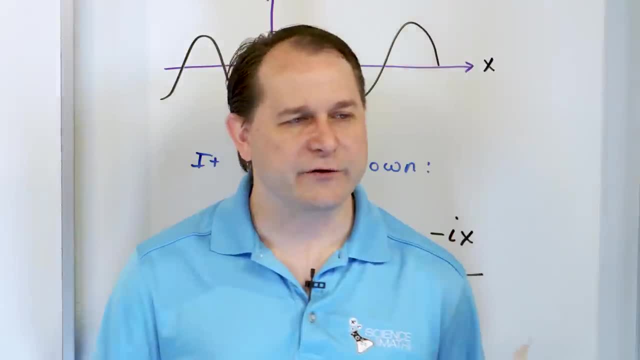 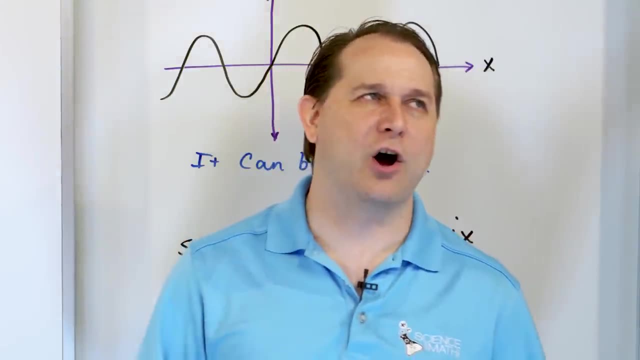 It's a real number And that's why it's so useful. Another example would be quantum mechanics way future physics, you'll study that long time from now: All the solutions of quantum mechanics. I shouldn't say all, but most of the solutions of quantum mechanics. 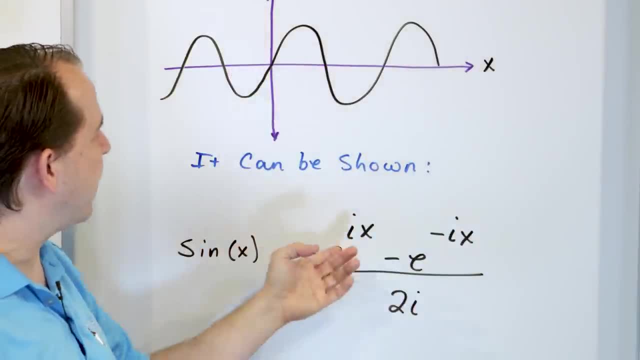 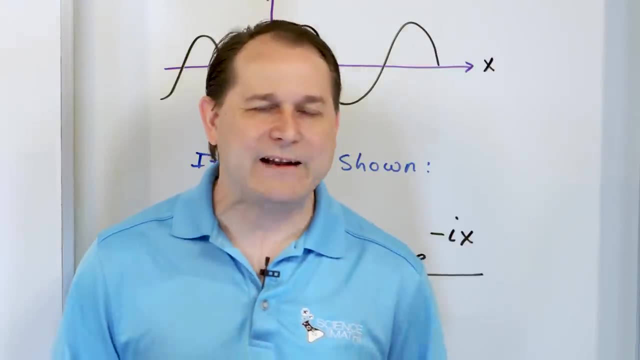 are all waves, They all involve these signs or they involve these exponents, with I in there, And you mix them around and oftentimes you get real numbers back right. That is why imaginary numbers are so useful. We don't know how to take the square root of negative one. 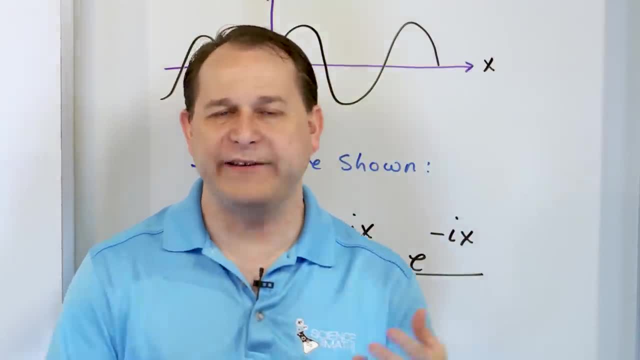 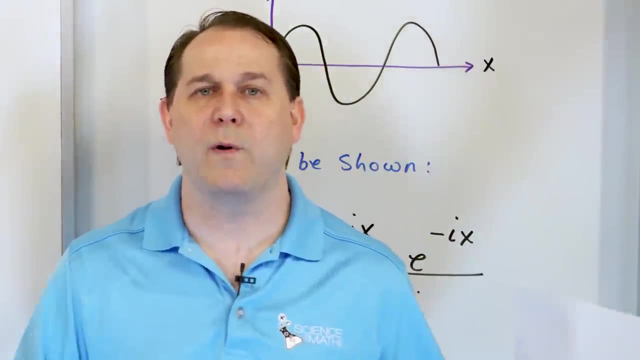 with a real answer, but as a placeholder we say: we just say it's equal to I. We keep it as a placeholder and we start combining it with other things And then oftentimes, pop poof, the imaginary numbers go away.